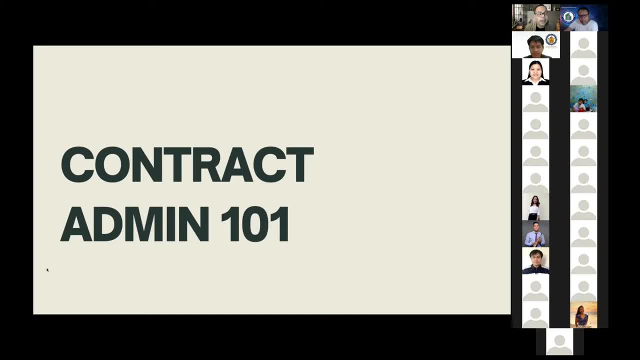 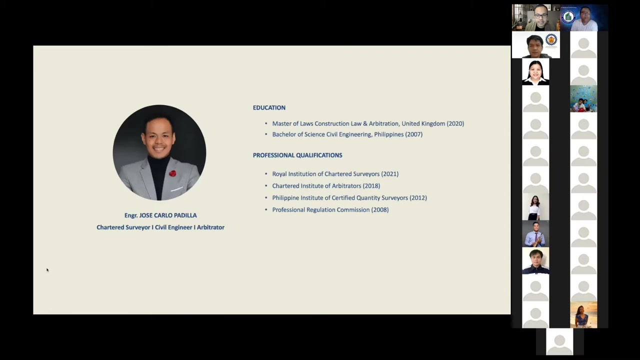 attendees are expected to have gained an awareness insofar as the clauses which concerns variations, extensions of time and limited damages. Again, I would like to thank Joe, Phil and Jet for having me today And before we begin, although it has been said earlier, I would allow me to introduce myself Again. I am Jose. 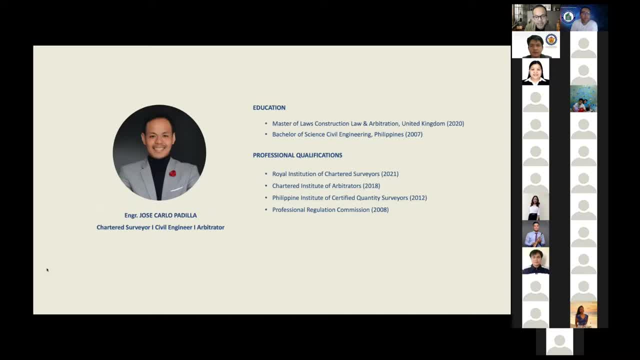 Carlo Padilla. I'm coming to you all the way from Singapore And I bring with me more than 10 years of experience in the construction industry, with involvement in projects that ranges from development of residential and commercial and civil engineering projects. I have a bachelor's degree in civil engineering from the Philippines and Master of Laws in Construction Law and Arbitration from the United Kingdom. I am a member of several professional organizations, such as the Royal Institution of Chartered. 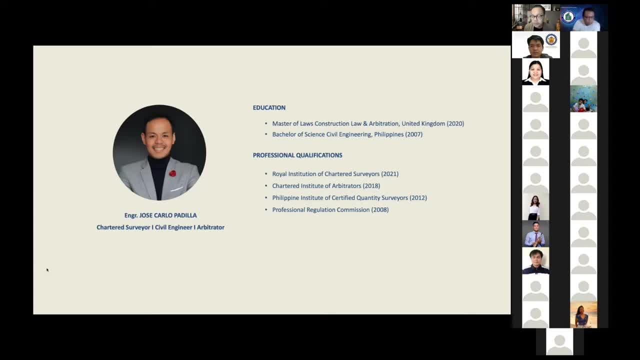 Surveillance and Chartered Institute of Arbitrators. Both of them are in the United Kingdom And in the Philippines. I am a member of the Philippine Institute of Certified Quantity Surveyors and a registered professional civil engineer under the Professional Regulation Commission, So my areas of expertise are procurement of construction works, contract administration and management, construction law and dispute resolution, among others. 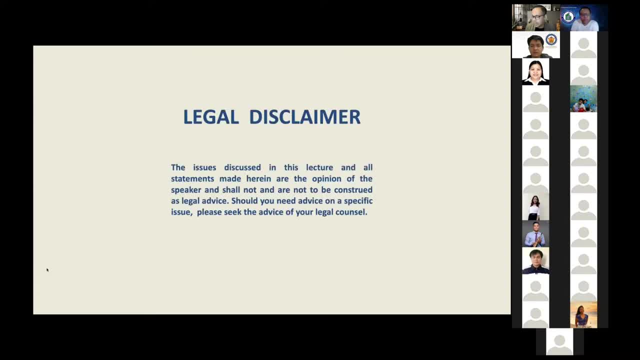 Thank you, Thank you, Thank you. allow me to read to you my disclaimer. The issues discussed in this lecture and all statements made herein are the opinion of the speaker and shall not be, and must not be construed as legal advice. Should you need advice on a specific issue, please seek the advice of your legal 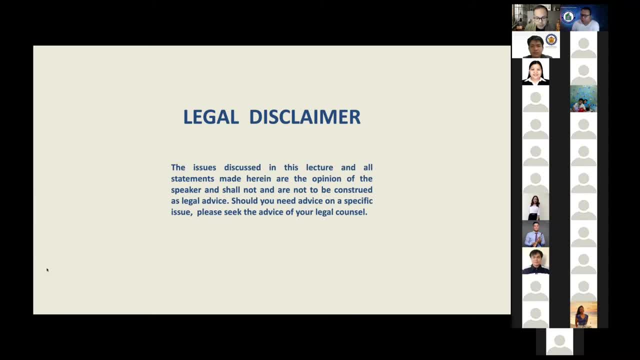 counsel. So at the end of the presentation there will be a question and answer part where you can ask your questions or, if you need clarifications on the issues that we will be discussing today. All questions or clarifications will be answered at the end of the presentation so as not to avoid. 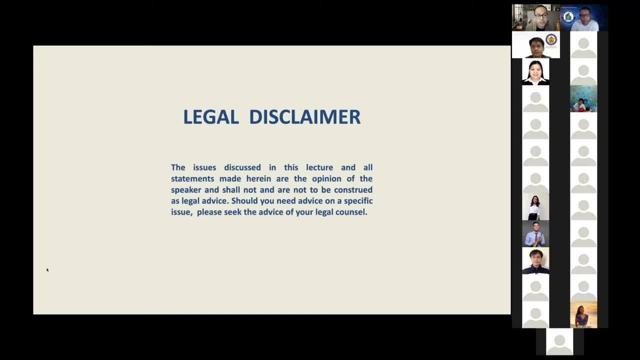 or so as to avoid disruption of the discussion for today. right, So we begin with the question: what is contract administration and why is it important? Contract administration is the management of a contract, in this case a construction contract, to ensure that the 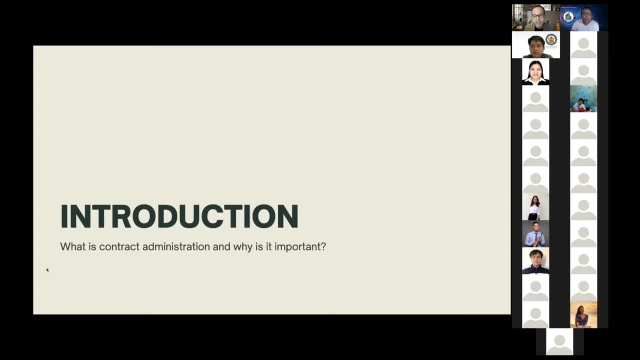 obligations of the parties are performed And their rights under the contract are preserved. A proper administration of the contract will lead to avoidance of disputes and, by extension, will lead to the timely completion of the project. Because of the broad scope of contract administration, I will be only covering 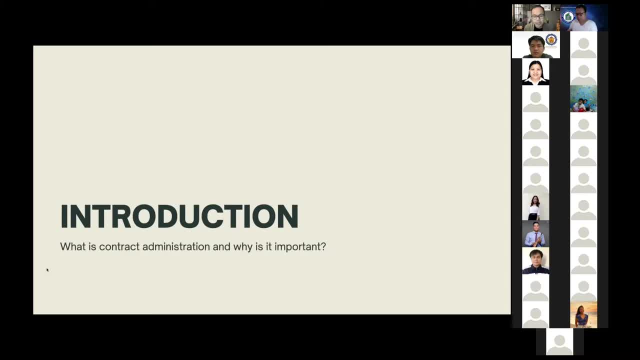 three topics for today, which are the most common sources of disputes. These are variations, a extension of time clauses and liquidated damages clauses. So before we begin, let's look at disputes around the globe and the common reasons why they arise. 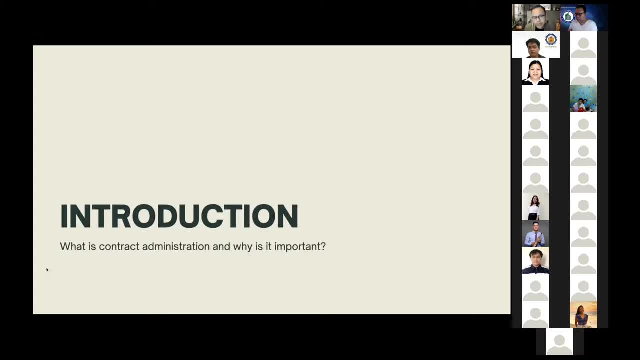 According to a study conducted by Arcadis in 2021, the amount of global disputes that is handled by them around the globe is amounting to 54.6 million US dollars, And among the most common areas of disputes or causes of disputes is the parties, meaning the client, the contractor or subcontractors. 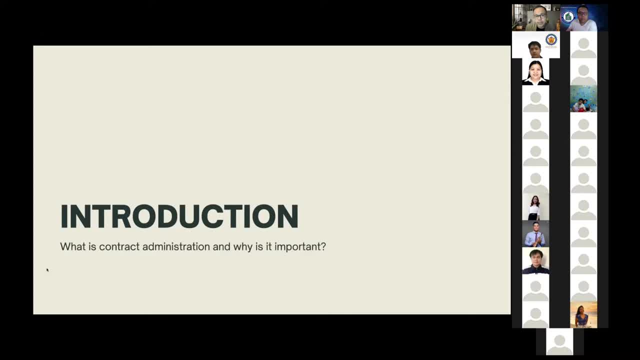 failure to understand and to comply. This emphasizes the need for a proper administration of the construction contract, Because if a contract is administered correctly, disputes can be ultimately avoided. So in this lecture, as I have said earlier, we will be discussing the three main focus. 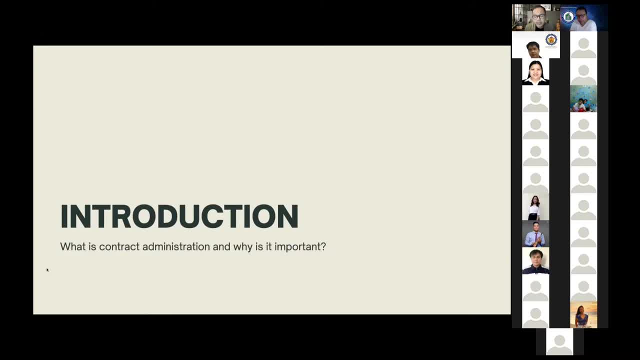 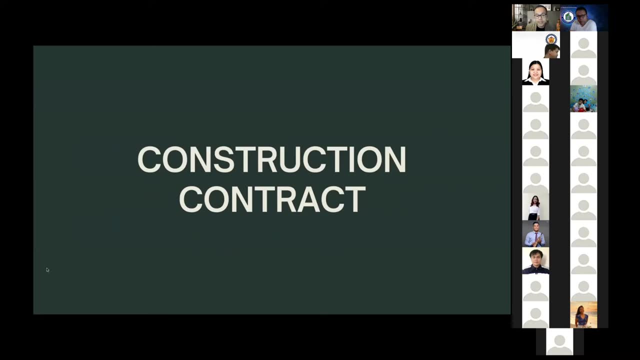 or the three main issues. that gives rise to the disputes. But first let us discuss what is a construction contract. So a construction contract can be defined in a number of ways. Generally, a construction contract is an agreement between the employer or the client and the contractor, where the 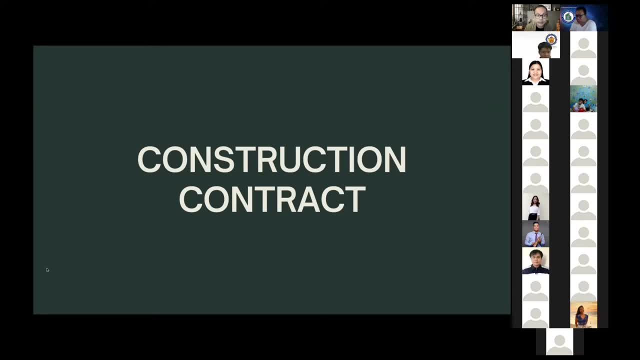 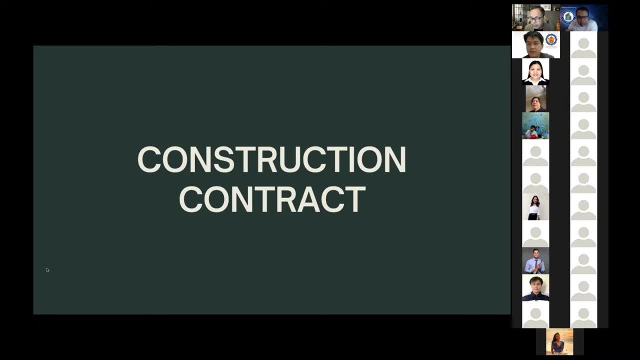 contract can be defined in a number of ways. Generally, a construction contract can be defined in a number of ways. Generally, a construction contract can be defined in a number of ways. Generally, a construction contract can be defined in a number of ways: mercy. 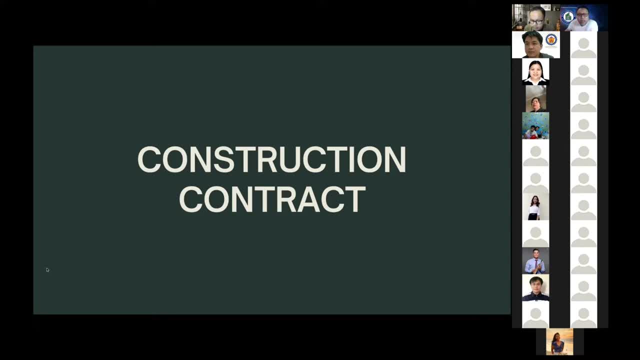 Jeremy Cor skies, Jerome terrified and word it coffee. We will have to put two speakers. Thank you, and I welcome everyone after us. The word has gone. Your name, Aye Aye, Aye Aye. 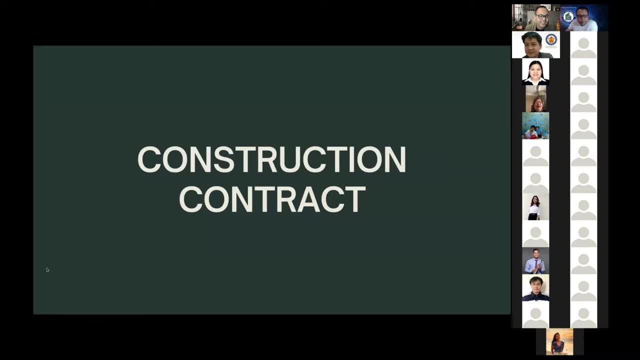 Aye, hello, mr engineer, carlo jose carlo padilla, for having accepting the challenge of the topic: contract administration 101. you know, and i'm happy to see uh 37, more or less 36 participants who give to this management. we have the just corporation, uh, just construction. 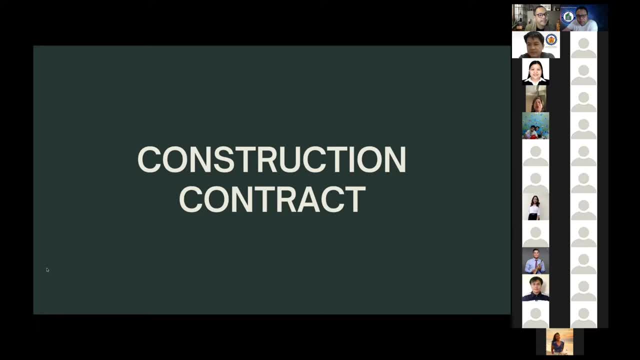 corporation and the vc graduate school who collaborated with this uh activity and i'm welcoming all the participants and i'm i'm sure that this will help those who wants to be a contractor someday or to to dwell in the construction business to take note of this uh topic: construction. 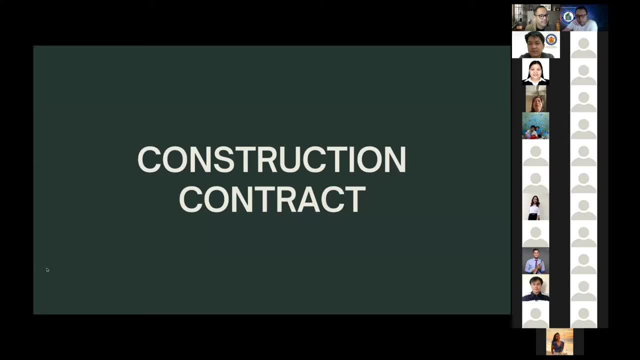 contract. so thank you, engineer, uh jose carlo padilla, and welcome to the participants and also to uh, dr joff hill hoxon, and to our extension coordinator, dr jet aquino. welcome and thank you, good afternoon. yeah, thank you, okay, jc. sorry. all right, so, uh, we um continue with the presentation, all right, so uh. 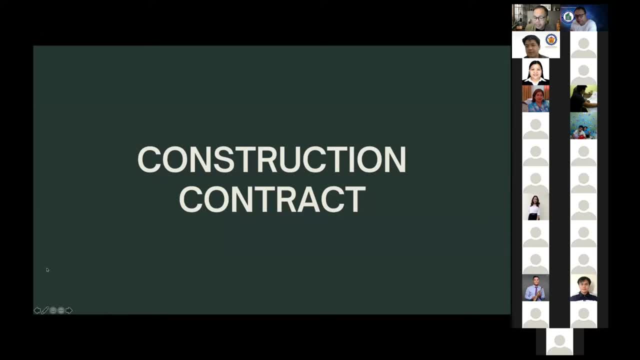 where am i all right? so, as i have said, uh, the article 1713 of the civil code of the philippines divide uh defines what a construction contract is. So the definition of the construction contract in the Philippines is guarded or defined in a legislative instrument such as the civil code. 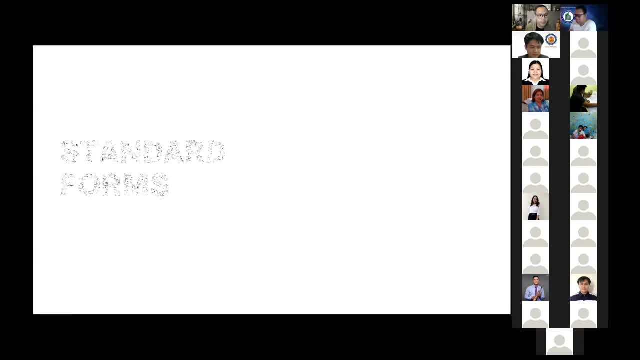 So now, we will now be proceeding with the standard forms of contract because, if you may not be aware, there are several standard forms of contract, because contracts can be difficult to draft and at least challenging to draft. So what the industry practitioners or the industry experts did is that they devised standard forms of contract. 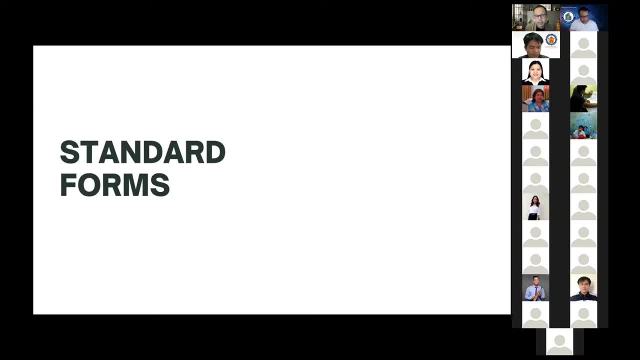 which are widely used And very popular in the construction industry. So standard forms of contracts, I have said earlier are templates or standardised agreements which supplies the legal basis and mechanisms and remedies which safeguards the contracting parties, Our rights and obligations concerning the construction works. 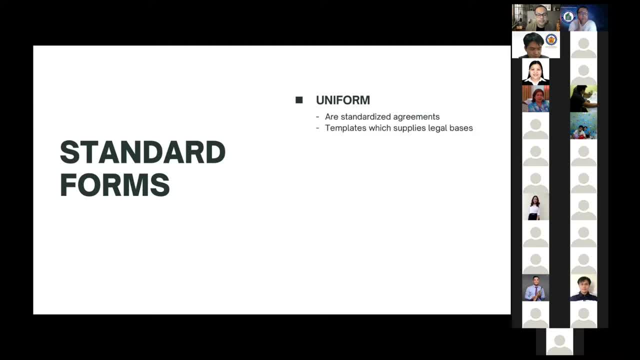 The standard forms of contracts are drafted by institutions with the support of the professionals and industry experts. It is a fair analysis of the design of the contract industry stakeholders. the standard forms of contract are prescriptive in so far as it provides guidelines on the operation of the contract which will assist in the contracting parties in the 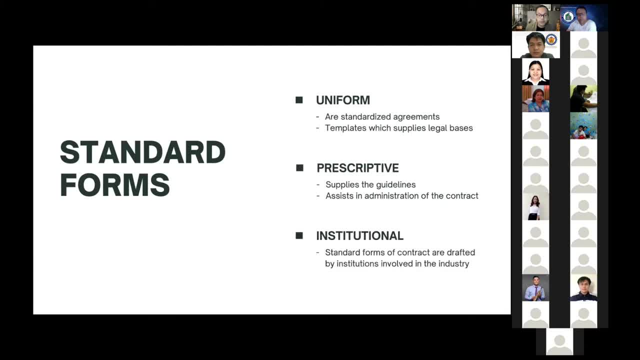 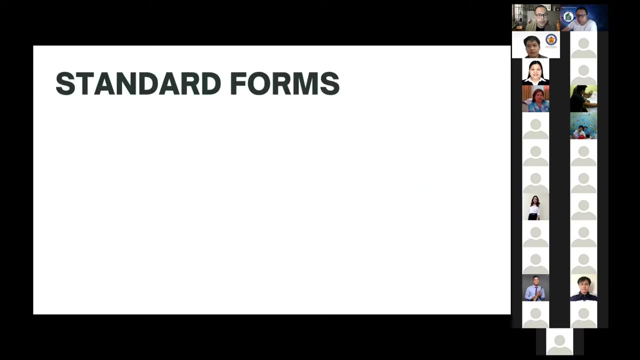 administration of their contract. and, finally, the standard forms of contract are published by institutions, which defines the standards in the industry. so in the next slides we will look at the standard forms of contracts available in the construction mark market and the institutions that publish them. so, uh, probably the arguably the most famous of the construction contracts. 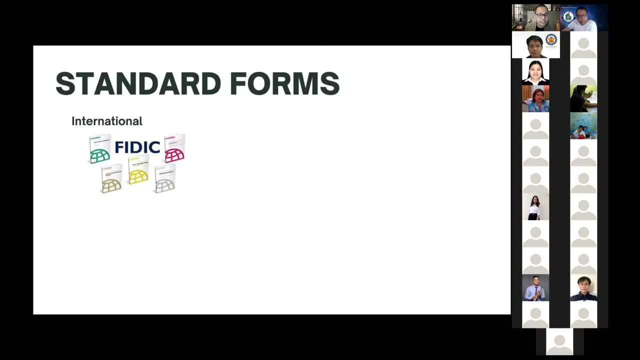 uh standard forms of contract is the phoenix suit of contract. so phoenix stands for federation international engineer or the federation of international consulting engineers. fiddick is an organization of 102 countries. it is known to be a contract written by the engineers for the engineers. fiddick form of contract is widely used around the world. 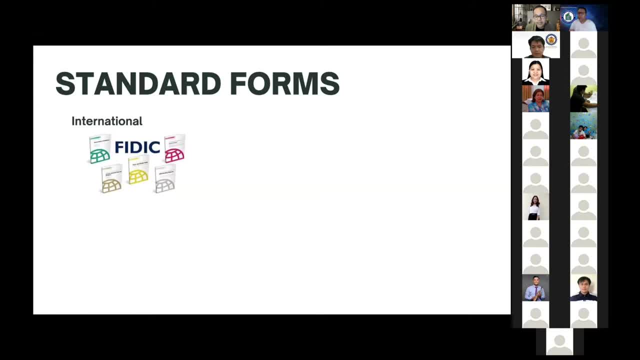 and in numerous jurisdictions, making it or making the interpretation of the clauses, supported by a wealth of case laws and jurisprudence. fiddick contracts has currently five iterations, which suits traditional contracts. so the first is the jcp. the most popular standard for this contract is the jct. 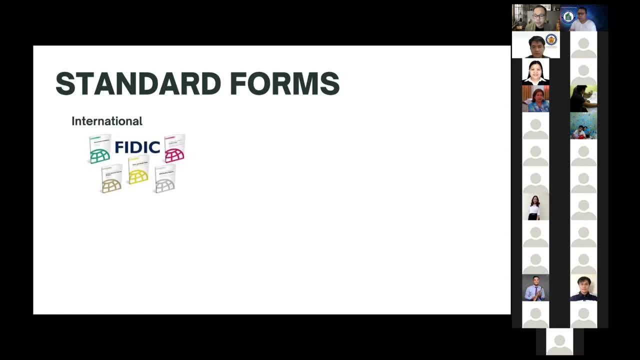 which is the joint contract contract, and the synth suit of contract is the, the joint contract of contract, which is one of the most popular standard contract forms of contract and it's designed for the red book, uh design and build procurement. for yellow book, uh design, build, operate, epc or what we call turnkey contracts, and that will be for silver book and a short form of. 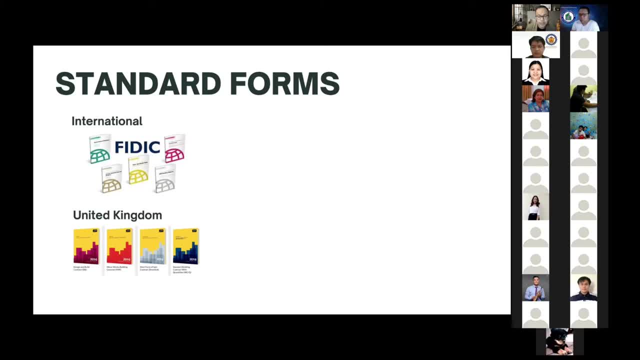 the most popular standard form of contract used in the United Kingdom. In fact, it accounts for 70% of the standard forms used in the UK. So the GCT consists of seven member organizations, which represents the sectors in the industry. Among these member organizations is the Royal. 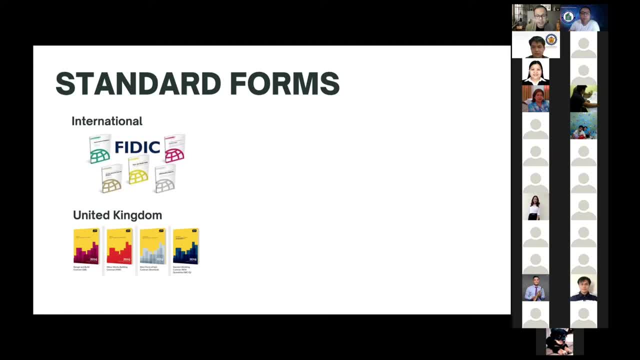 Institution of Chartered Surveyors and the Chartered Institution of Building. The current edition of GCT is 2016 and it has four main variants for contracts procured through: traditional procurement, the design and build route management contracting and integrated team partner. And finally, in the Philippines, we have what we call the uniform. 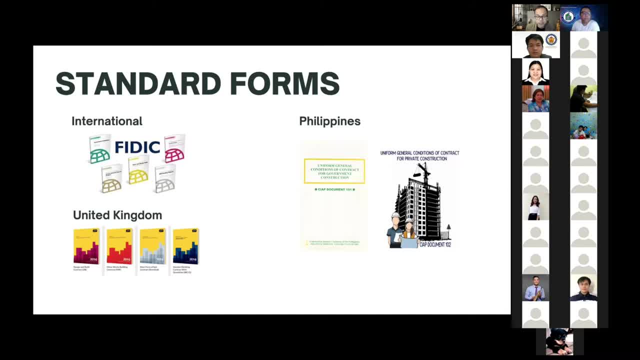 general conditions of contract for government construction and for private construction, both issued by the CIAP or the construction industry authority. So now, having discussed the standard forms of contract, we are now ready to look at the provisions usually contained in the standard forms of contract. So first issue that we will be 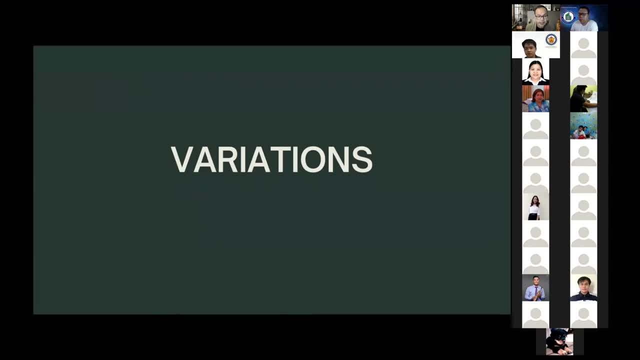 discussing today is variations, So variations is a common occurrence in construction contracts. Due to the complexity of the construction projects, variations are inevitable and without an express provision allowing the parties to vary their provisions, In the case of the construction contract, the contractor is not compelled to comply with. 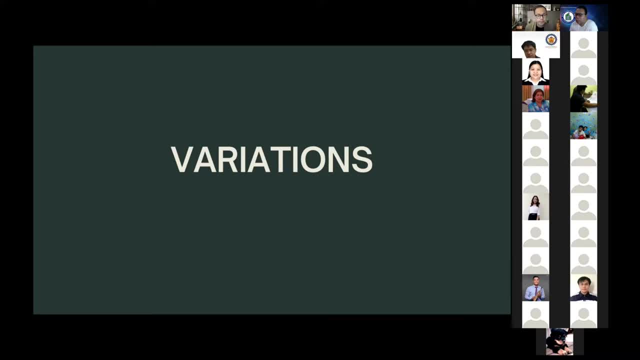 the instructions to vary the works unless they agree and enter into a new contract. So therefore, absent a clear provision for variations in the construction contract, the contractor cannot be compelled to comply with instructions to vary the works. And that's where the standard conditions of contracts prove to be useful. And in cases of 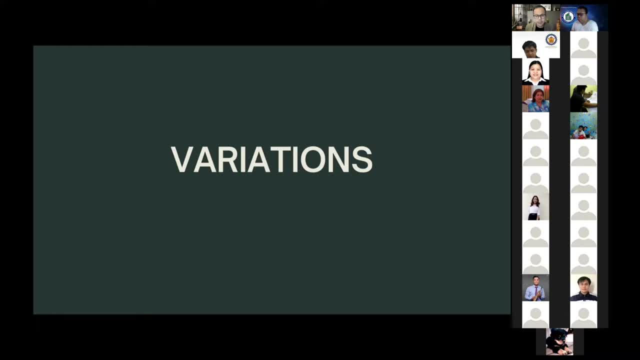 bespoke contracts. they are not considered to be necessary as the contract is not required and the contractor can be swayed by the contract. Therefore, this process is something to look out for. A variation mechanism or procedure is important so that disputes could be avoided in the event. 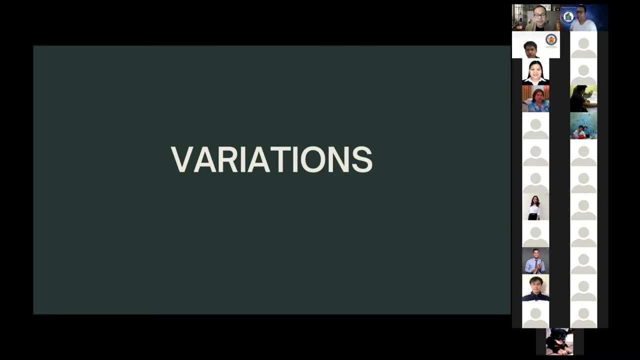 the contract needs to be varied. All standard forms of contract that I have described earlier includes within them a provision that allows for the works to be varied. So in this section we will be discussing the nature of the variation, an instruction to vary the contract and the procedure that is to be employed to accommodate. 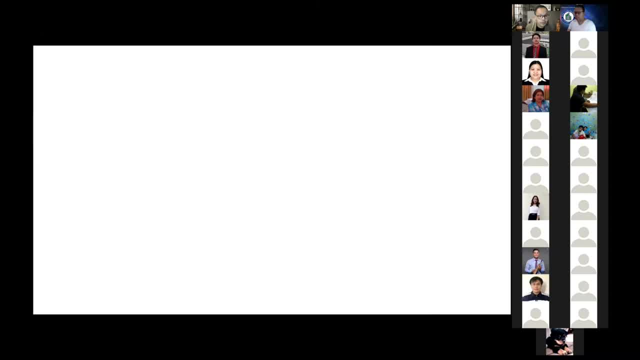 these variations? So what is the nature of variation? What is variation? So there are various circumstances that may give rise to instructing a variation, such as, inter alia, changes to specifications and quantities, discrepancies between the construction drawings and the contract drawings, and so on and so forth. So variation also may arise from conditions. 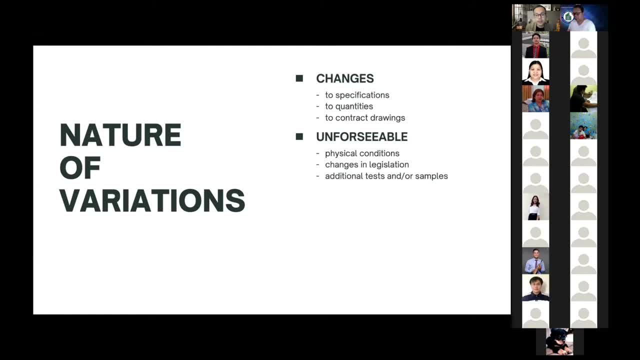 which are unforeseeable to both parties when the contract was concluded. It is important to note, however, that the wordings and descriptions, including specifications, provided in the contract are not limits to what a variation is, And then in cases where compliance to the construction. 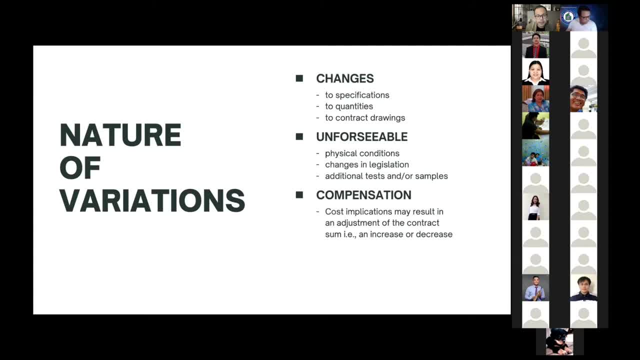 sorry, instruction will lead to the contractor incurring additional costs. the contractor may, according to the provisions of the contract, be compensated in terms of monies, extension of time for completion, or both. While a specific work is not mentioned in the descriptions, it is generally accepted that the contractor has 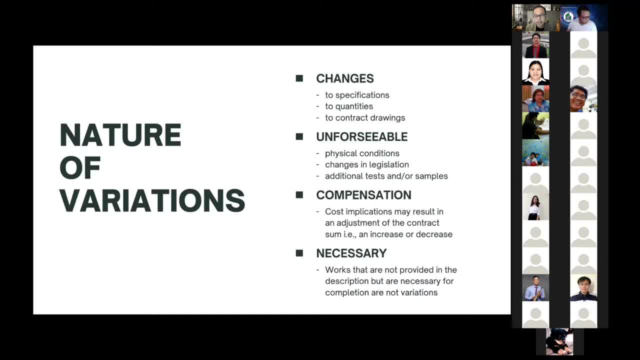 an implied obligation to carry out the works and bring such works to completion. So, therefore, all the works which are indispensably necessary are included and does not give rise to, in other words, a variation, In other words, if a specific work that is not included in the 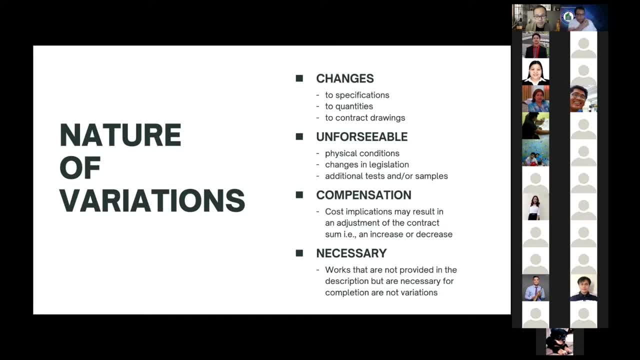 description in the bills of quantities or in the specification in the contract documents, but indispensably necessary, meaning the contractor cannot bring that specific work to completion without carrying out that work, then that is not a variation order. So who then has the power to? 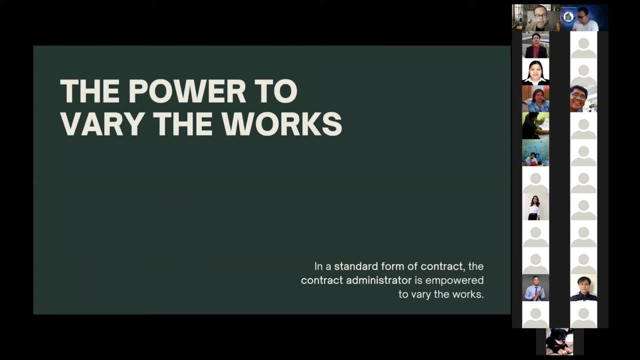 vary the works. So in a standard form of construction the contract administrator is empowered to vary the works. Absent the express provision in the contract, the contract administrator does not have the power to vary the works In the standard conditions of contract. 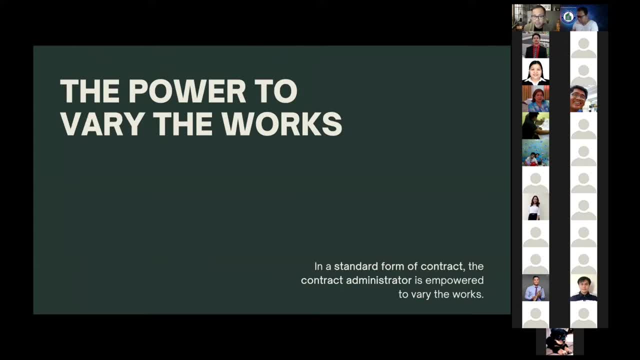 the contract administrator acting as the employer's agent has the power to vary the works In case of FIDIC Red Book 2017,. this power is provided in sub clause 13.3, which we call variation procedure. The sub clause provides that the engineer 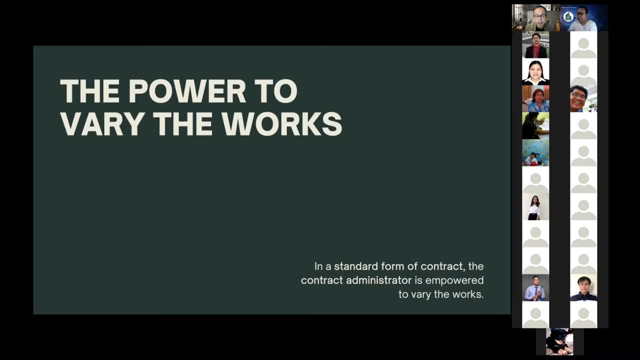 is empowered to issue an instruction to vary by way of a notice describing the required change, and should state any implications on costs. The engineer who is the contract administrator under the FIDIC Red Book at any time prior to the issuance or issuance of taking over certificate. 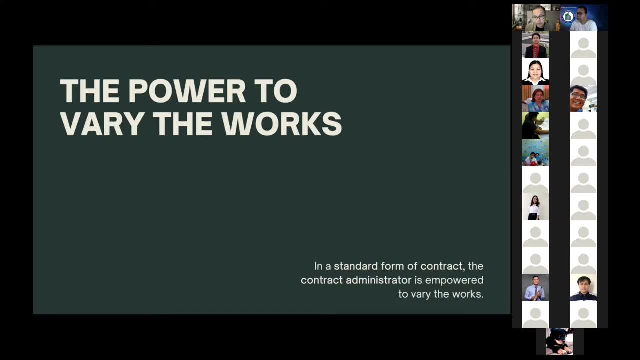 may initiate a variation orders by issuing an instruction or by requesting from the contractor a proposal to take over the certificate. The FIDIC Red Book 2017 has the power to vary the works. The contract administrator is empowered to vary the works In case of FIDIC Red Book 2017,. 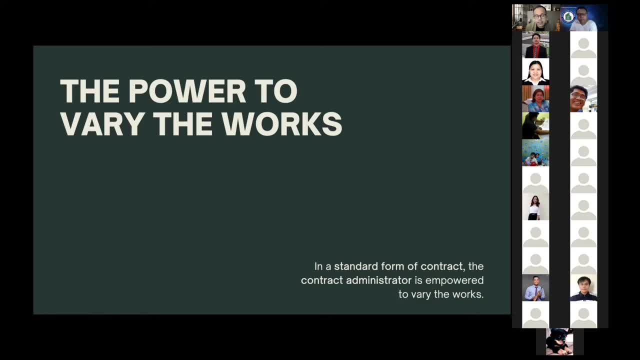 this power is provided in sub clause 13.3,, which we call variation procedure. The contract administrator at any time prior to the issuance of the instruction. If your contract is bespoke, meaning it is not in a standard form, you must check your contract on who is the person empowered. 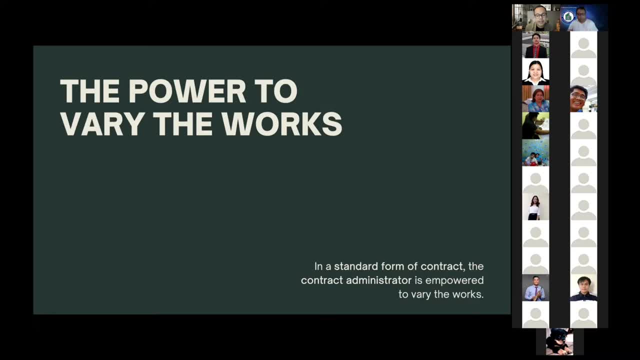 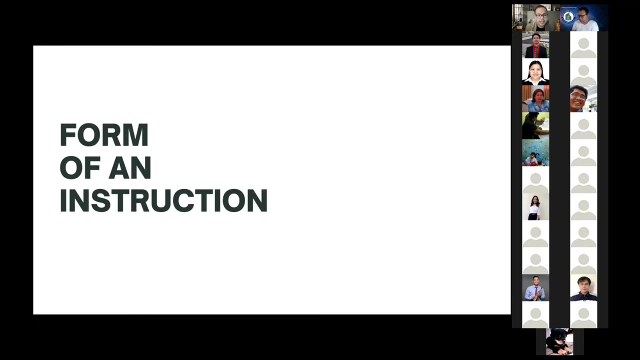 to issue the variation instruction and make sure that any instruction to vary the works is in line or is compliant with what is provided in the contract. So there are various circumstances that may give rise for instructing a variation order And when those circumstances arise. 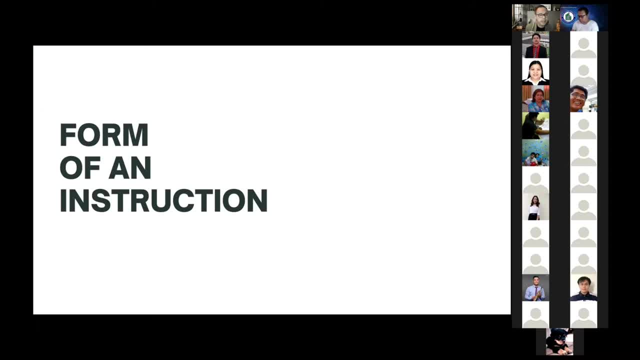 what form does an instruction take? So, first, the instructions should be in writing. So any instruction to vary must be in writing. It doesn't have to be necessarily in a letter, but it should contain express instructions to specify the change that must be made. 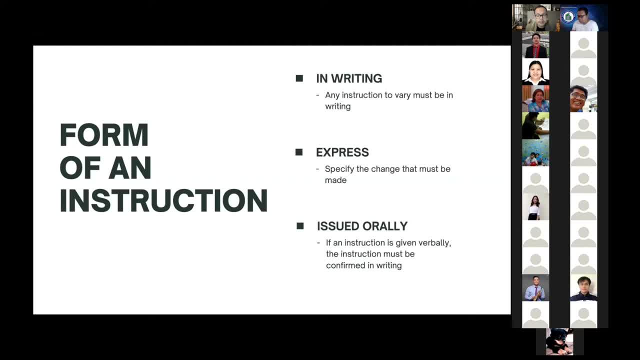 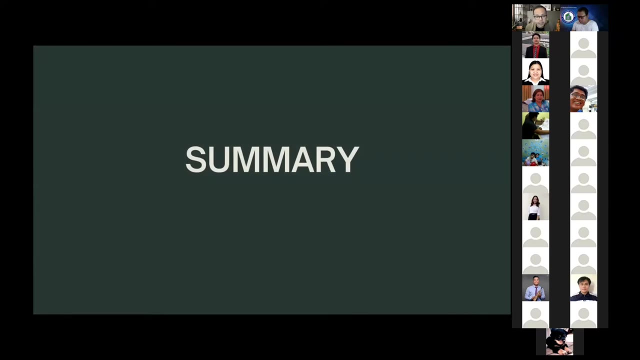 If the instruction is issued orally, then the instruction must be made or must be confirmed in writing so that it will comply with the in writing requirement. So finally, as a summary to this section, variation clauses, when incorporated in the contract, ultimately will afford the contracting parties. 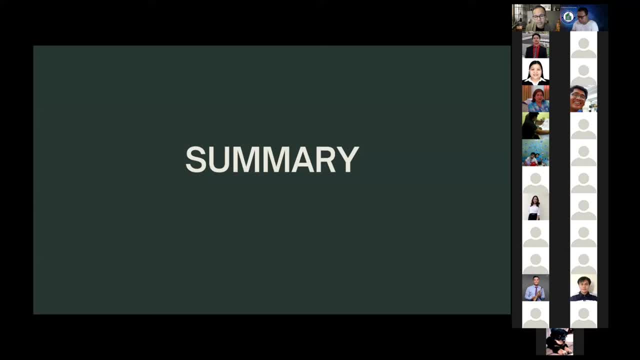 a certain degree of flexibility insofar as the scope of the contract is concerned. However, once an instruction to vary is issued and absent any valid reason to resist compliance, the legal implication of an instruction to vary is that the contractor is the contractor's necessary compliance. 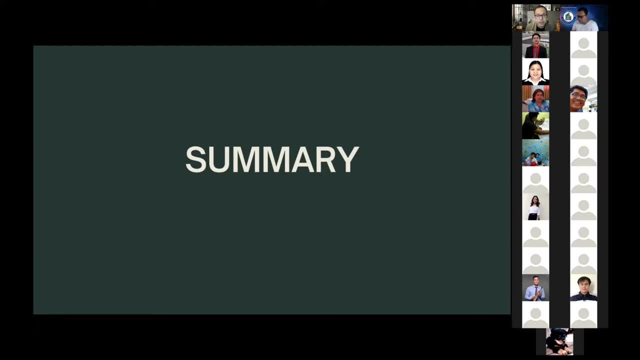 Since the effects of the variation can either increase or decrease the contract sum, these clauses also inevitably cause uncertainty to the budget of the whole of the project. Therefore, management of the variations is necessary to keep the project within the limits in terms of costs. 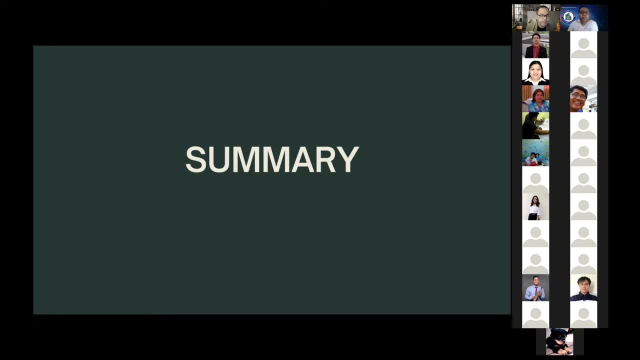 So, after discussing, or having discussed, variations, we will now proceed with the next sub-topic, which is the extension of the contract. Next slide, please. So most, if not all, construction contracts are time-barred, In a sense, the contractor shall deliver the contracted works. 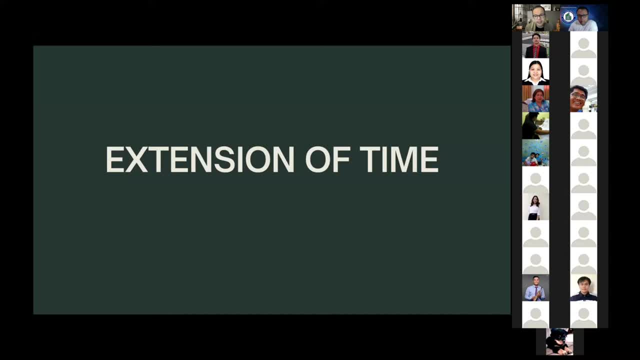 or services within the agreed date. If the contractor fails to do so, the contractor is in breach of contract and therefore the employer may be entitled to recover liquidated damages or any remedy expressly provided in the contract. However, if the contractor, at any point, 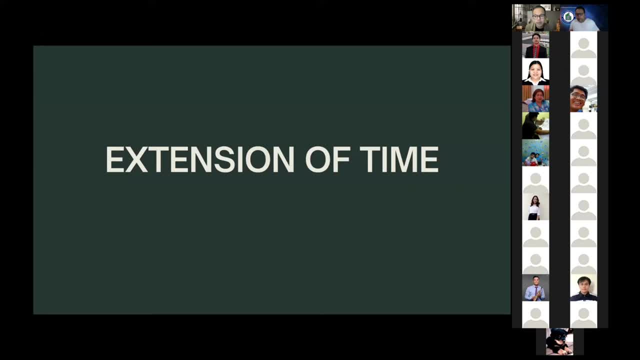 in the performance of the contract was disrupted or prevented by the employer or by events which are beyond its control, the contractor may be entitled to extension of time. This section will explore and discuss the legal basis for the extension of time and its legal underpinnings. 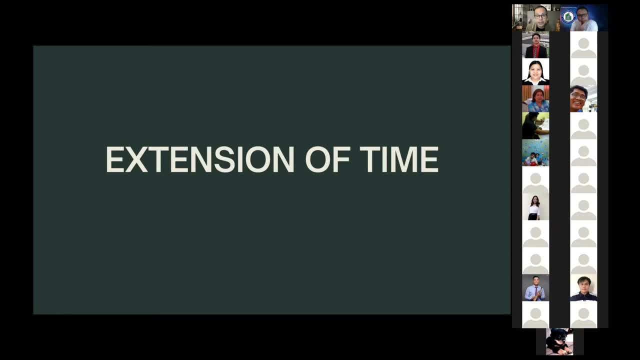 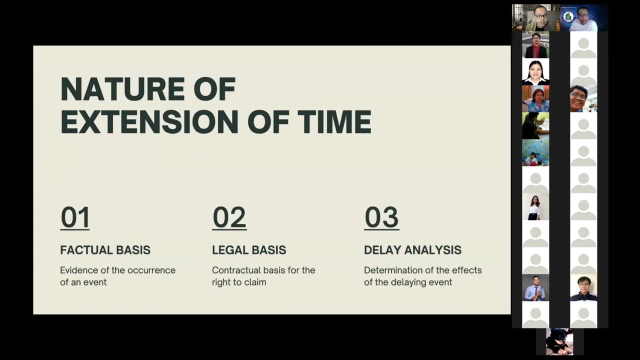 under the issues and other issues surrounding timing. Next slide, please. So extension of time clauses are indeed important, as they preserve the rights of the employer to recover liquidated damages and enable the contractor to be informed of their financial exposure when delays occur. First you have to establish when claiming 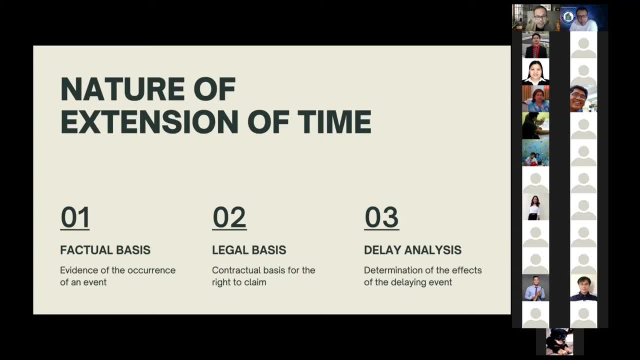 for extension of time is the factual basis. The contractor has an implied obligation to bring the contracted works to completion without delay, meaning within the contract period. Therefore, if the contractor is interrupted or the contractor must be compensated with time or money or both. 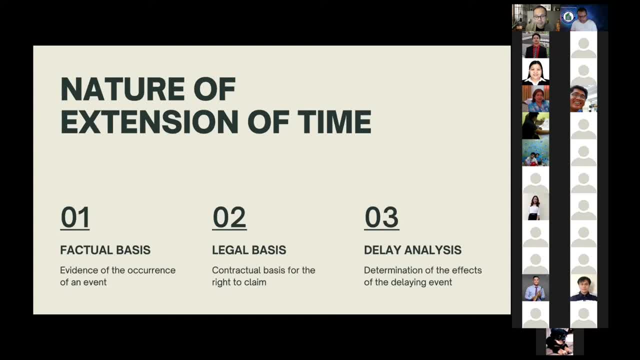 provided that the delay was not caused by them. this is the first burden that the contractor must overcome for them to be entitled to extension of time that delaying event is not attributable to them. Proof of the delay or proof of delay of the event occurring must be documented. 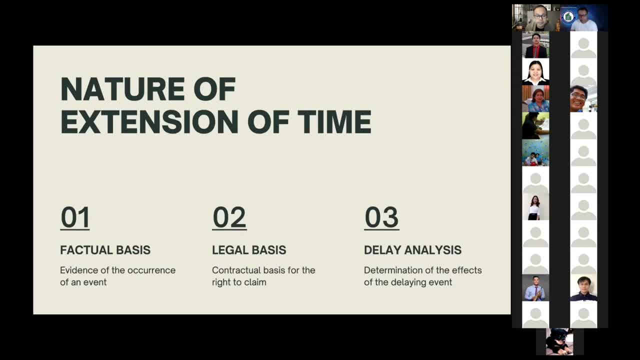 and shall be included in the submission of notice or claim. The second burden that the contractor must overcome is the establishment of the legal basis. So, while the right to extension of time is in the contract, it is not automatically given. Therefore, if the contractor deems the delay incurred, 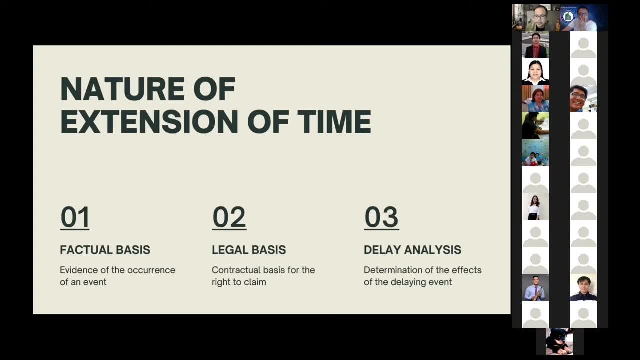 are excusable, meaning not caused by them. the contractor must reserve its right to extension of time by following the procedures set forth in the contract, such as submission of notices in the prescribed form, clearly identifying the entitlement and including all information and substantiation. 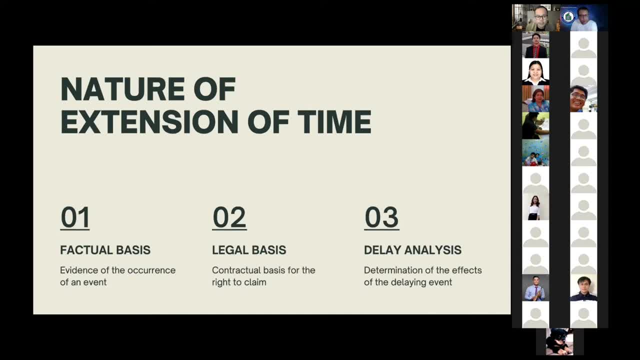 within the time bar. Most contracts provide a duty to mitigate as a condition preceded to the entitlement for extension of time. So you have to also prove that you have mitigated and have noted your choice after doing mitigation measures, that you still will be delayed. 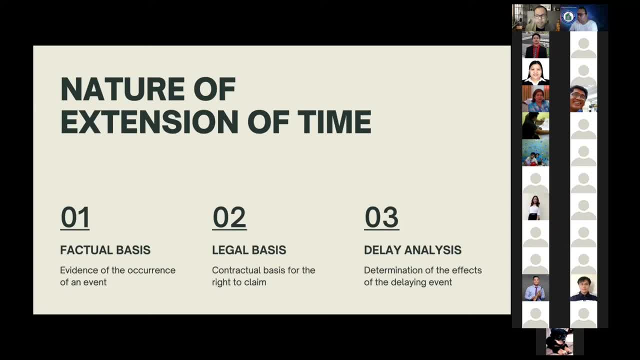 And then, finally, the third burden, and probably the most difficult burden to overcome, is proving that you have been delayed. So this is what we call the delay analysis. For the contractor to be entitled to an extension of time, the contractor must prove that the event 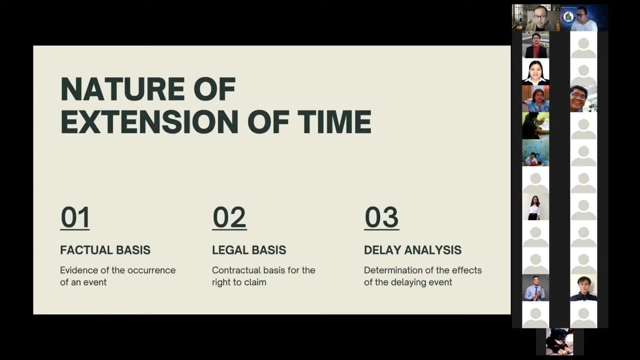 which has occurred has caused them delay. There are several delays: delay analysis, procedures to determine the effect, or the lack thereof, of an event. Delay analysis will also lead the determination- sorry, the delay analysis will also lead to the determination of the quantum of the delay. 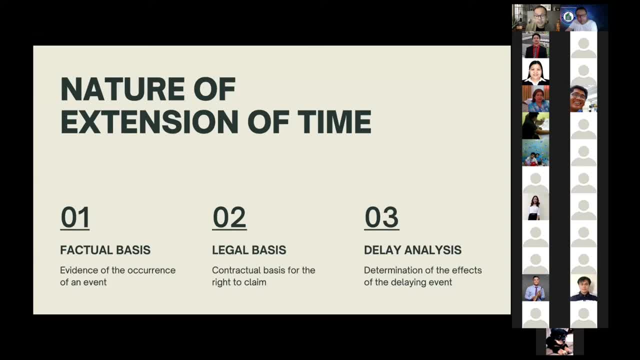 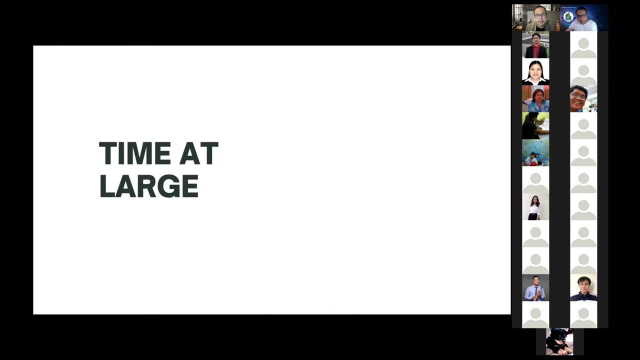 in terms of days, months, et cetera, and the cost that comes along with it, such as loss and expense and other damages that are due under the contract and under the law. So what if the contract does not have an extension of time procedure? 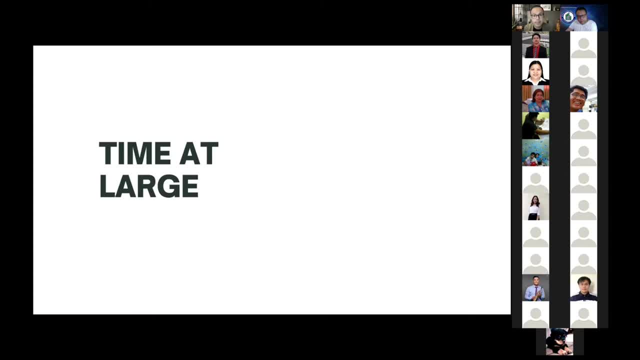 or does not have an extension of time mechanism, Then we consider that the contract is at large. So, as mentioned earlier in the slides, construction contracts are time barred, in a sense that they must be performed and completed within the agreed period. But what if the contract does not contain such mechanism? 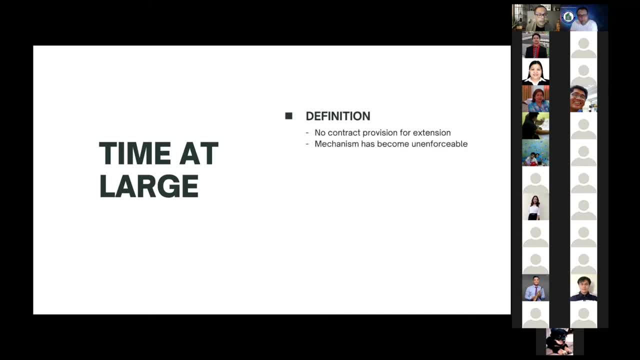 So the contract enters a state that we call time at large. So when the contract is set at large, the time is no longer binding on the contractor, So time is deemed to have been at large when the agreed completion date expires and that there is no mechanism in the contract. 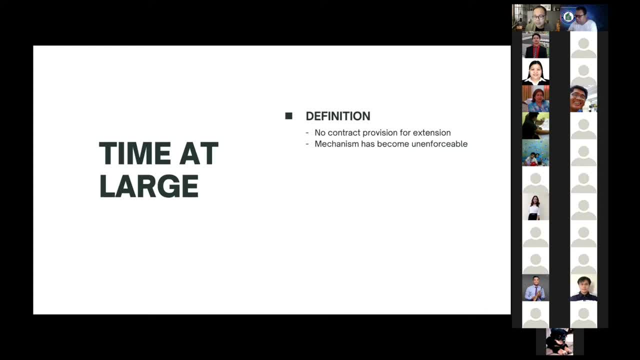 that allows for extension, Or when the mechanism in the contract has broken down and becomes unenforceable. So what is the effect? So the effect of the time being set at large is that the contractor is released from its obligation to complete the project within the agreed period. 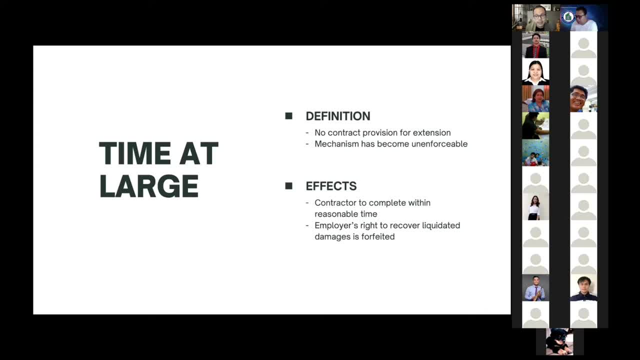 and the contractor is instead allowed to complete the project within a reasonable time. Furthermore, when the time is at large, the employer can no longer recover liquidated damages from the contractor arising from its failure to complete the project within the agreed time. So we've been discussing extension of time. 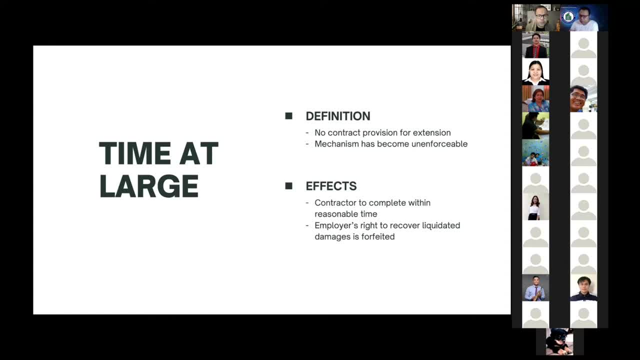 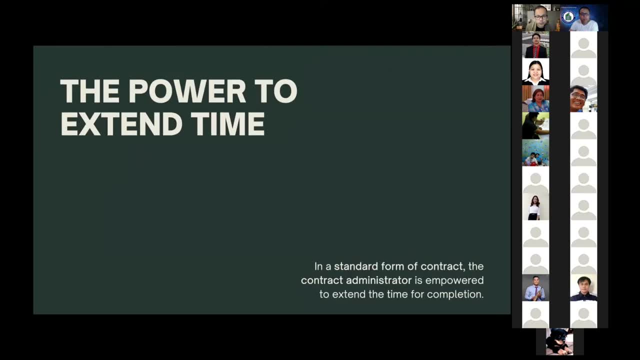 in the previous slides, but who has the power to, who is entitled or who is empowered to extend the time. So in standard forms of contract, it is the contract administrator who is empowered to extend the time for completion. The standard building contract gives the contract administrator 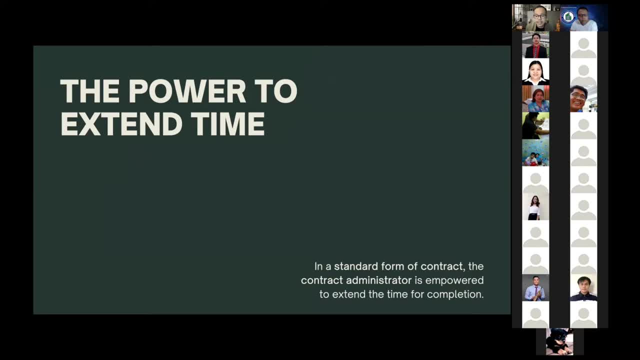 the power to adjust the completion date of the contract In cases where relevant events occur which delayed the contractor from performing his obligations, such as natural causes and acts of men. The contract administrator, upon receipt of notice from the contractor of the delay or occurrence of a relevant event. 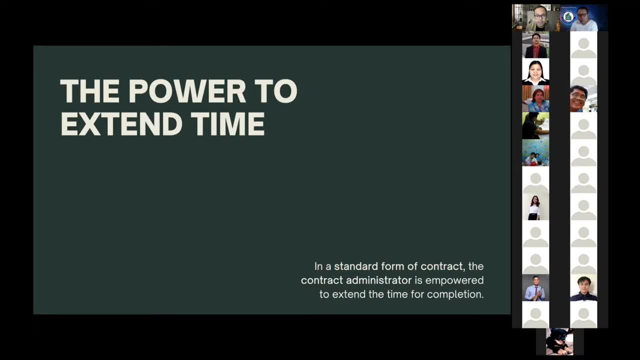 the contractor shall notify the contract administrator of such event, and the contract administrator will then reply within reasonable time before the expiry of the time bar. So, while the contract administrator has the discretion in granting the extension, the arbitrator or the court may intervene in circumstances. 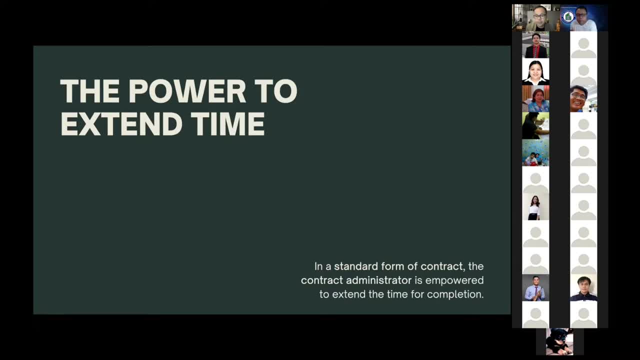 where an allegation of bias or inequity in the decision is present. This was the position of the court in the case of John Barker versus London Portman, where the court held in that case that the court or an arbitral tribunal may open and review the decisions. 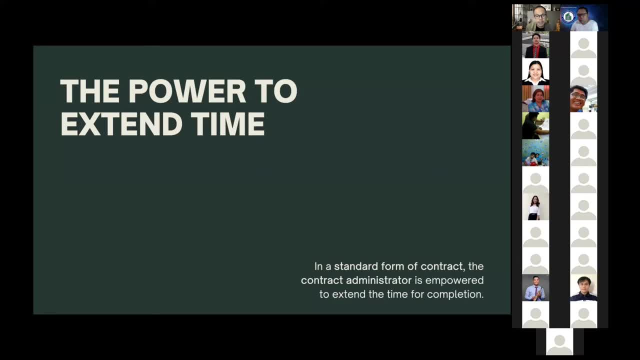 of the contract administrator, when the mechanism provided for in the contract has broken down or when the application of the provisions of the contract are incorrectly applied or interpreted, which resulted in a manner that is biased to 140 and therefore not fair. So what are the delaying events? 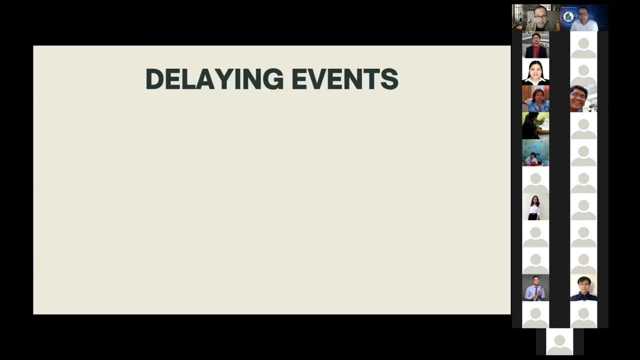 So I have classified the delaying events into three categories, So delaying events or events which were caused by the employer, which delaying events which were caused by nature and other events which cannot be classified on the employer in nature. So among the risks or among the delaying events. 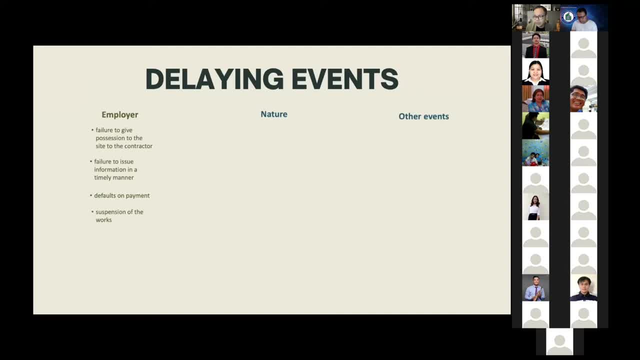 caused by the employer is failure to give possession to the site to the contractor, failure to issue information in a timely manner, defaults on payment, suspension of the works, instructions relating to variations and provisional sum delaying events which were which are of natural causes. 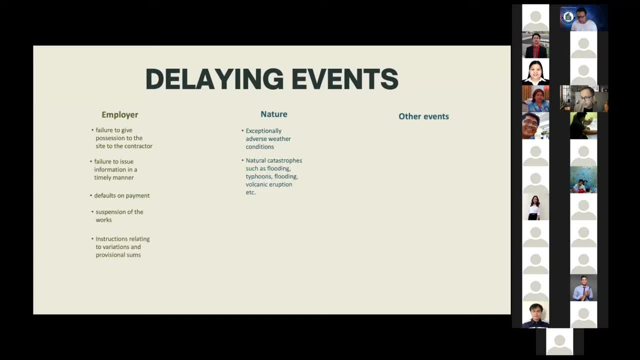 or exceptionally adverse weather conditions, natural catastrophes, force majeure and epidemics, which may result in movement control or restrictions. Other events are changes in legislation, civil commotion, such as wars, terrorism and strikes, and shortage in manpower or labor, and changes in statutory requirements. 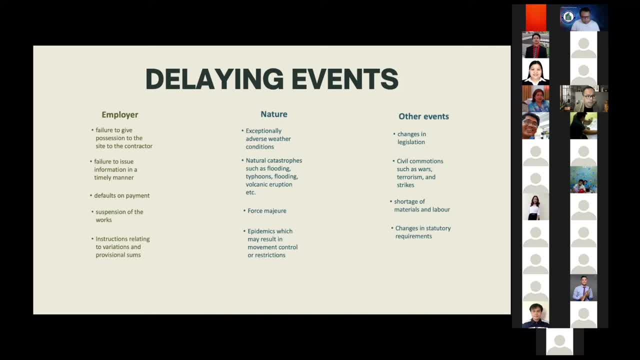 So, as you can see, the current pandemic there, the delaying event of the caused by or the pandemic being a delaying event is not necessarily under the contract. However, the circumstances or the events resulting out of the pandemic may qualify the contractor to extension of time. 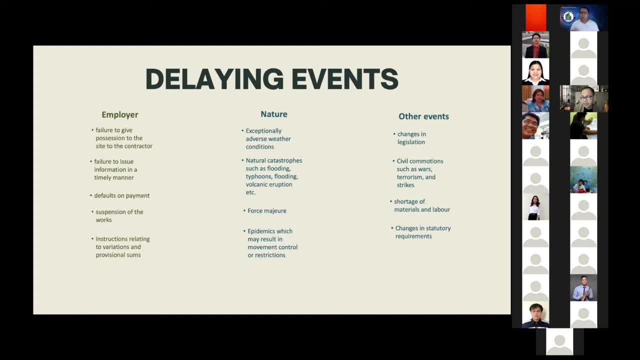 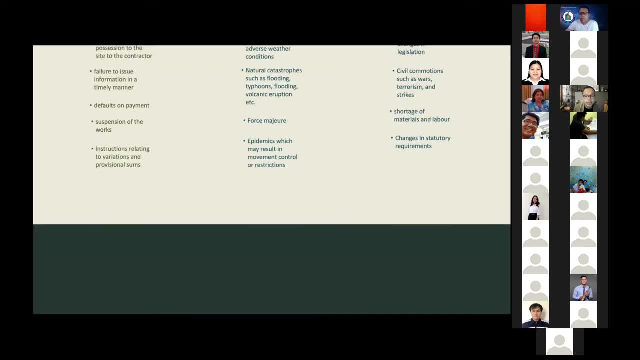 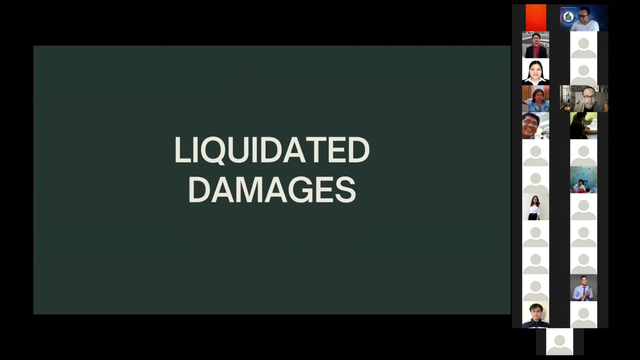 So I'm expecting questions about this later in the question and answers. So, having discussed the extension of time, we will now be proceeding with the discussion on liquidated damages. What is liquidated damages? So it is important to distinguish damages arising out of the breach of contract. 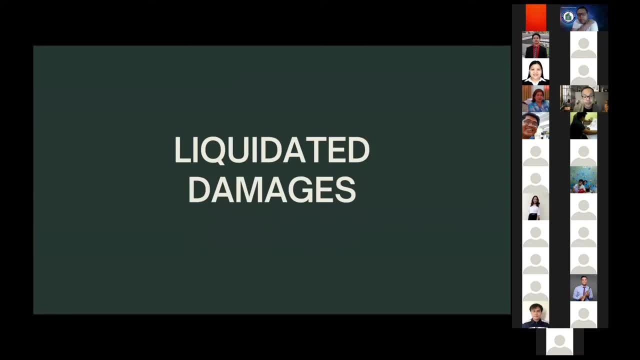 and claims which arise out of the term, out of the terms in the contract. So, therefore, this section will explore and discuss remedies for breach of contracts, such as liquidated damages, and contractual claims, such as claims for direct loss and expense, global claims. 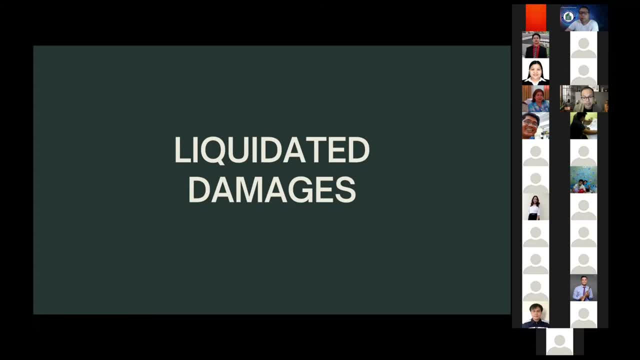 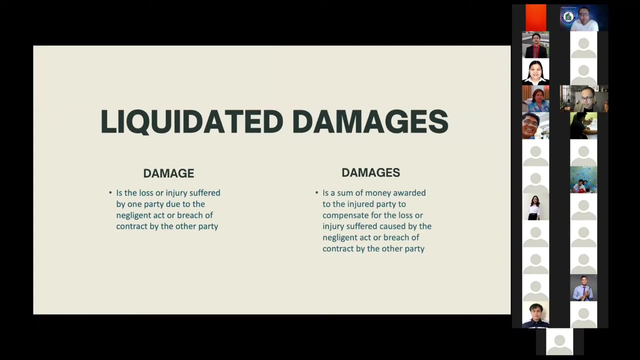 et cetera, which are rooted in the mutual liability, which mutual liability claims for the compensation of both the employer and the contractor. But before proceeding with the discussion, it is important to distinguish damage and damages. So damages are compensatory in nature. 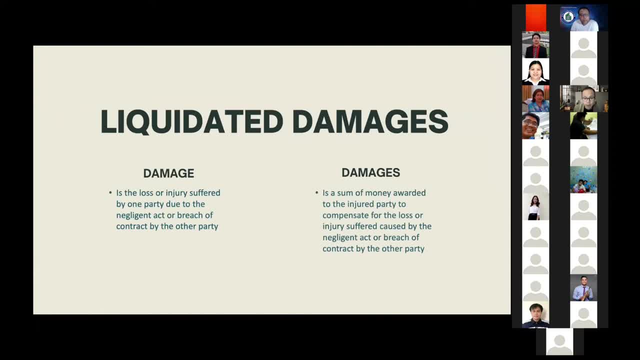 In other words, damages are a sum of money awarded to the party who suffered loss or injury due to a breach of contract. The objective of damages is to restore the status of the injured party to a state that is as if the injury or loss did not occur. 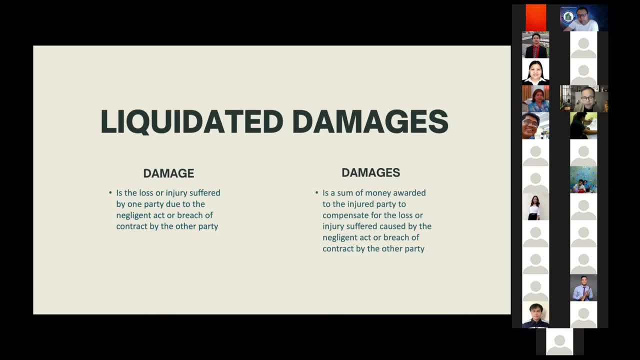 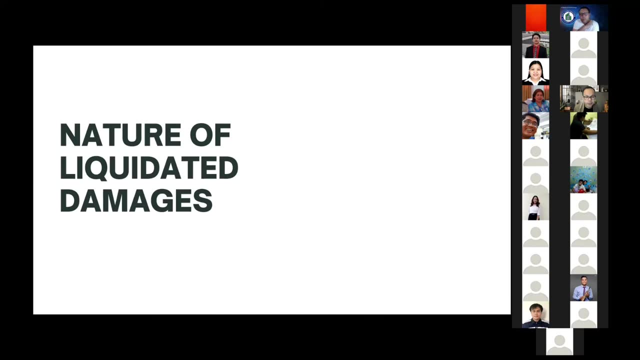 Damage, on the other hand, is the loss or the injury suffered by one party due to the negligent act or breach of contract by the other party. So what is liquidated damages then? So where a contract exists, the terms of contract will generally provide a mechanism. 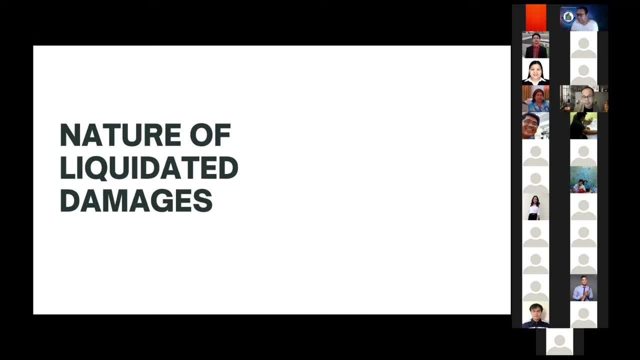 to remedy the party's breaches. When the employer defaults or fails to perform its obligation, the contractor is entitled to extension of time. However, if the contractor defaults on its obligation to complete the project within the contract period, the employer is entitled to recover. 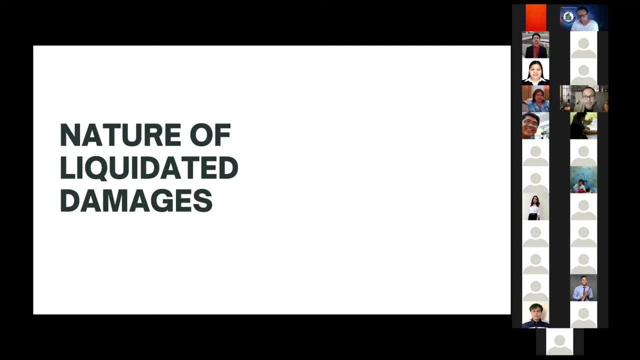 what we call liquidated damages. So hence the question: what is liquidated damages? So liquidated damages are an agreed summary or an agreed sum of money that becomes payable by the contractor to the employer in the event of the contractor's breach, say, for example, delay in performance. 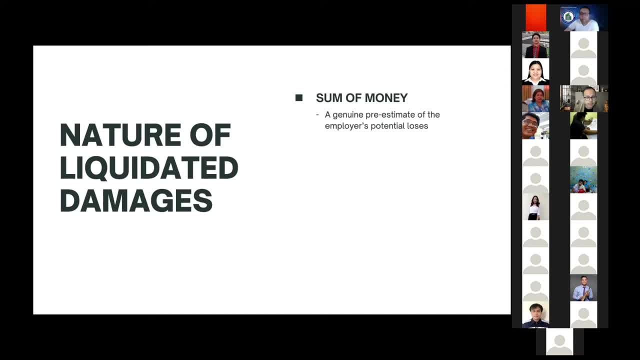 or what we call culpable delay, Liquidated damages or liquidated certain damages in some jurisdictions, is a genuine pre-estimate of the employer's potential losses, which may include loss of profit or income, cost of financing, alternative accommodations, and so on and so forth. 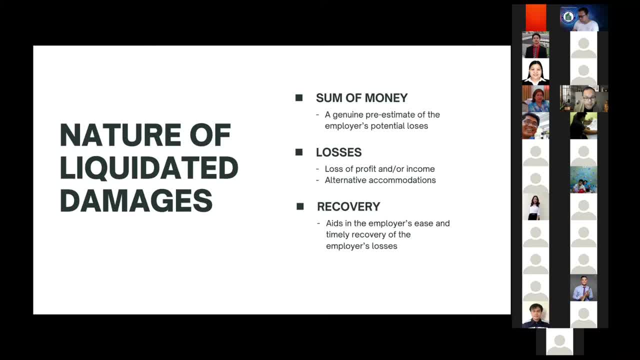 In determining the exact or precise number of damages that is brought about by a delay in performance can be inexpensive, challenging and time-consuming. So therefore, the parties agree in the outset a figure that is likely to be the sum of money that will be come. 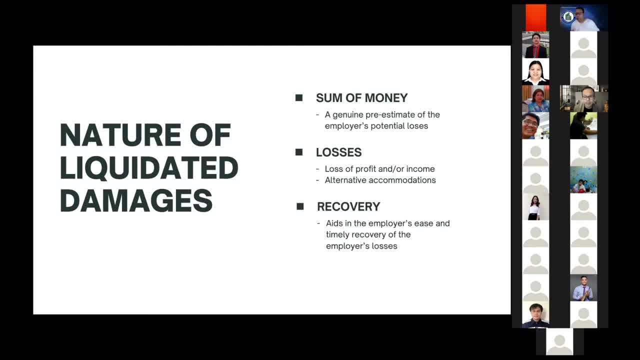 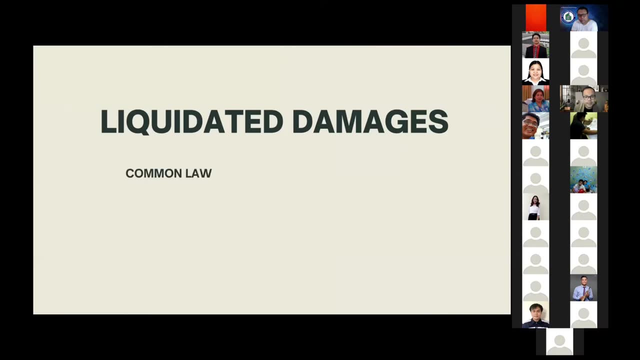 or that will be the loss of the employer, and then it will be recovered by the employer from the contractor when a culpable delay occurs. So that's the nature of liquidated damages, And I would also like to highlight the difference between the liquidated damages. 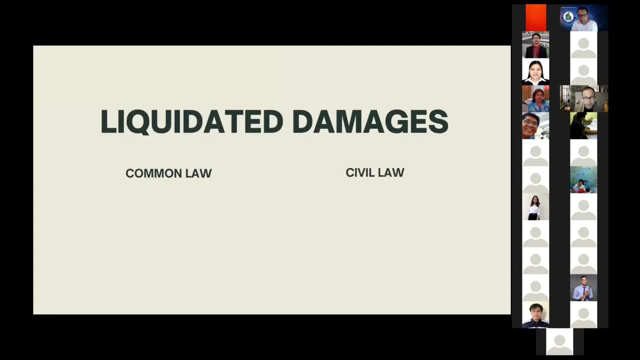 in common law jurisdiction and in civil law jurisdiction. So common law countries or common law jurisdictions are countries such as Australia, United Kingdom, Singapore, Canada and so on and so forth. So in these jurisdictions the liquidated damages are unenforceable. 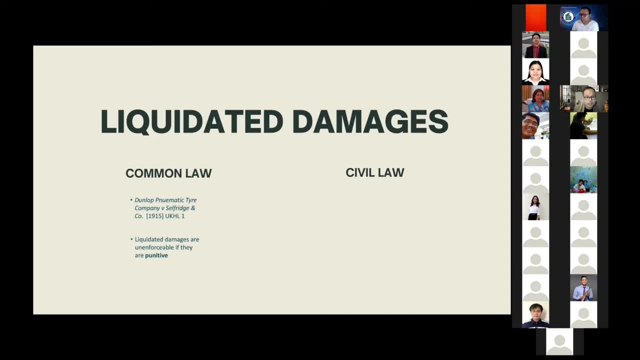 if the delay or, sorry, if the sum, is punitive. So liquidated damages in a construction, sorry, in a common law jurisdiction- is not a penalty. This concept was established in the case of Dunlop Pneumatic Tire Company versus Selfridge and Company. 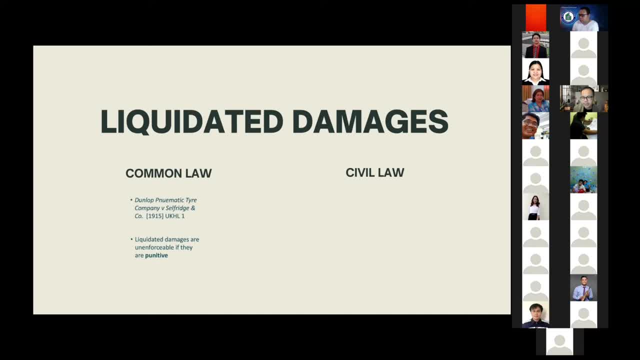 So in that case the court held that while the liquidated damages is a genuine pre-estimate of losses, it may be deemed as a penalty when, first, the sum is extravagant and unfair when compared with the greatest loss that can be proved to have arisen. 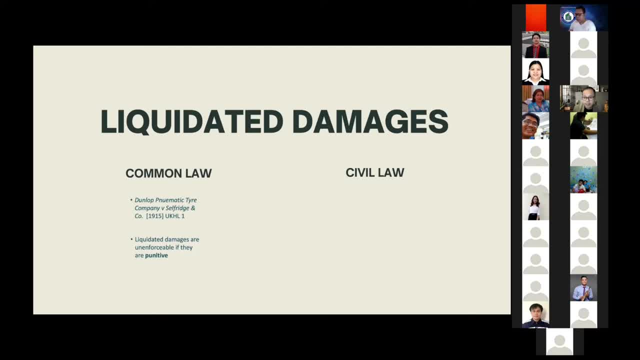 out of the breach, Or it is considered a penalty when the sum is greater than the sum which ought to be or which ought to have been paid. And, finally, it is a penalty when the sum is made payable as a weight of compensation on the occurrence. 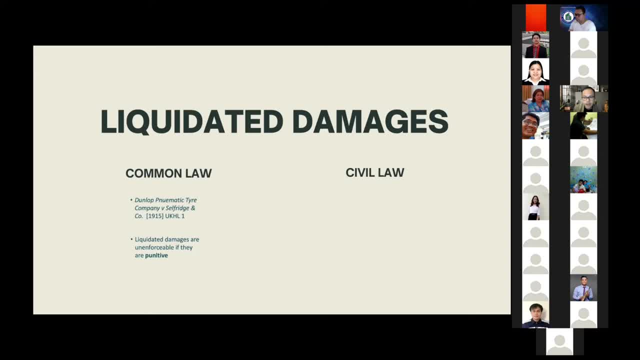 of one or more events which are serious and which are not serious and others but trivial or trivial in nature. This was the ruling as well in the case of Phillips versus Attorney General of Hong Kong. So in a nutshell, in a common law jurisdiction. 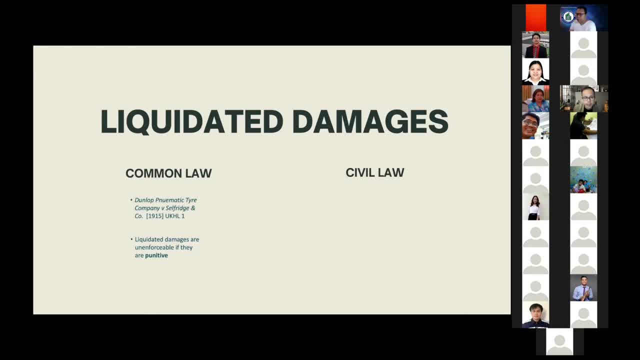 if you are practicing in a common law jurisdiction, a liquidated damages clause is unenforceable if it is punitive, meaning it acts as a penalty When contrasted in the Philippines or in a civil law jurisdiction such as the Philippines and other Eastern European nations. 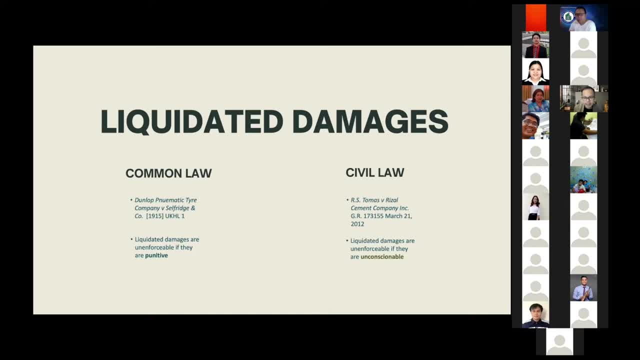 a liquidated damages clause, which may be seen as a penalty, is enforceable provided it is not unfair. This view is taken as an encouragement for performance of contractual obligations. While traditionally civil law countries do not distinguish between penalties and liquidated damages, the courts now 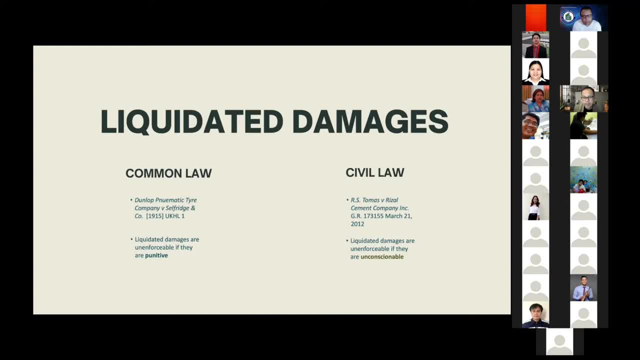 narrows the scope of the penalties clause and liquidated damages. So in recent cases, the liquidated damages clause, when found to be extravagant, is reduced to reflect a more realistic amount of the harm done to the claimant. This was the position of the Supreme Court. 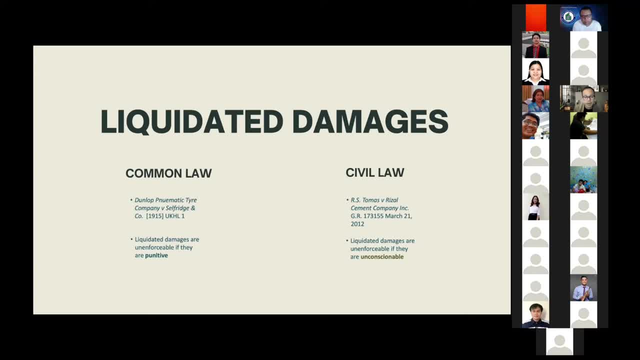 of the Philippines when it ruled in the case of RS Tomas versus Rizal Cement Company, where the court held that the decision of the lower court in reducing the amount of the liquidated damages because it is unfair is justified and correct. So there's the conundrum. 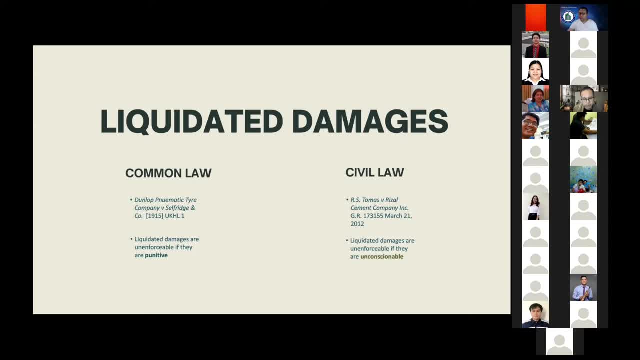 between a civil law jurisdiction and a common law jurisdiction. So in the Philippines, as I have said earlier, the courts consider liquidated damages as penalties to be enforceable. So what are the legal bases found in the legislation that we have, So in the Civil Code? 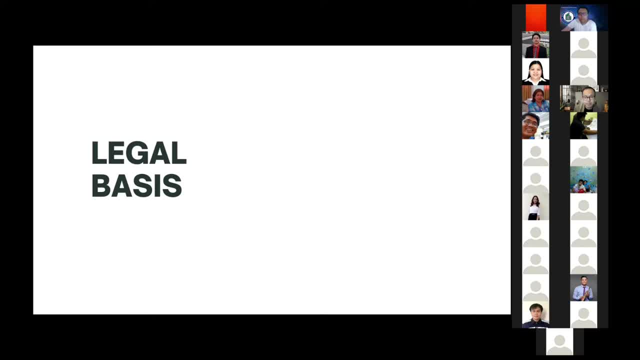 of the Philippines provides the legal basis for the nature and the entitlement of liquidated damages. Article 2226 of the Civil Code provides that liquidated damages are those agreed upon by the parties to a contract, and these are to be paid in breach or when a breach 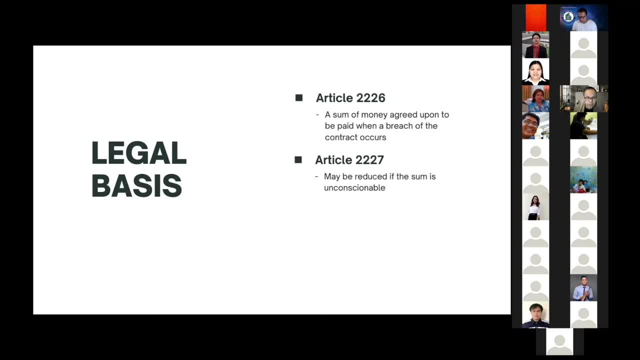 of the contract occurs In 2227, liquidated damages is defined or liquidated damages, whether intended as an indemnity or a penalty, should be equitably reduced if they are iniquitous or unconscionable, meaning unfair And finally, 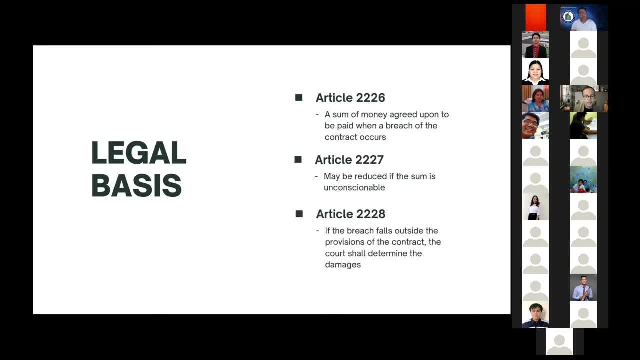 in Article 2228 of the Civil Code of the Philippines provides that the legal basis that, as the contract committed by the defendant is not the one contemplated by the parties in agreeing upon the liquidated damages, the law shall determine the measure of the damages and not the stipulation. 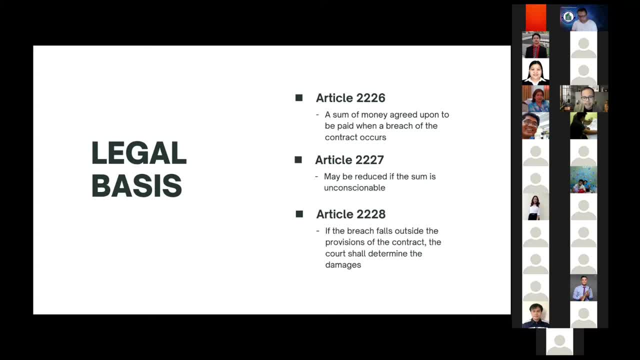 So what 2228 means is that the court has. when the sum or when the liquidated damages validity is put into question, the court has the power to determine the actual measures of the liquidated damages clause, Rather than what has been agreed. 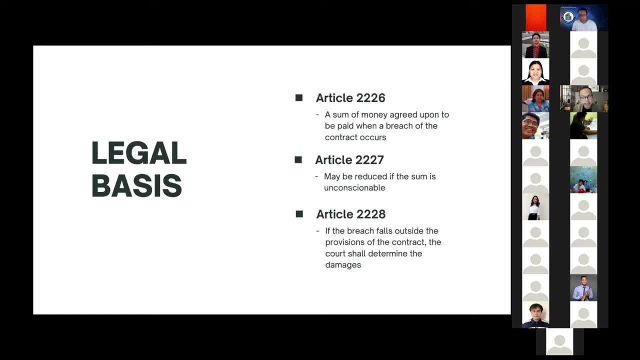 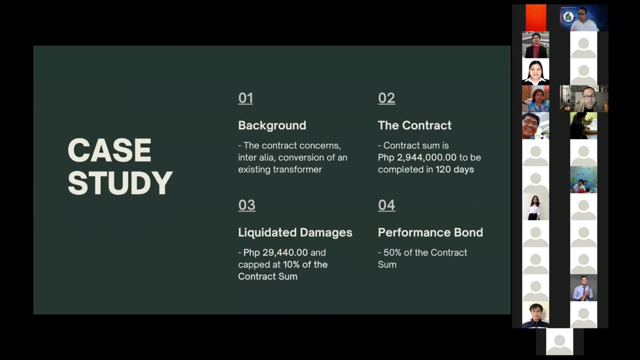 So the court can step in and revise the amount. So I have mentioned earlier the case of Arrest Tomas. So just to give you a brief case study or the background of this case. So Arrest Tomas and Rizal Cement Company entered into a contract. 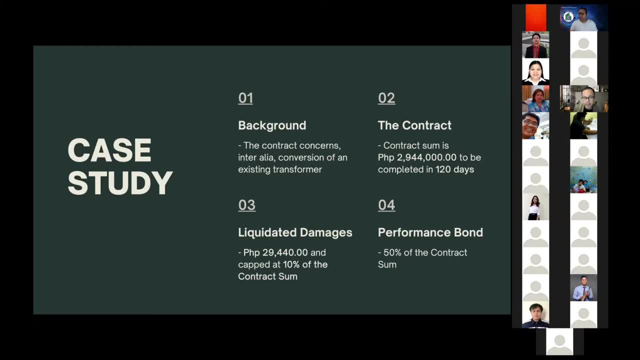 which concerns the supply of labor, materials and technical supervision for a series of job orders which, among others, is the installation of line system, primary protection switch and conversion of transformers. So the sum for the contracted works to which Rizal Cement agreed to pay. 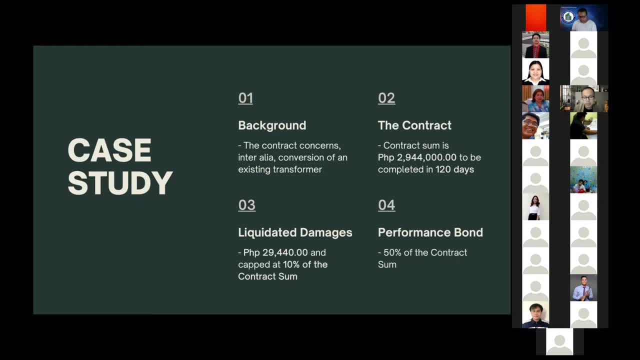 in exchange of Arrest. Tomas' performance is 2,944,000, which is due to complete after 120 days of the contract taking effect. So their contract provides for 29,440 per day of delay, which is the representation of the 10% of the contract sum. Arrest Tomas acquired a performance. sorry, the liquidated damages clause is capped at 10% of the contract sum, So Arrest Tomas acquired a performance bond amounting to 50% of the total contract sum, which is 1,458,000. 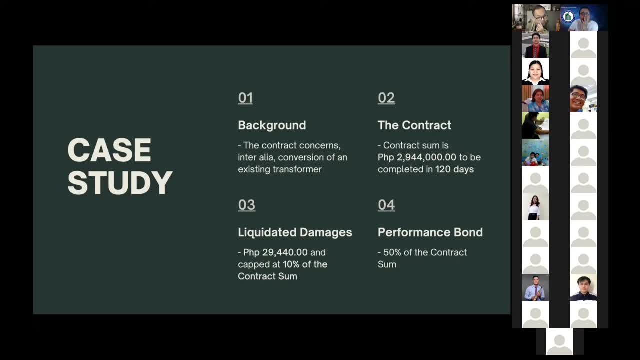 which is 1,458,618 for the full and faithful completion of the project. So during the course of the construction there were delays which were attributable to Rizal Cement, And this went to an arbitration and then the arbitration was appealed in court. 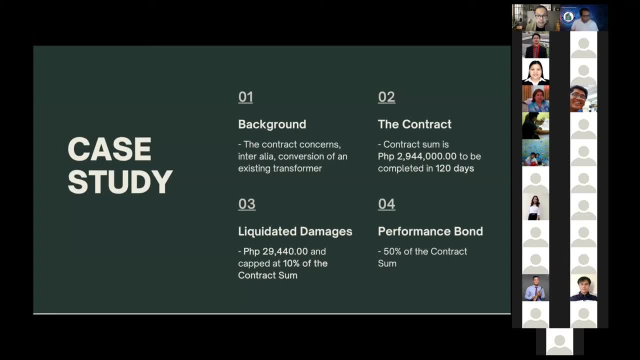 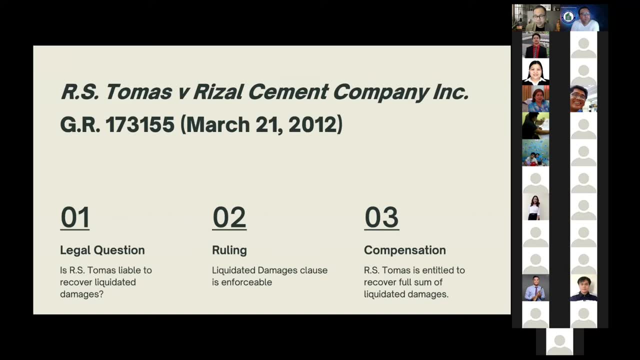 And the court. the Supreme Court intervened in 2012.. So the legal question which were put, among the other questions that were put before the court, is: is Arrest Tomas liable to recover liquidated damages? The court says yes, Its liability arises out of the liquidated damages. 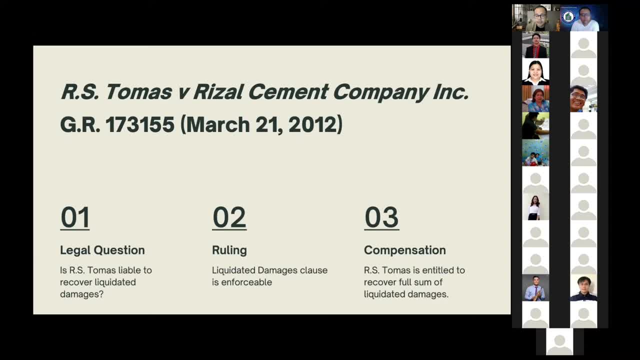 So the Supreme Court sustained the decision of the arbitrator. The court explained the legal principle of party autonomy, where the parties are free to enter into a contract And if the contract is concluded they are bound to its terms, including liquidated damages. 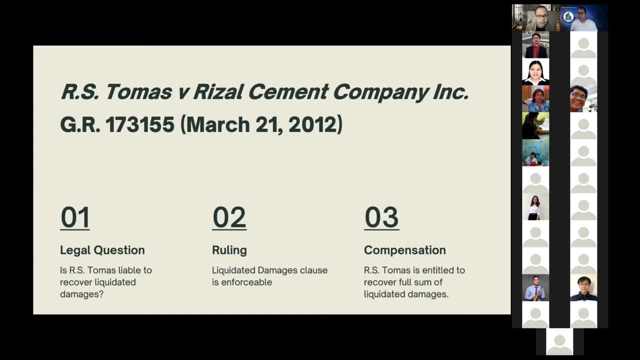 And by applying the same, the court ruled that Rizal Cement Company is entitled to recover liquidated damages from Tomas Arrest. Tomas defaults. The court awarded the full sum amounting to 10% of the contract sum, ruling that while the court 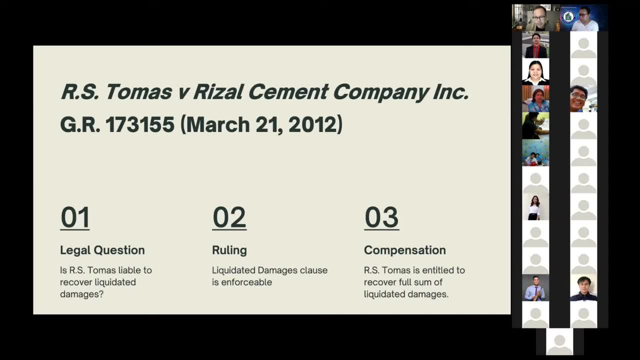 can reduce the amount of the liquidated damages in cases where it is unfair or unconscionable. it is not in this case. So, if we can, analyzing the case or the decision of the Supreme Court, if your current contract has a limit of 10%, 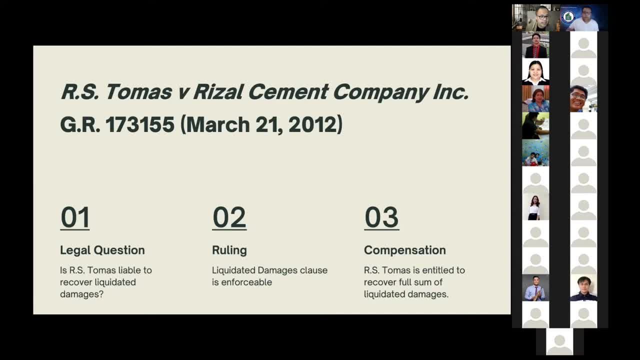 of the total contract sum that is deemed to be fair and reasonable by the court. So there are other similar cases to this Arrest, Tomas, which were decided earlier, such as the Filinvestland versus Pacific Equipment et al and the Urban Consolidated. 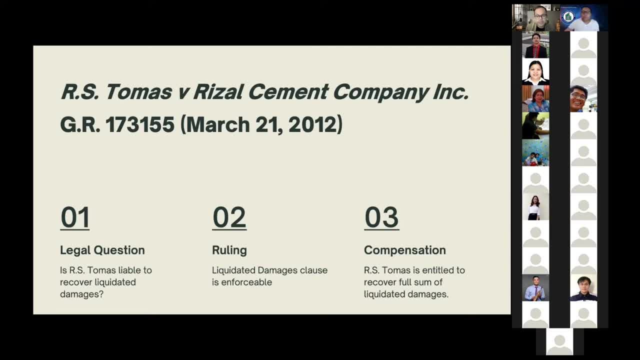 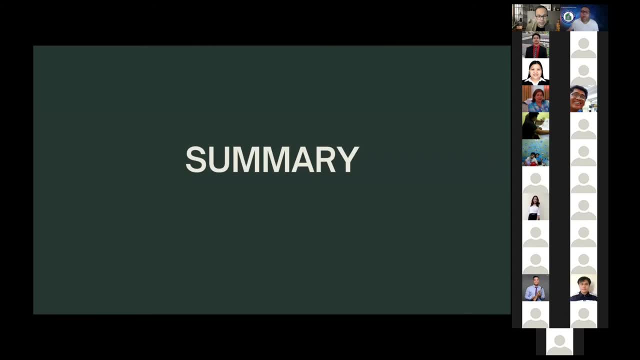 Contractors of the Philippines versus Insular Life Assurance Corporation. So, in conclusion, liquidated damages are genuine pre-estimate of the likely losses of the employer in the event the contractor defaults on his obligations to perform the contract within the agreed construction contract Or within the agreed. 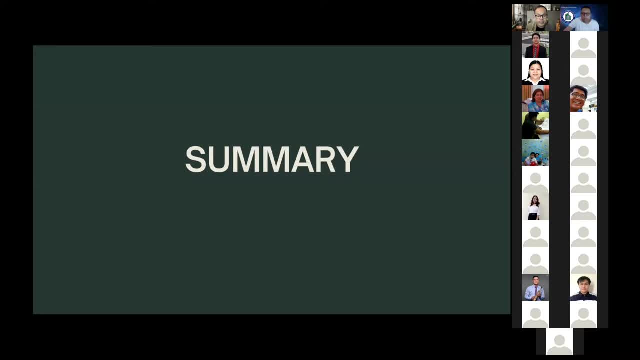 contract period. liquidated damages are agreed upon by the parties on the onset or on the conclusion of the contract. If questioned insofar as its intentions is raised to a court, it will be reduced by the court if it is found to be iniquitous. 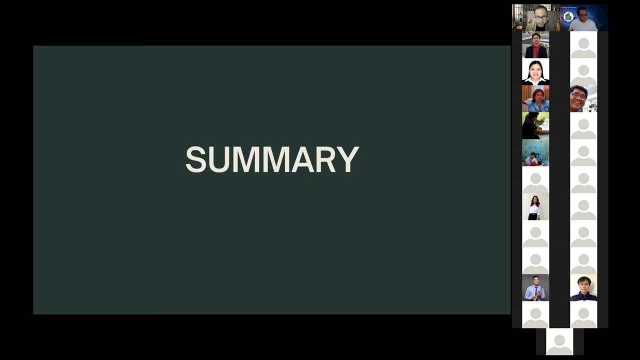 meaning immoral or unconscionable meaning unfair. While common law jurisdictions where the court will refuse enforcement if the sum is penal or trivial, in a civil law jurisdiction such as the Philippines, the civil court does not make a distinction between a penalty and the liquidated damages. 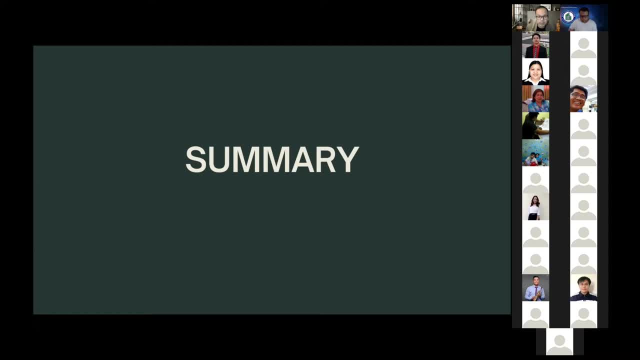 and therefore will enforce the agreed sum, except when it is again, as mentioned above, immoral or unfair. And with that the presentation ends and thank you for your attention, And we may now start the question and answer Or the lecture. Okay, 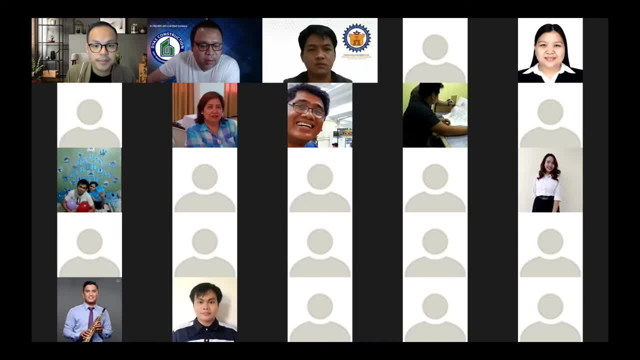 Thank you. Thank you, JC. Now there's a question here. Wait, Where is it? The nature of the contract administration is very legalistic because we are looking at the specifications and the specific terms in the contract. So it's important. 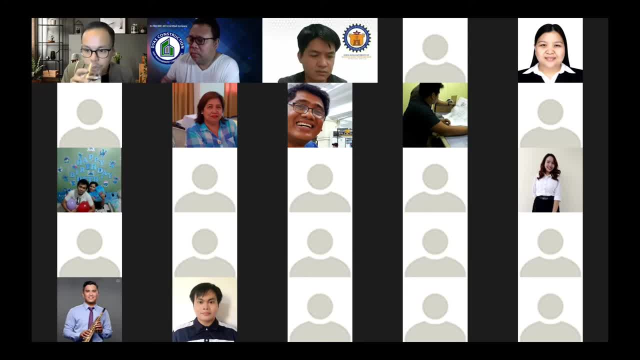 to have a very good legal basis. Okay, First question, Sir. Hi, sir. What is your insight regarding claims for extension of time and additional cost and expense due to the pandemic? Now he is referring to the COVID-19 pandemic. 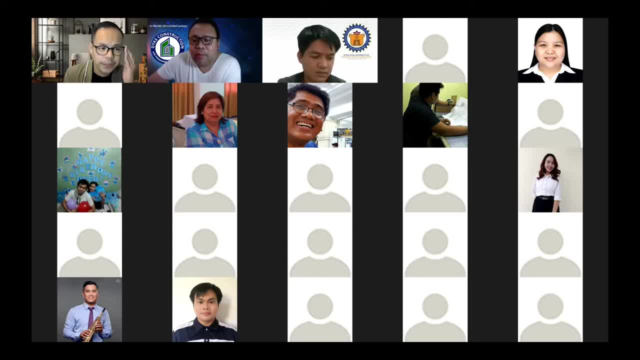 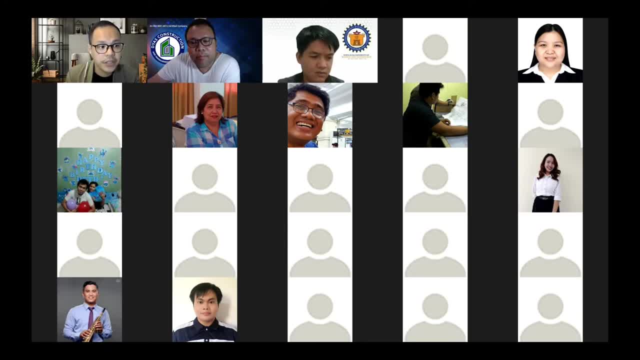 are arising out of regulations, out of the pandemic, Say, for example, movement controls, extra safety, preconditions on site, reduced labor, because we are reducing manpower on site to minimize transmission. So are these really arising out of the pandemic or are these? 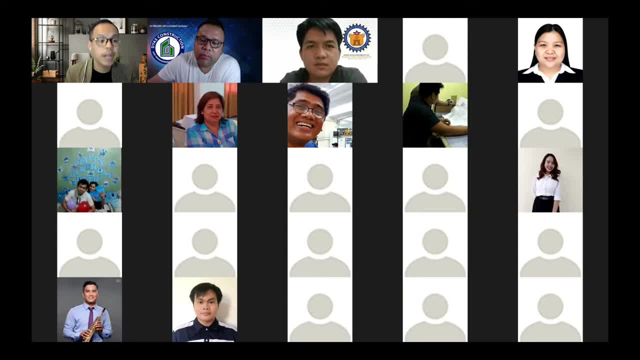 arising out of regulations or limitations brought about by the pandemic. So you have to differentiate that. And in cases or in contracts where they enumerate the list of the delays and pandemic is not there, you cannot claim directly for the costs arising out of the pandemic. 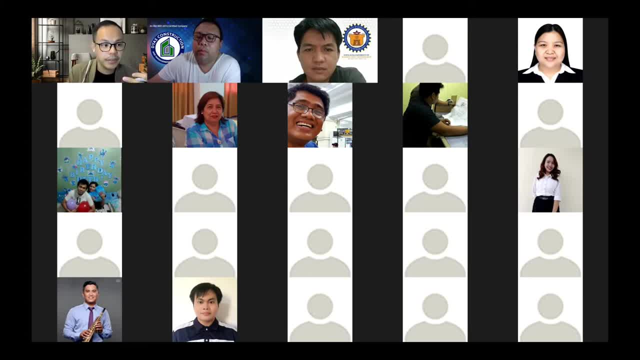 So you have to, in establishing your legal basis, you have to be sure on your grounds as to what contract provisions is concerned. Okay, Any other questions? Here is some comment. It says here that, depending on the contract provisions, cost entitlement. 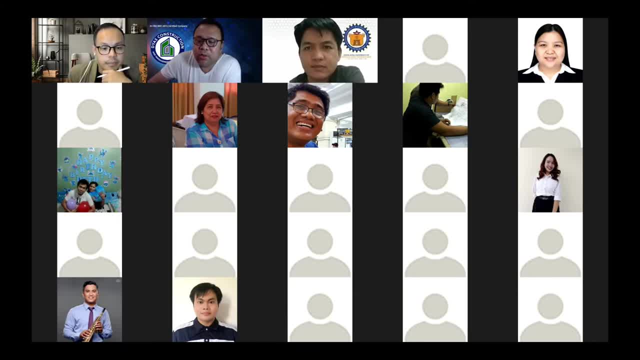 is valid due to the changes in legislations, which covers government directives or changes in law. So that view is correct. Okay, Any other questions? Do you have any other questions? I actually made my presentation quite short. It's less than an hour. 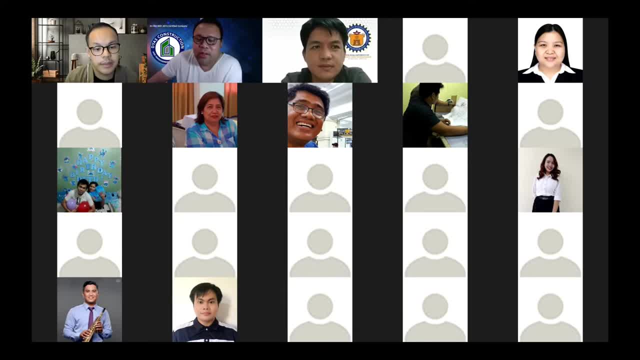 so that at least we can have ample time for discussion or questions. Any questions from the contractors? No Right to your questions. Those who raised their questions. You can unmute and ask questions if you can. Any questions, Clarifications, Comments. 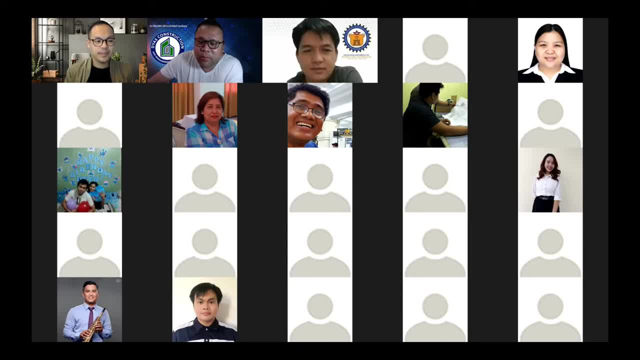 Suggestions: Hello, Okay, It looks like you understand it. Follow-up question from Ms Marites here. Yeah, Let's talk to her. Hi, sir, Is the extension approval? Yes, You can. that will be under loss and expense claims. 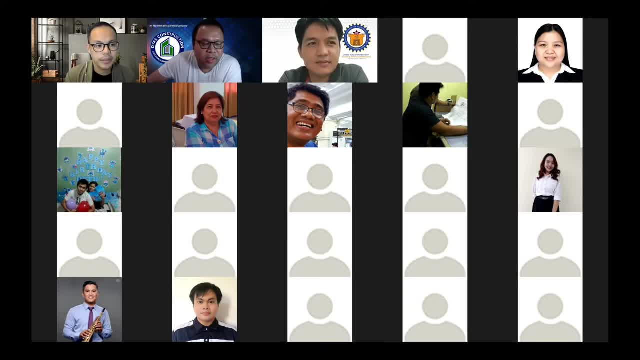 or what we call prolongation claims. Yes, it is claimable. Yes, it is claimable, But you have to take note that the actual cost of the extension it is not based on the amount in the contract period, It is based on the cost of the bond that is stated in the POQ. Say, for example, 100,000.. And then the contract period is 10 months, So there will be 10,000 per month. And say, for example, your contract was: 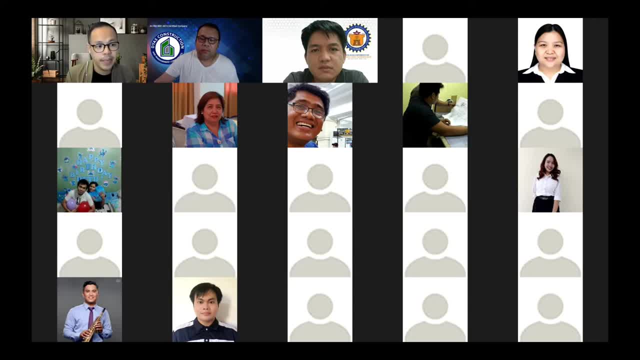 extended for a further three months. You will have to buy the contract to the insurance company or to the broker or the guarantor. Okay, Questions More. Sir, I have a text message. This is for the benefit of the contractors listening here. 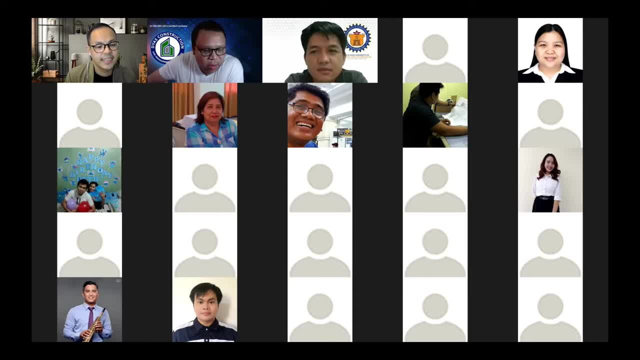 The text says: could you please clarify the request for time extensions? Could you please clarify what are those? Sorry again, sir, I did not get it. For the request of time extension, let's say, for example, of the contractor. what are the reasons or the valid reasons why the contractor is entitled for extension of time? Yes, for the extension of time, But not all extensions of time are. the contractor is compensated on both money and time. There are events say, for example: 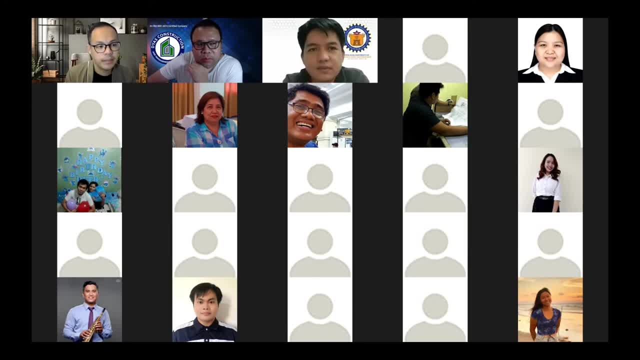 in the contract. you have to be very careful in distinguishing those two And make sure that if you are applying for extension of time, your claim must be within the time bar or within the time limit stipulated in the contract. Say, for example: 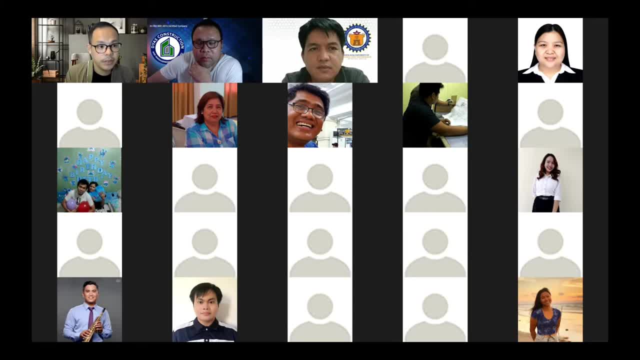 in FIDIC you are required. the claim, regardless of its merits, will not be considered. Okay, For example, for pandemic. you know the COVID-19 pandemic is one reason for the extension of time. right Now, what will? 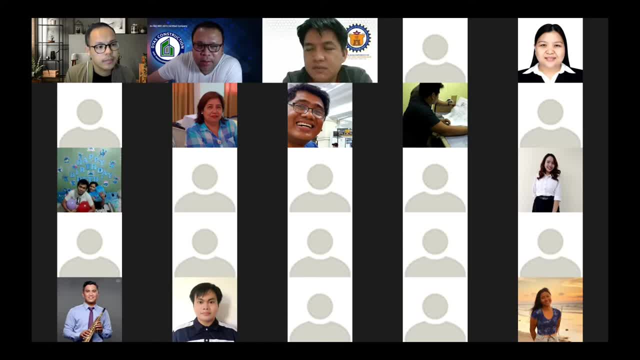 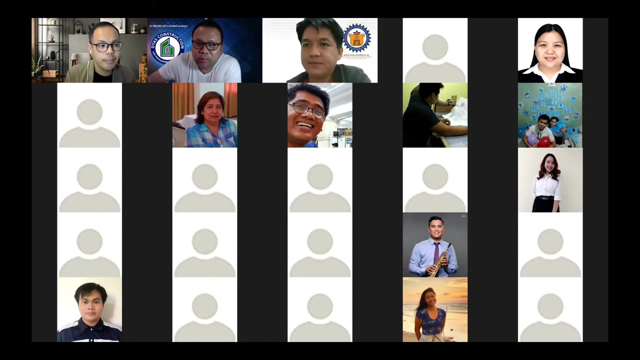 be the basis for the extension of time due to COVID pandemic? What will be the basis? Yeah, So you have to make sure when establishing your legal basis. you have to make sure what are the reasons? what is your legal basis? Are you? 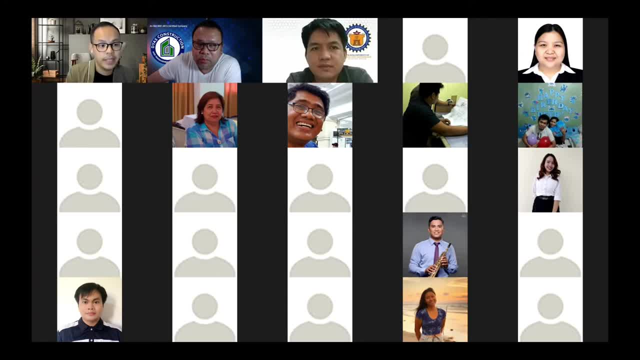 clearly claiming because of the pandemic, For example, movement controls, delay of shipments abroad or disruption, loss of productivity, because before the pandemic it's 10, now it's only 5, because of your compliance to the government instructions which we 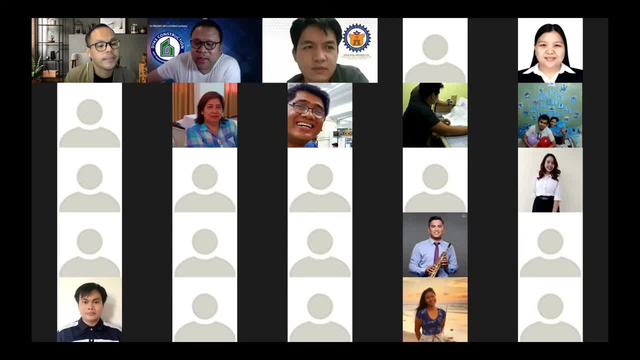 consider legislations or government actions. So you have to be very clear in that. Yes, sir. Okay, There is a question from the chat box. Sir COVID-19 pandemic is considered as force majeure? If yes, since usually force majeure is part of the contract provisions, therefore the costs incurred due to government regulations are budded to claims. 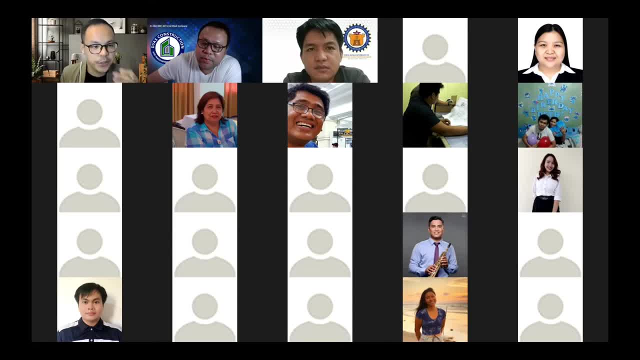 The question is a bit convoluted. So first: yes, this is asking first for the COVID pandemic. Yes, If pandemic, is the pandemic considered a force majeure event? I have advised many clients about this And my decision will. 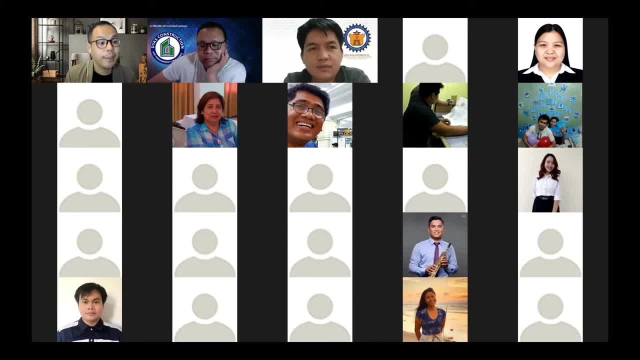 always? my answer to them is always: what is in your contract. So there are certain contracts in the delaying events, There are certain contracts that are written as force majeure. So how will you? and the thing is that when you, when your contract only specifies force majeure, 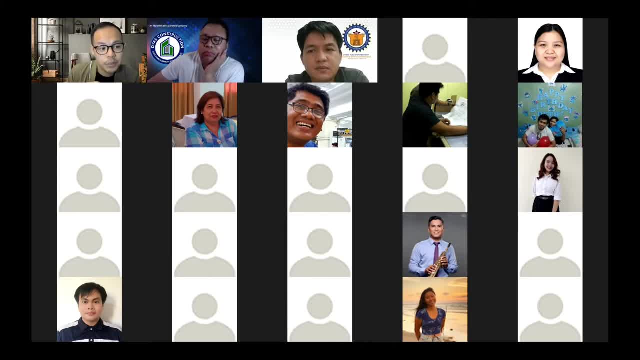 what is force majeure? Then the question will be: what is force majeure? Is pandemic a force majeure? So it will depend, and then your question will evolve or will move on to what is force majeure In China. 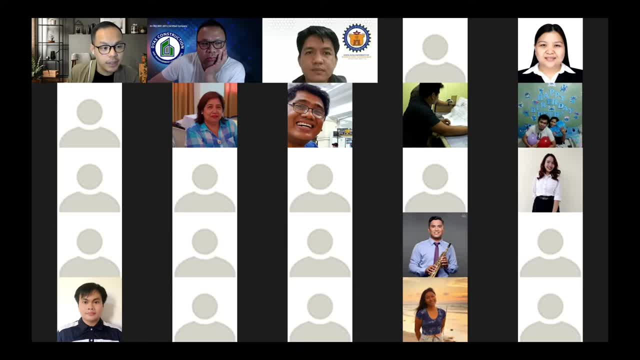 which is a civil law jurisdiction. the government issued a certificate actually saying that the pandemic is force majeure. However, the validity of that certificate is still untested in courts. But luckily most Chinese companies accepted out that certificate. However, outside China, 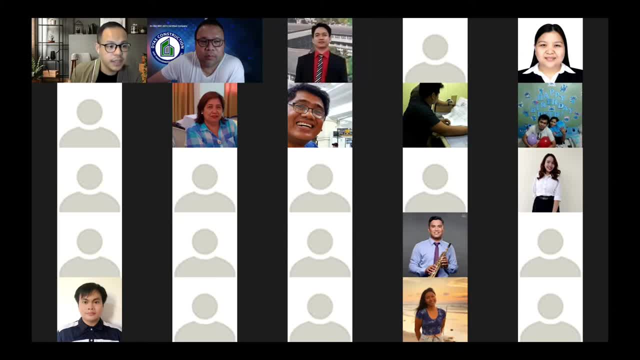 that will be very difficult in the in justifying that the pandemic is force majeure. However, my suggestion is that look at your contract. Is there a written legislation? Is there a written shortage of manpower? Is there a written shortage of materials? 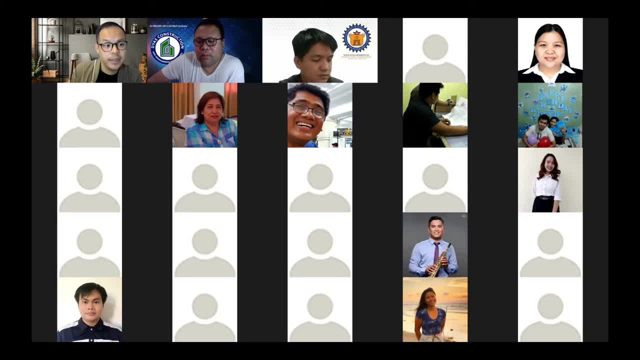 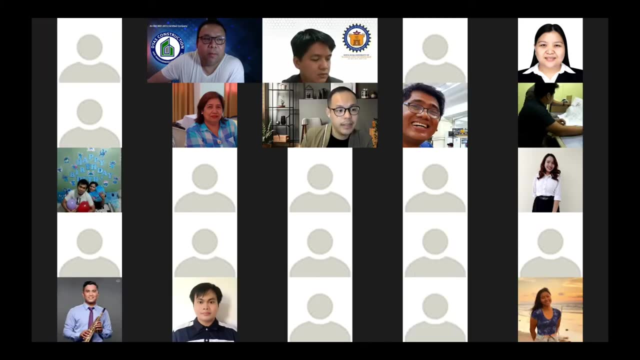 Then if that's the case, then you can claim for extension of time using those events and not the pandemic. But if your contract expressly provides that a delaying event, a pandemic, is a delaying event, then that's fine. You can claim for that. 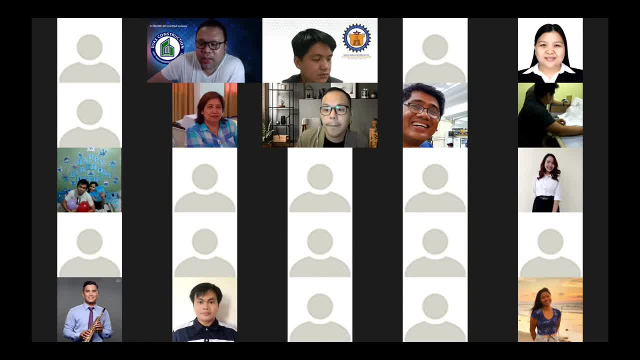 Okay. Next question: It is valid to have a contract that doesn't allow variation order? Okay, As I have said, I have said earlier now, the parties are free to agree on the terms and conditions of the contract. So if, if you are, 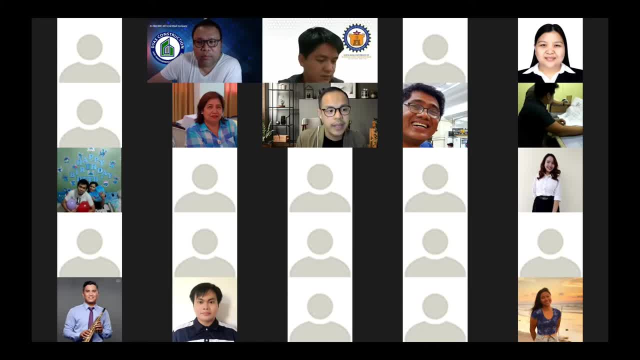 if you are entering into a contract which does not have a variation order, then that's the risk of the contractor. So if the contract does not provide or does not include a variation order clause, then when you need to to vary the work, say for example: 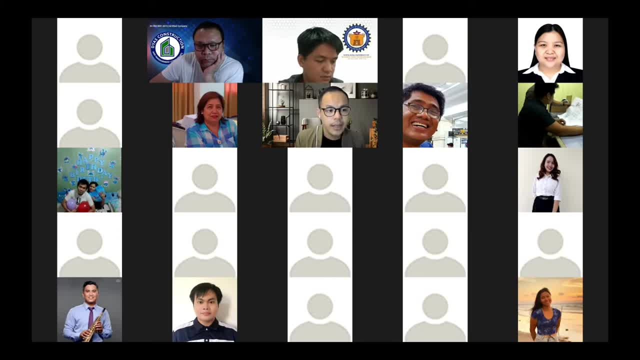 changes in materials or just even changes in quantities, you have to enter into another contract, which will be time consuming because there will be negotiations and then there will be disputes like masyadong mahal, or what will be the basis of the rates, and so on and so forth. 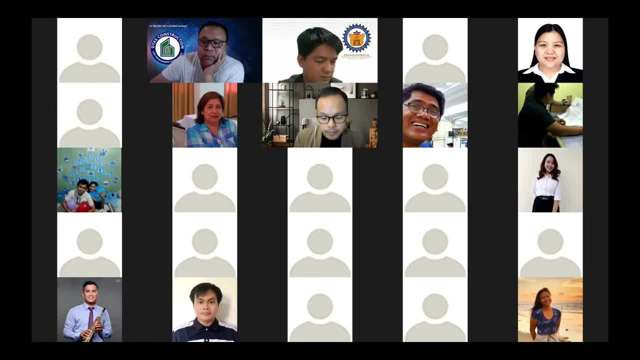 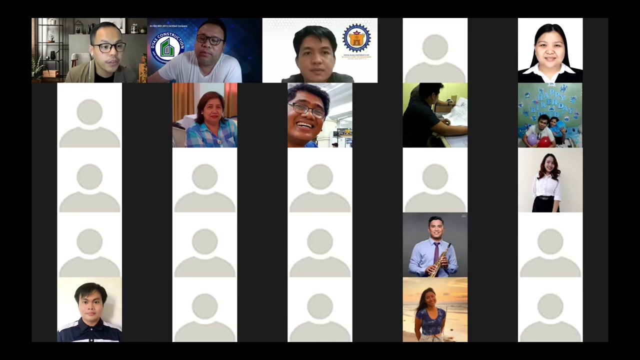 So it is enforceable, but it will be very risky for the contractor to undertake such contract. Okay, Another question: Is the contractor entitled for profits on expenses related to COVID pandemic? So for loss of profit, no, Because we are only considering direct losses. 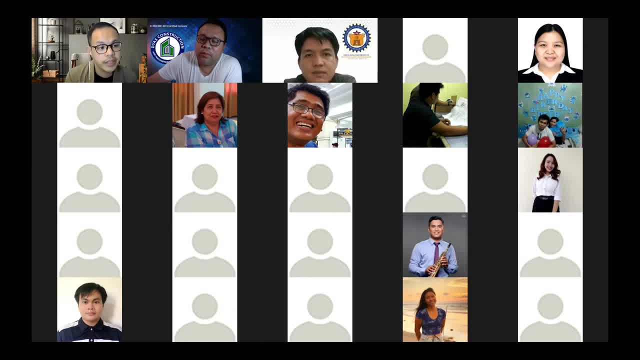 and loss of profit is not a direct loss or direct costs. So usually we just like overheads. These are not- how do I say it? Non-direct costs. So the direct costs are just say, for example, the extension costs for extensions of insurance and bonds. 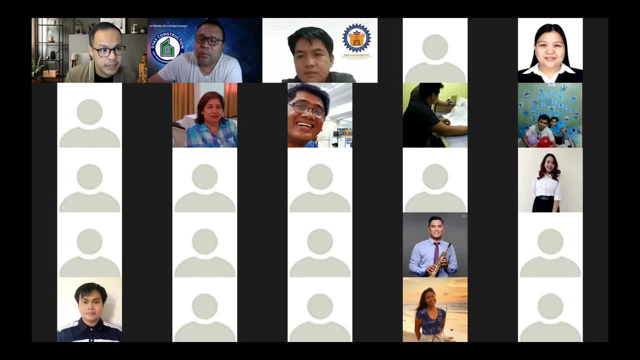 office rentals, site staff, machineries which were idle or stuff like that. But profit, no Profits. profit is considered not a direct loss. Okay, Some more questions. Oh, here is a clarification, a question rather Follow up, sir. 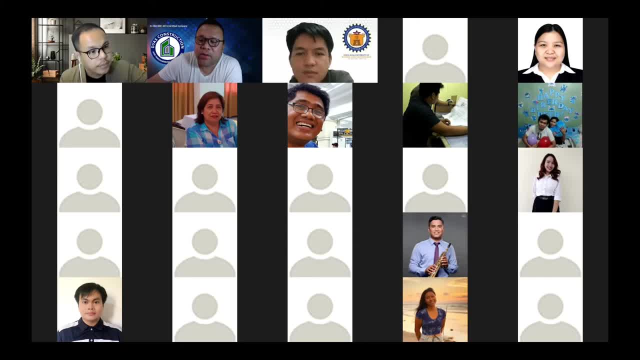 To Ms Cruz. It is claimable if suspension is contractor initiated for the bonds and insurances. What is the reason for the suspension? That is the first question. Is it the suspension because COVID-19 pandemic? And then what is the? and then, 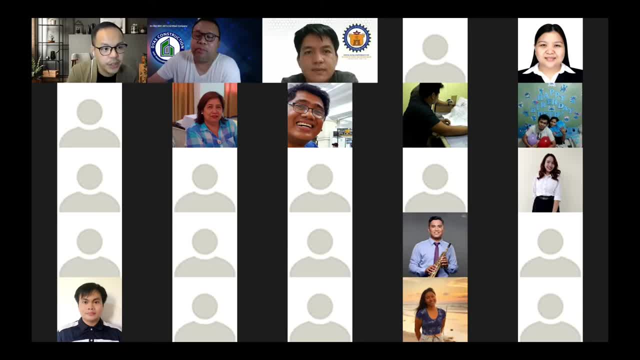 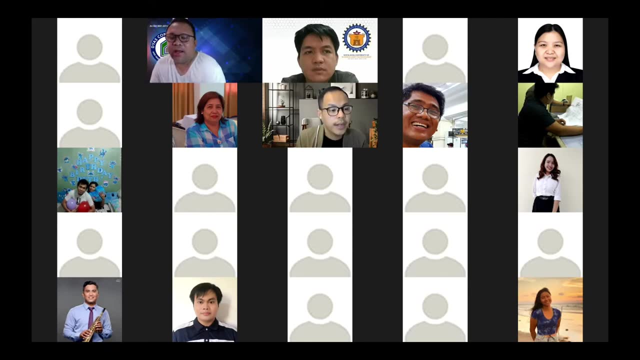 let's go to again the root cause. So what is the legal basis of suspension? Is it because they received an order from the government that they have, or did they? did they out of their own volition? Yes, It says here. it is contractor initiated. 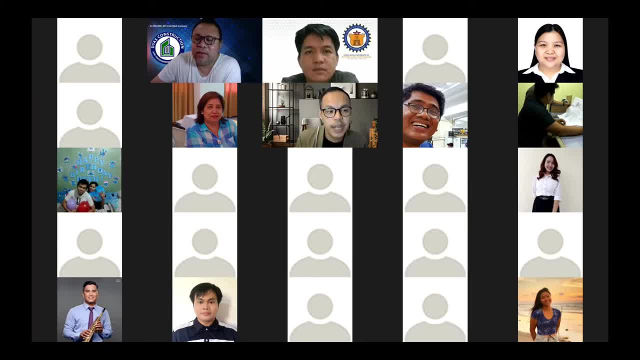 So if it's contractor initiated, what is the motivation? This is important. What is the motivation, Sir? Hello, Good afternoon sir. Yeah, Please, Ms Maisie. Okay, Go ahead. So, sir, what I'm asking? 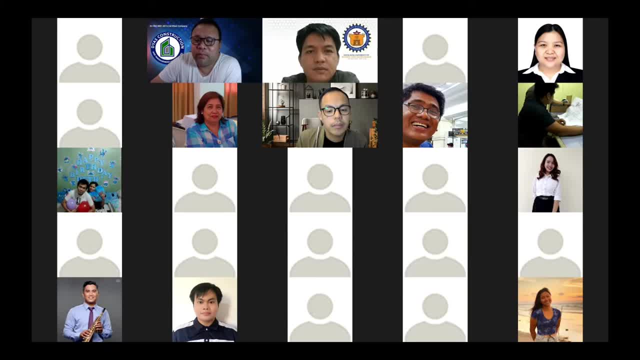 is suspension is because the project was suspended. Then, upon lifting, the contractor claimed claim for security, carry and performance fund. Okay, So it is claimable Because of the, because of the suspension, Suspension And the risk of the, because you said: 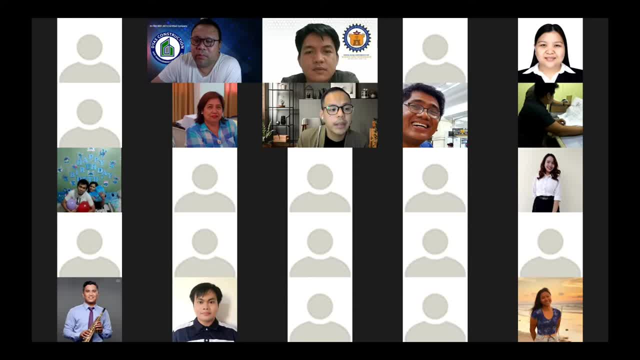 because of the application of the permit, correct, Yes, sir. So they initiated the request of suspension because they couldn't get the permit from the government. Then the employer gave the employer the suspension Due to the request of the contractor. 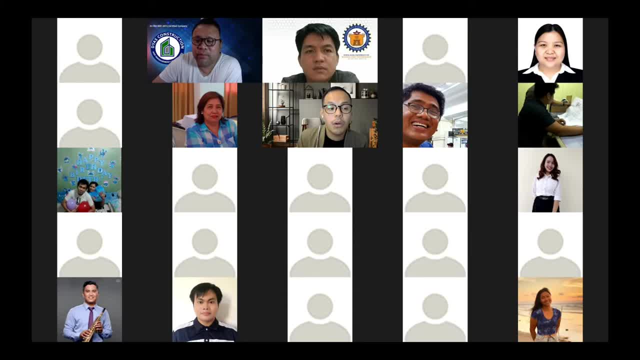 Yes, Oh, What if they? because in FIDIC, if I'm not mistaken, the contractor can notify the insurer or the bonding company if such events will happen or happen. Okay, I'm not sure on that specific provision, but I know. 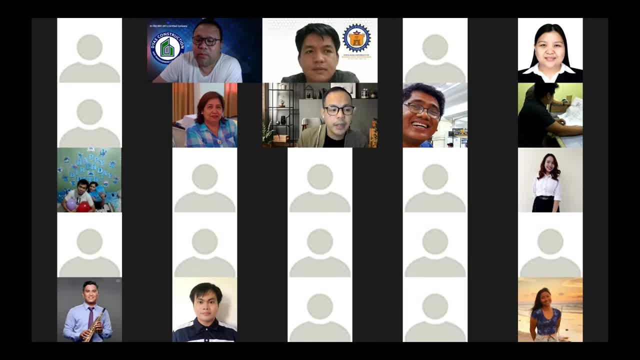 a provision that gives the right to the contractor to suspend the works, But the reasons are also there and they're very limited. So, anyway, I think so is that a question, or it's like you just encountered it on your side, that the issue 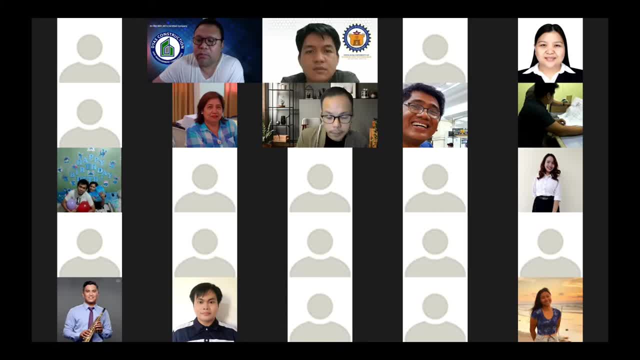 is already settled. So just an insight, sir, if the contractor can claim it, if he initiated the request, Because the main reason or the root cause of the suspension is because of the contractor's failure to get permits correct. No, Actually. 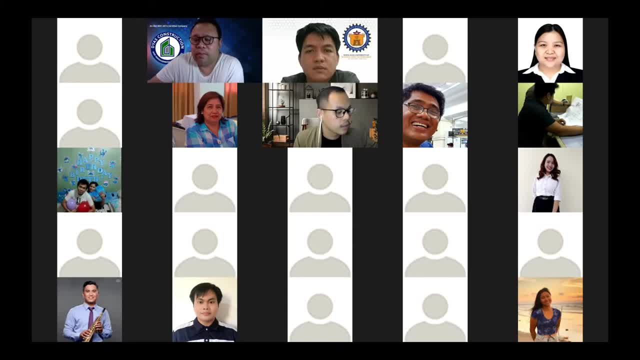 it's not a failure, sir, because he got it but he wasn't able to give it to the concerned agency. Yeah, Sorry. So now we're very a bit the, the, the, the lawyer hat I'm wearing a bit, so I'll ask you now. 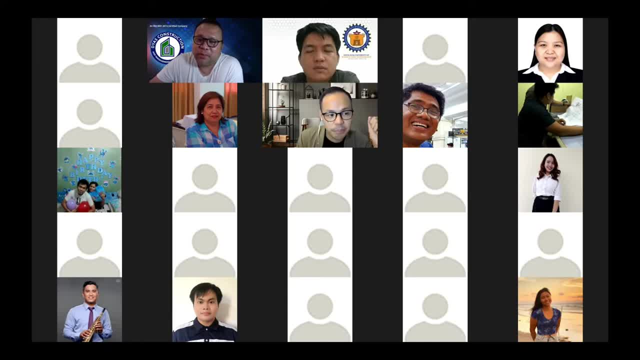 Is there a permit or not? No permit, Then the contractor failed, correct? Yeah, Ah, yeah. So if that's the case, if that's the case, then the contractor is not entitled, because the contractor is at risk, because the contractor 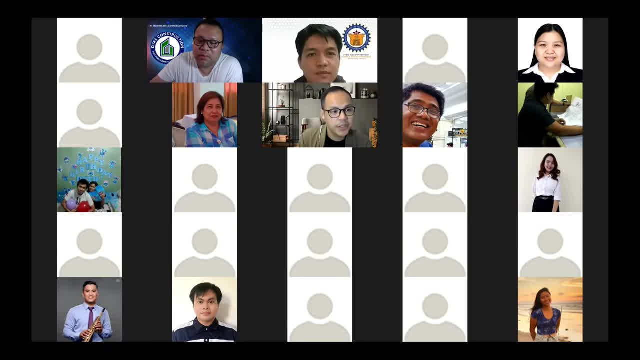 is at risk of the permit acquisition. Okay, sir, But but regardless. if you said because of that, the employer issued the instruction to suspend the works, then you have an argument because you'll say, oh, you're the one who ordered the suspension. 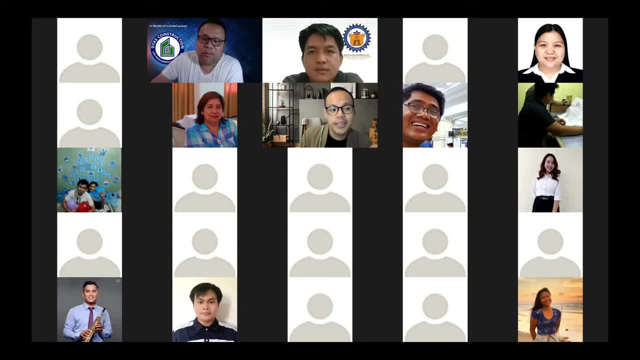 So, regardless if we initiated it or not, you still issued the suspension and suspension, the employer is entitled the contractor for the additional costs incurred. So it's very ah. if you look at it, your scenario is very complicated, but 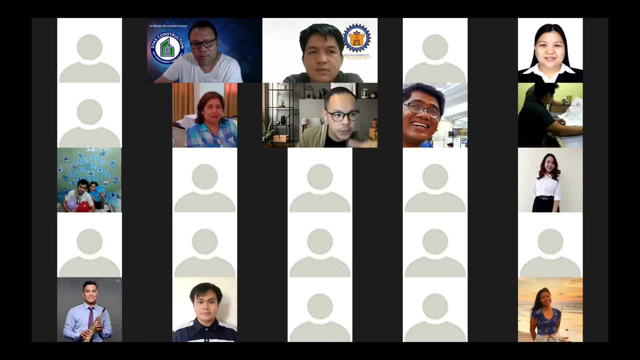 Yes, you deduce it. you deduce it into what is provided in the contract and who is really at risk. So you can argue on that, on that, on that point. But but then that's not an advice. 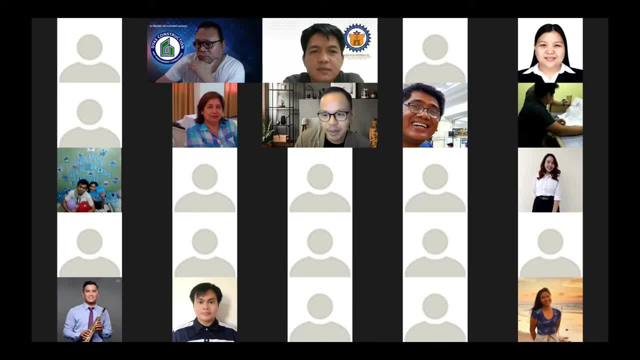 just an opinion. So if you did that and then maybe you sue me for for your losses because you complied or you followed my advice, That's just an opinion, Okay, Okay. So thank you so much, Don't quote me on that. 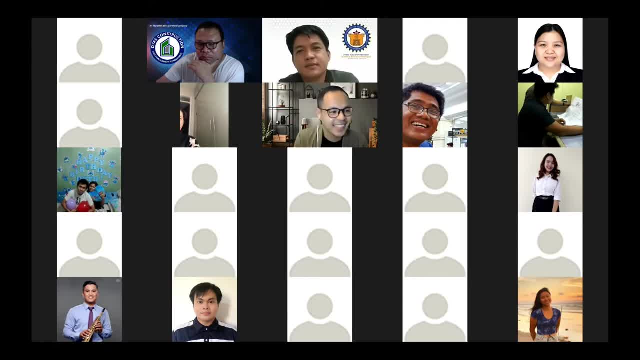 All right, Don't quote me on that. Here's another text, JC. It says that the contractor, for example, he likes to claim for an extension of time, but the reason is due to supplier's delay. third party supplier's delay of the materials. 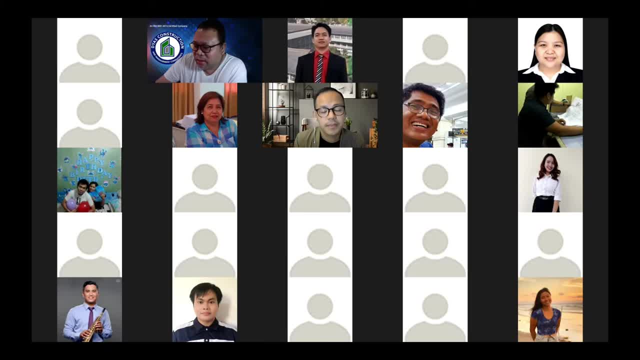 Can the contractor claim it to the proponent as a reason for extension of time. So si contractor meron siyang contract with the employer, correct? Yes, Si contractor. employer may claim as a reason for extension of time. So si contractor 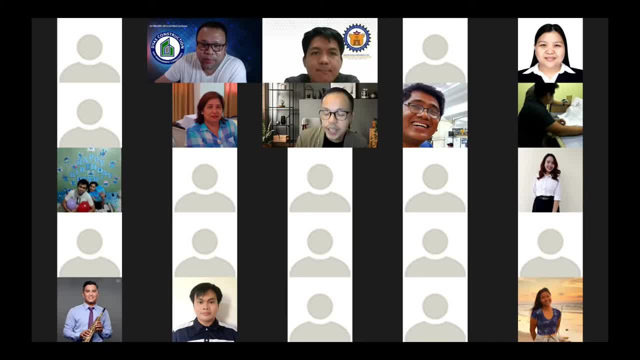 meron siyang contract or employed another subcontractor for the supplier of the materials. Actually, the supplier materials will be by the contractor, but he has the supplier to supply to him. Yes, Yeah. So again, we will be employing the privity of. 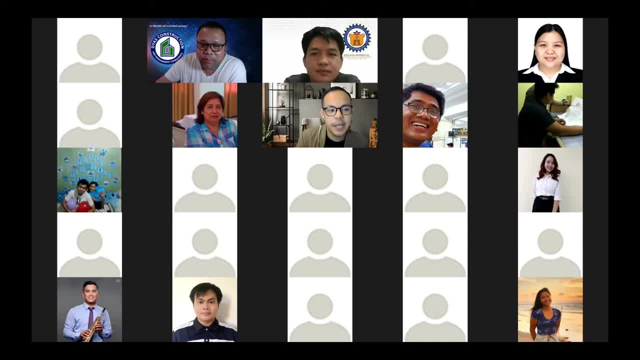 the privity of contracts. Walang kinalaman si employer dun sa mga subcontracts mo. So once ang liability mo kasi kay employer is to deliver the materials and to complete the works. Ngayon, when you employ a subcontractor, 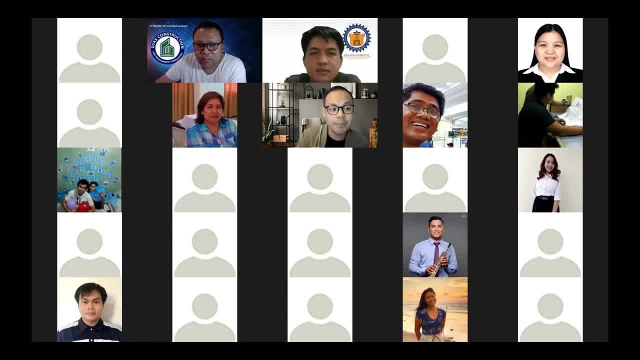 who will supply your materials or your goods. that becomes your risk. So if na-delay ka, if na-delay ka because of that subcontractor, wala nang sorry for the lack of a better term, pero wala nang pakialam dun yung. 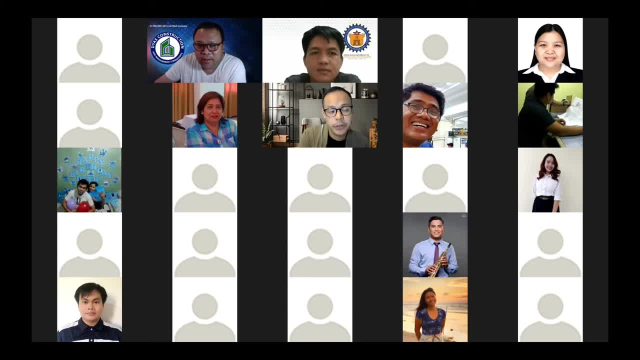 employer. Yeah, correct Yung employer, kasi it's between you and your subcontractor. So for the employer titignan lang niya: ano ba yung liability mo sakin? Ang isang way na pwedeng i-resolve. 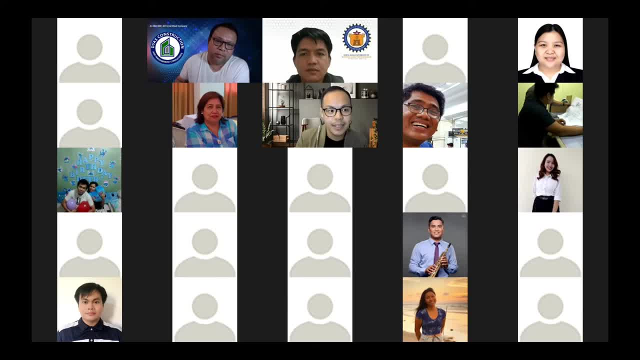 those kind of issues is to pass the risk ni main contractor, ni subcontractor niya Kailangan meron ka ding liquidity damages clause. Okay, Para just in case, ma-recover yung liquidity damages sayo, ire-recover mo lang din. 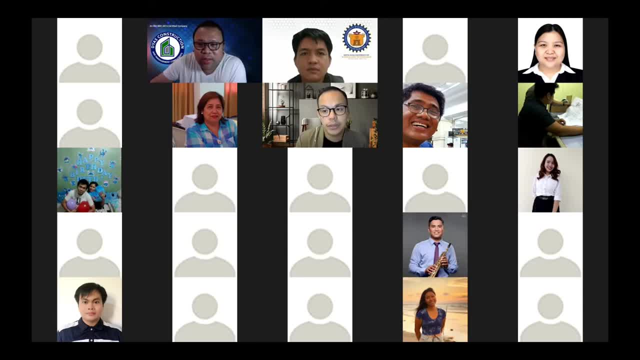 yung kay client, So wala kang laws, Yeah. He further mentioned that the reason of the supplier's delay is due to COVID-19 pandemic. That would be a reason for the extension. Regardless, Again, regardless. So the contractor. 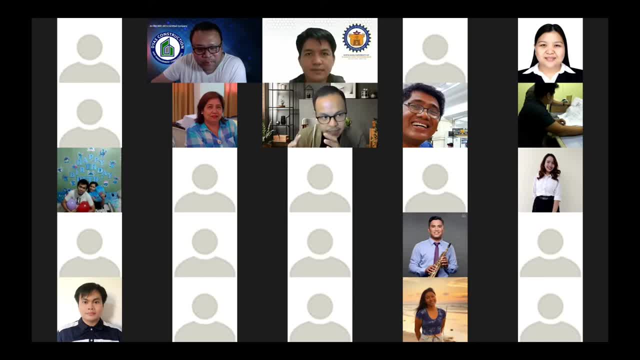 the contractor's agreement atsaka yung subcontractor's agreement niya. It's a separate agreement from the main agreement itself. So ang solution to that is tignan niya yung terms and conditions mo with your subcontractor And from there. 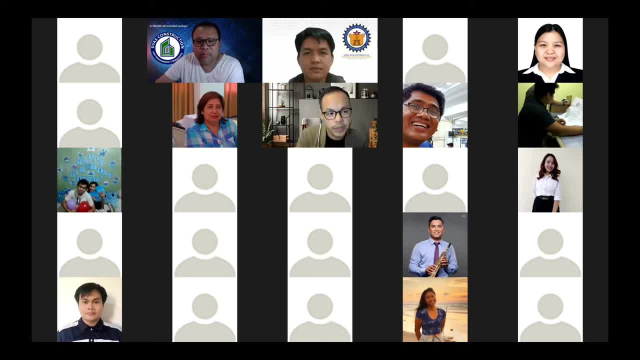 titignan mo ngayon yung terms and conditions mo with the main contract and the employer, Kung paano mo ma-me-mitigate or ma- ma-ayos yung para ma-minimize yung loss mo. So 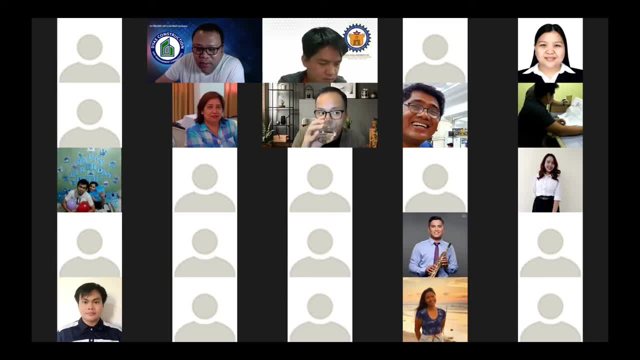 Yeah, Agree, Any questions? Any questions? Unmute your speaker and speak for some clarifications. I guess may mga contractor tayo dyan: No Pwede di ano, ah, Pwede tayo mag-Tagalog, Naintindihan naman. 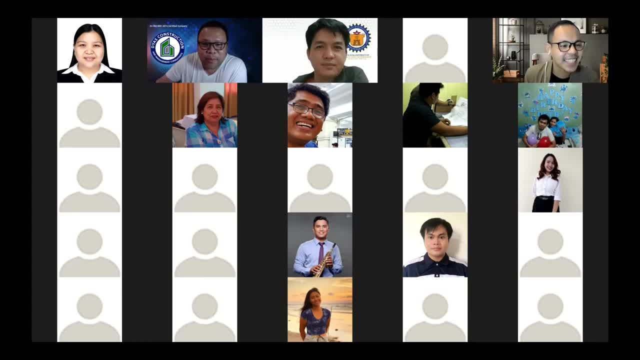 ng JC. yan, Yes, Tess, Hi, Hi, sir, Magtatanong lang po ako regarding dun sa ano: What if yung contractor failed to give notice of claim, say about time or variation, within the specified time ng contract? Okay lang ba na. 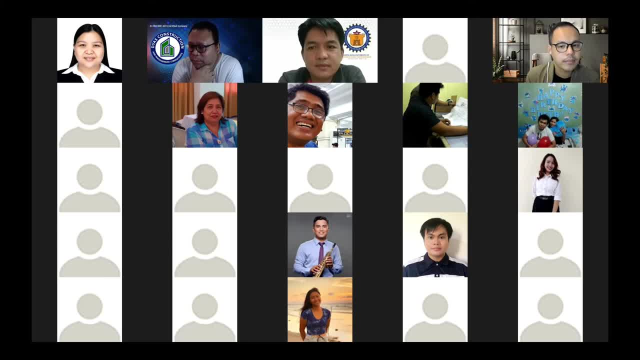 I mean outright denial na ba ng claim yun ng entitlement niya. Okay, Very good. Okay Yun yung question Apo. Alright. So in a common law jurisdiction say, for example in: as I have said, bigyan kayo ng perspective. 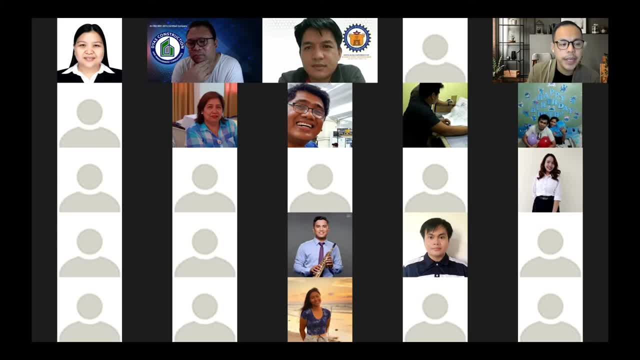 on the difference of the two jurisdictions. no, In a common law jurisdiction, say, for example, in Singapore, UK, Australia, Canada, it is an outright decline, Meaning regardless of the merits, regardless of the merits of the case, kapag hindi mo na. 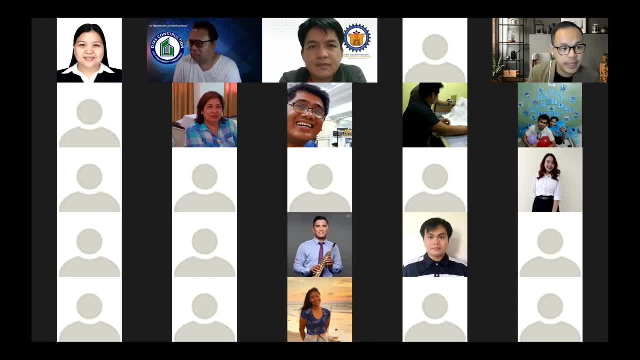 comply yung time bars. for example, you have to submit it in 14 days. Sinabit mo siyang on the 15th day. hindi na pwede yun. Your claim has been forfeited, Okay. However, in a civil law, 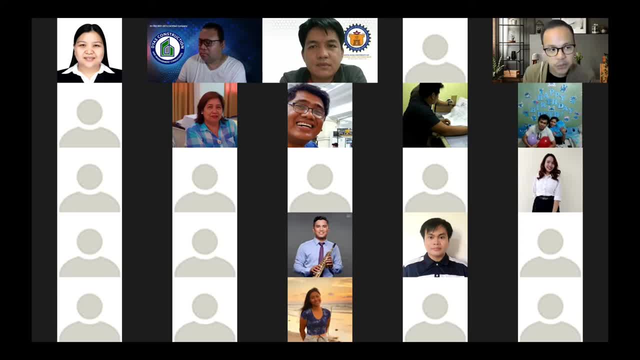 jurisdiction such as the Philippines actually may sinusulat ako regarding this issue. In the Philippines, ang argument kasi dyan is: it is unfair Di ba? The same principle applies sa liquidated damages Kapag ang clause, ang contractual clause. 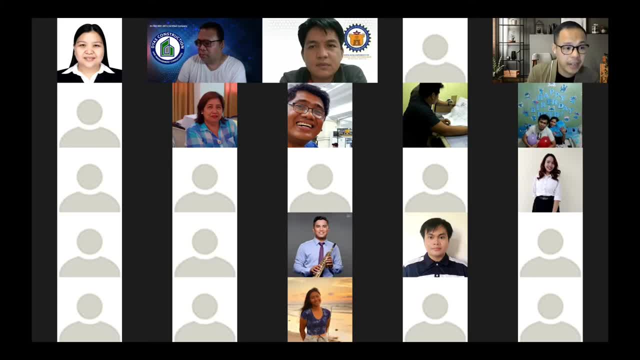 is unfair. is unfair pwedeng pumastok si court or si arbitral tribuna to decide whether whether to allow or not to allow the claim. So in a civil law jurisdiction, pwede mong i- i-argue on that point na? 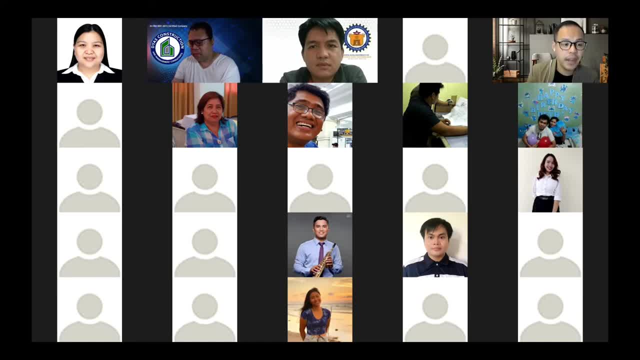 it's unfair kasi, whether to allow or not, We're working from home. wala kaming staff and stuff like that. So pwede mong i-argue yun sa court In a in a civil law jurisdiction? pwede mong? 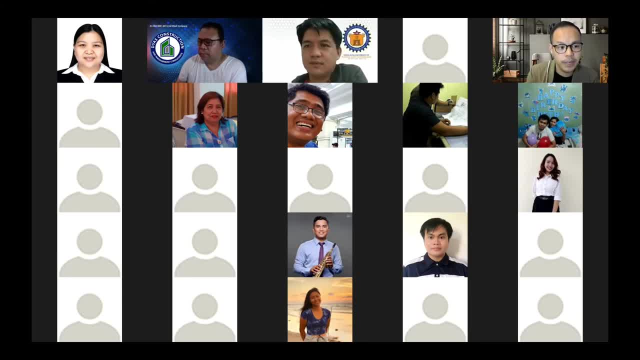 it's still arguable. Meron ka pang, meron ka pang so-called ray of light, na chance for that claim to be considered. Pero in a common law jurisdiction that is an outright no Kasi very strict sila, sa very strict sila. 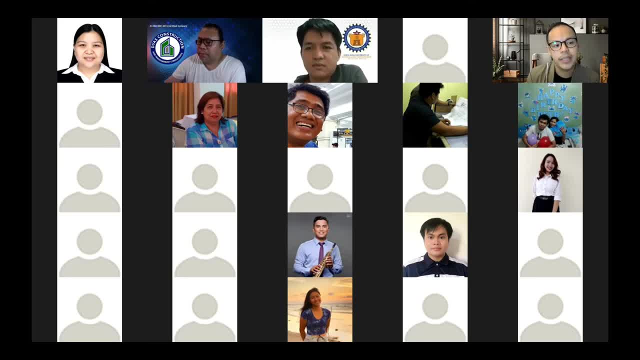 sa performance or sa time bars? Sir, follow-up question lang ulit. May same case kasi ko, kaya ako siya natanong: Hindi ba parang nagko-conflict yung mga technical requirements as to the contract versus dun sa? 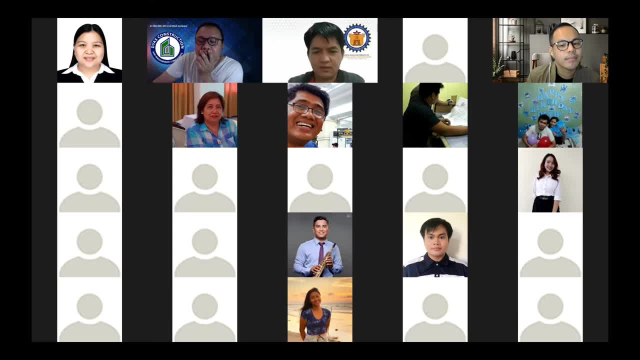 legal requirement, Kasi we had the same case na ano po nag-fail ng notification si contractor sa amin, So outright dininay namin dahil nga doon sa technicalities, Parang say about a year bago siya nagsabi na magkiklaim siya. 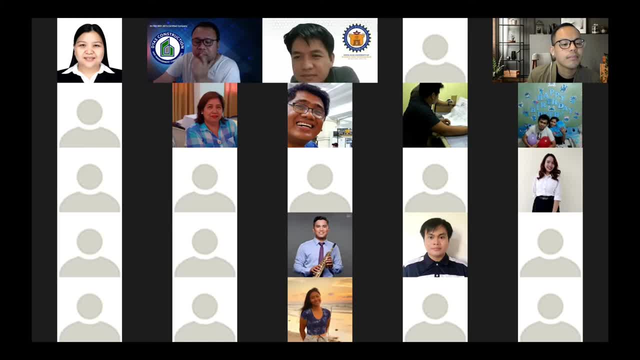 But then again, nung nakarating kami sa legal point of view, lumalabas, dahil nga meron kami inspector on-site, Noon sa inspector yung nangyari on-site, So parang doon tinignan ni legal na. 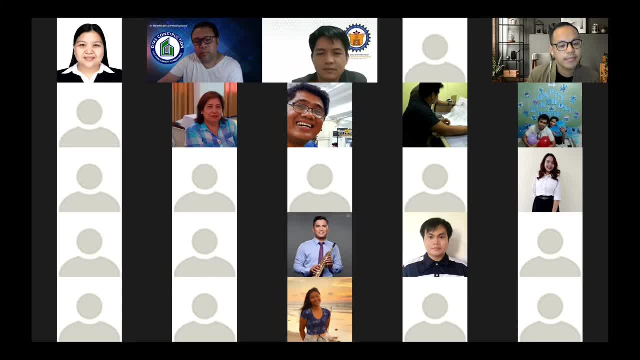 na kung may notice o wala the fact na aware yung yung representative na employer dun sa nangyaring variations on-site, ibig sabihin parang tinatanggap mo siya na claimable dahil wala kang binigay na notice. 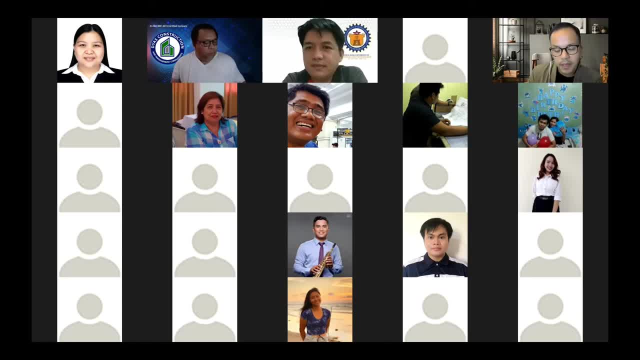 na kinokontest mo yung ginagawa on-site. Parang ganun po yung nangyari. Silence is not consent. So regardless kung sabihan kita na gawin mo to or regardless kung alam kong nadelay ka. 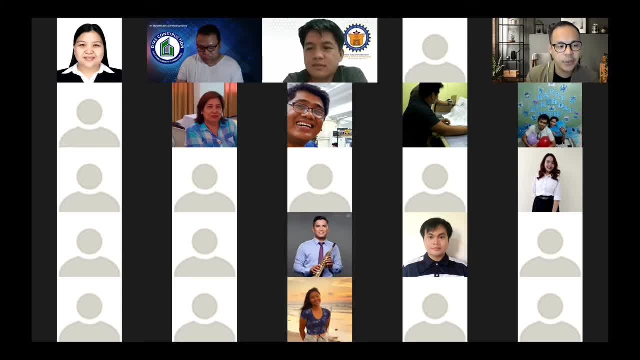 kung wala kang notice, kung wala kang, kung wala, kung ang provision sa contract is kailangan mo kong inotify, Tapos wala kang binigay na notification sa akin, Then what sense is the contract? 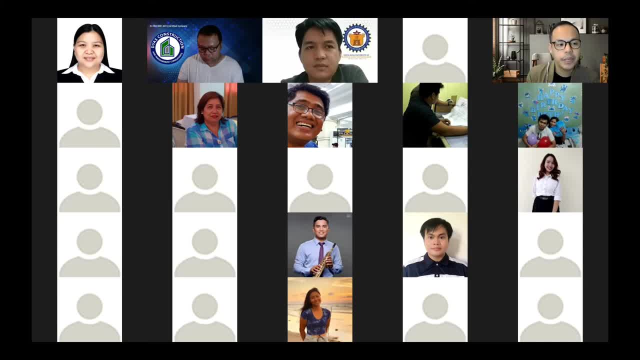 Get what I mean, Kung, if you'll take it as a common knowledge. So I think the gist, or what I'm just trying to say here, is that you have to comply with the terms of your contract. Hindi porke alam ni contractor. 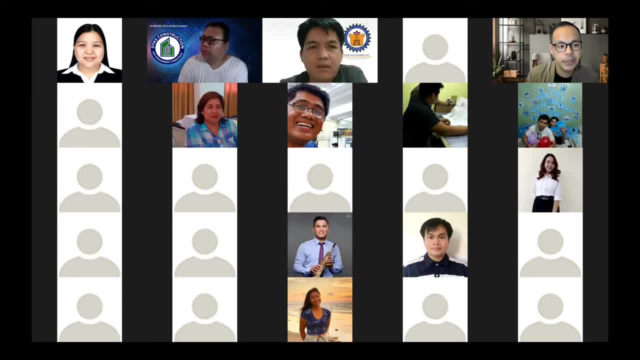 or hindi. porke alam ni employer na yung delaying event is aware siya doon sa delaying event and that might cause you, that might cause you delay. You still have to send a notification, Kasi paano niya malalaman na makiklaim ka pala. 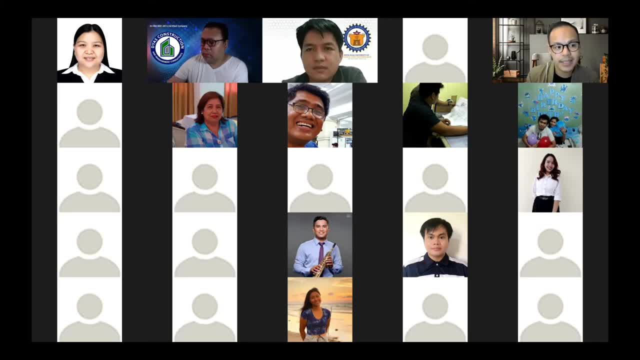 Paano niya ma-allocate yung funds niya, Paano niya ma-allocate yung risks niya. So kaya a notice is very, very important And, as much as possible, you have to follow what is your contract terms. 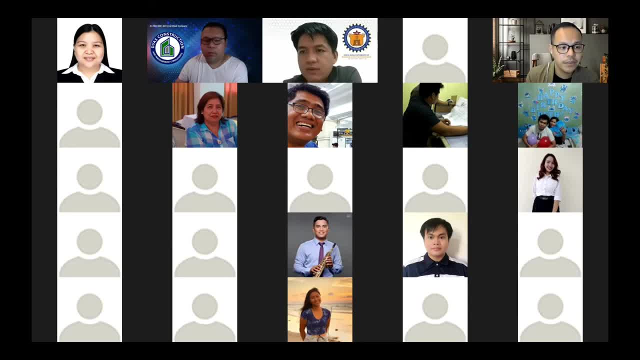 But again, if nag-succeed naman yung claim ninyo for that, then that's good. I'm always for amicable settlement and the resolution of dispute, So if at the end of the day it was allowed, then that's better. Okay, sir. 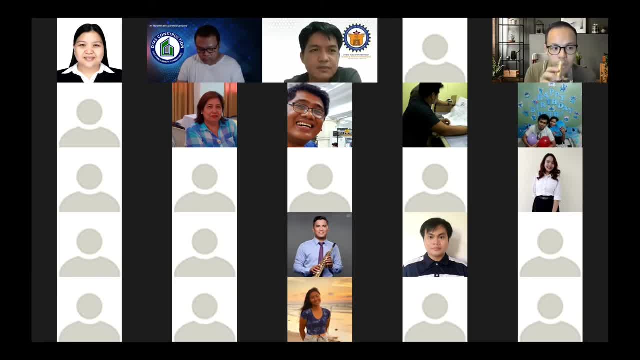 Actually nag-add na yung issue. ang nangyari nga is ano amicable settlement. siya Ang nangyari. pero ang nangyari nga nakapag-claim siya, Although walang notice. That's good for you. 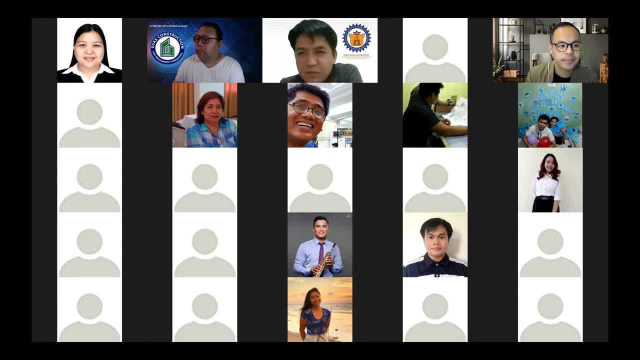 Thank you, po. Okay, Okay, thank you, Ma'am Marites. Yes, Sir Jaycee. another question here from Sir Raymundo. So if the contractor suffers delay due to the restrictions set by authorities, like limited working time for public convenience, 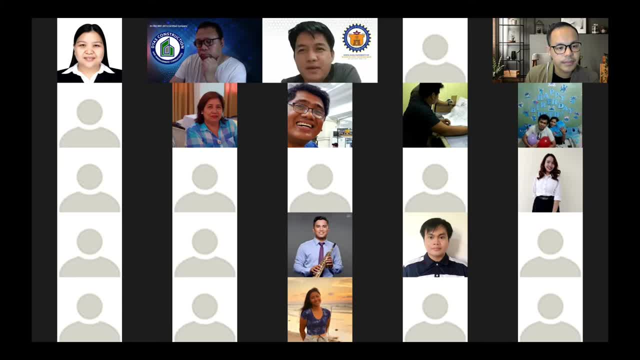 is the contractor entitled to post-claim? I think, in terms of costs I would have to look at the contract first, But as a rule of thumb, kapag hindi si employer yung naging cost ng delay, then walang claim for cost or walang entitlement to cost. 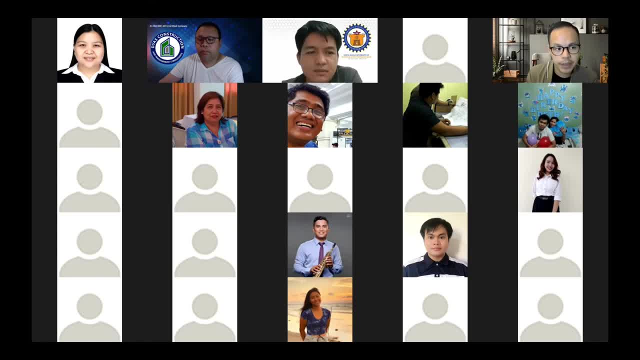 si contractor time lang Pag neutral yung event. I think this is a good guidance: Kapag neutral yung event, meaning hindi kasalanan ng either ng contractor or ng client, ang entitlement mo will be just time. Pero say, for example, ang delay mo is: 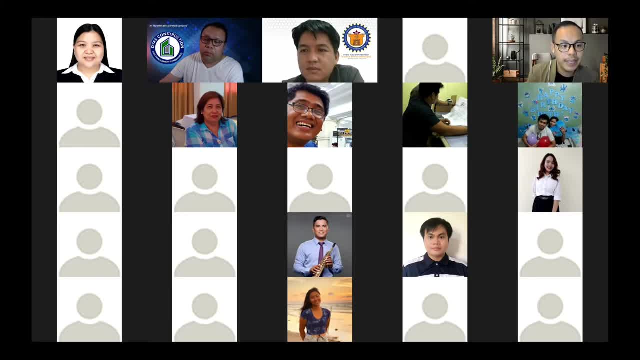 cost by the employer, then you will be compensated or they will give you time plus cost Yun yung, I think, magandang guidance doon, Okay, sir. So another question from Christine Ann Abarca. So our government issued an order on what are the things? 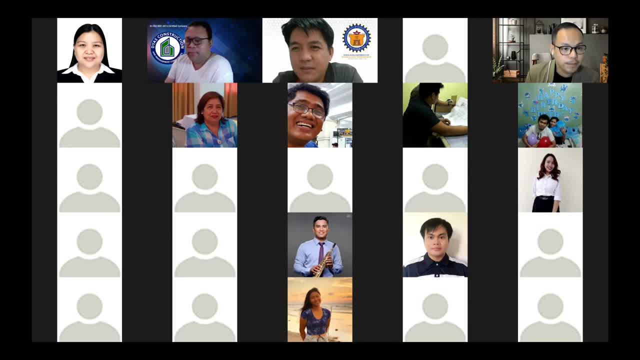 the employer should shoulder as a result of the pandemic. What if the government does not explicitly mention that the employer should pay for the extension of bonds and insurances as a result of the pandemic? Then is it really claimable under prolongation whether it is the contractor's? 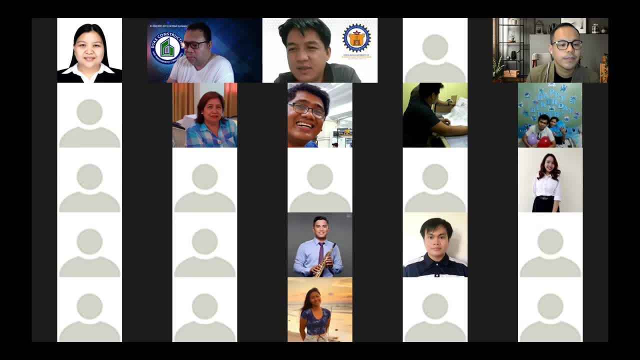 responsibility to provide bonds and insurances under the contract. However, the government issued lockdowns which affected the work, hence the extension. So our consultant used that argument. That is why I want to clarify. So again from Christine Ann Abarca, Sir Daisy. 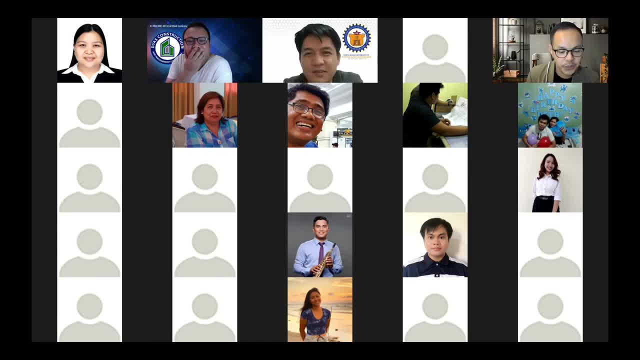 Okay, Medyo mahaba yung tanong. So sabi niya our government issued an order on what are the things that the employer should shoulder as a result of the pandemic Correct. So that is very clear. Kapag nag-issue ng order yung government 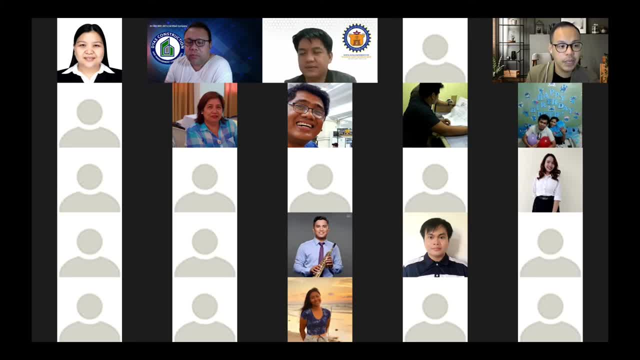 you have to comply regardless of what is the stipulation in your contract, Because, again, the governing law always supersedes the contract. And then the second part is: what if the government does not explicitly mention that the employer should pay for the extension of bonds? 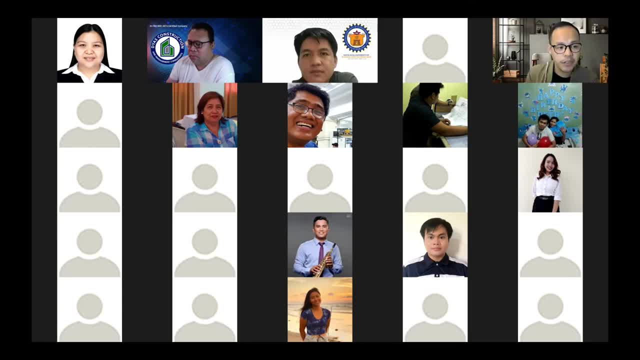 and insurances as a result of the pandemic. So if the government did not issue an order, then you look at your contract. Ano ba yung entitlement sa contract? So that's why you will go back to your terms and conditions. And then another question is: 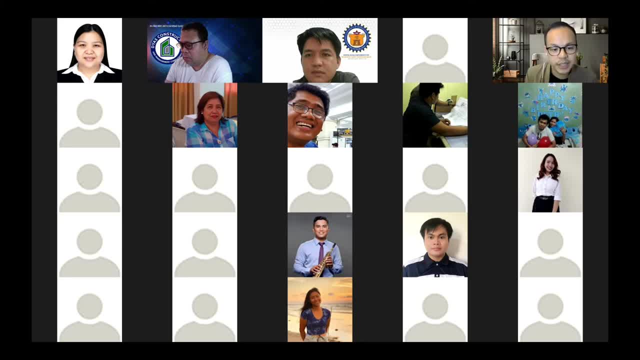 is it really claimable under prolongation when it is the contractor's responsibility to provide bonds and insurances under the contract? Ito yung sinasabi ko, kanina, na sino ba yung nag-cause ng delay. So say, for example: 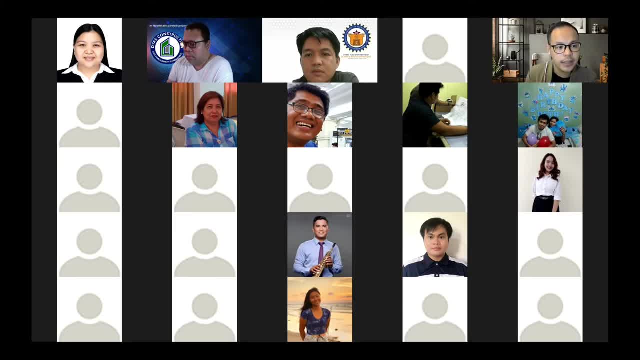 if the contractor causes the delay, then of course logically the contractor should bear the costs for the extensions of such insurances. Pero if the employer is the cause of the delay, then the employer should bear the costs arising out of that delay. Pero what if neutral yung event? 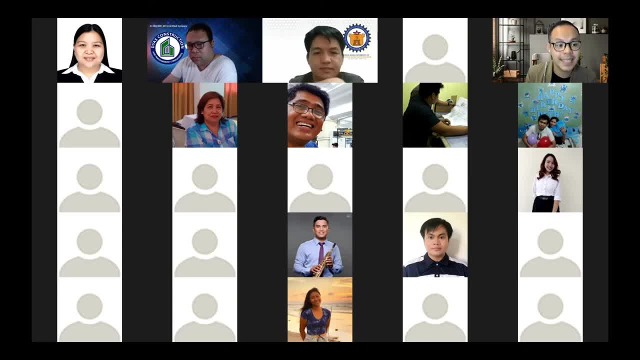 say, for example, this government issue, So that is the risk of the contractor. So unfortunately hindi siya entitled si contractor. hindi siya entitled for that because, again sabi mo nga, it is the contractor's responsibility under the contract to procure such insurances and bonds. 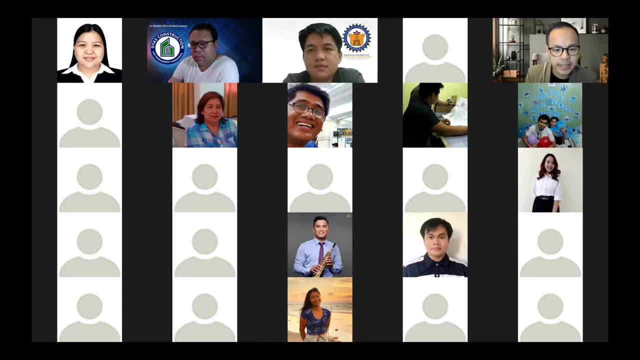 And then, I think, however, the government-issued lockdowns which affected the work. I think that answers the bulk of the question. Okay, Sir, another clarification: How many times can a contractor be given a time extension for Their single or ongoing contract? 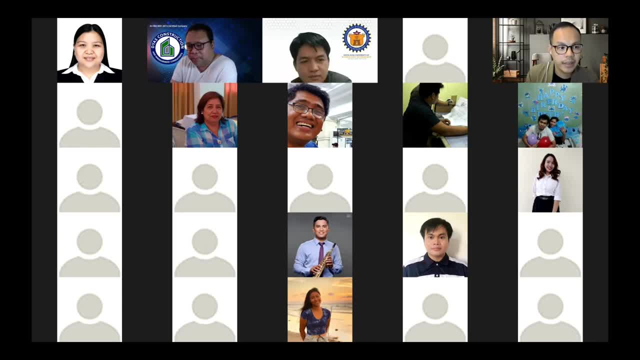 So long as there is an event that entitles the contractor to extension of time, then they can claim As many as they can, So long as ayoko sabihin as many as they can, but so long as an event occurs that entitles them for extension of time. 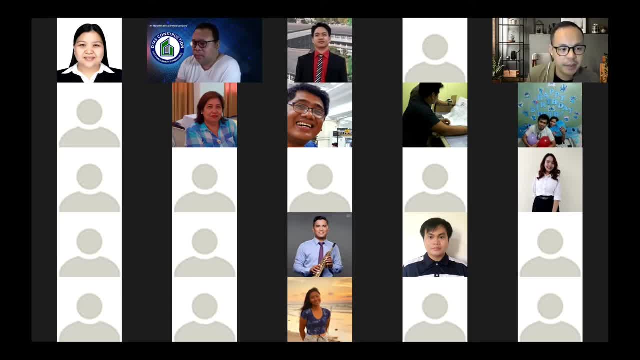 Okay, And, of course, within the time bars. Yeah, correct, Okay, Any questions? Oh, clarifications, Clarify na Hi. Hi. sir Jaycee, May I have a question? Yes, Sir, may I ask? 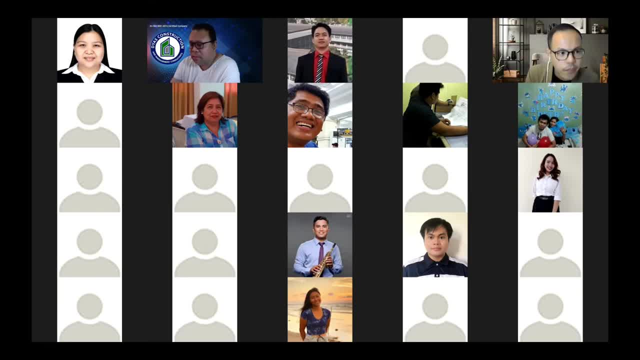 Sir, may I ask, May I ask? May I ask Sir, may I ask? May I ask Sir, may I ask Sir, may I ask Sir, may I ask? May I ask? Then, after a few months, sir, we had a claim that we had an extension of time due to revision. 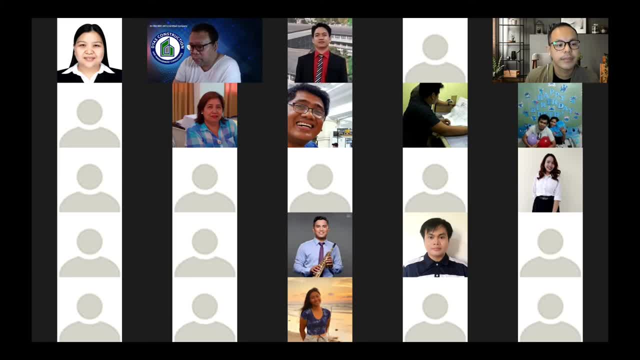 So now, sir, the first justification, the delay that we're talking about, is we can still catch up. I think, na-cut off si Marnie Wala, si Marnie, Marnie, Marnie, Marnie. 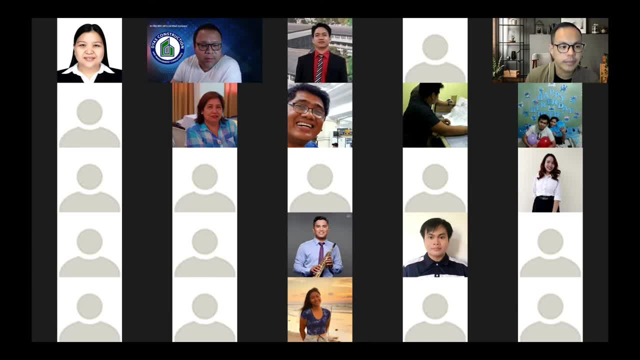 Hello, Marnie, Wala siya, Very interesting yung point. I would just like to say very interesting yung point niya. Kasi kanina sinabi sa slides: no Ang isang title, isang isang. 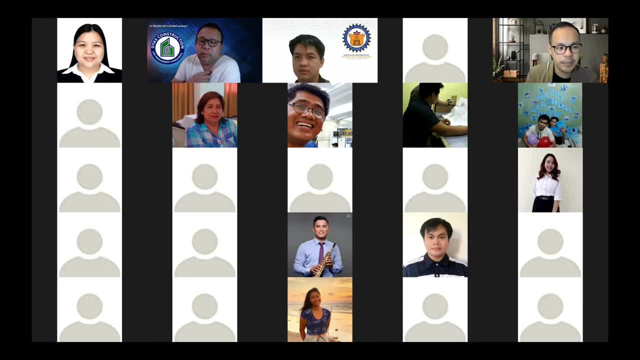 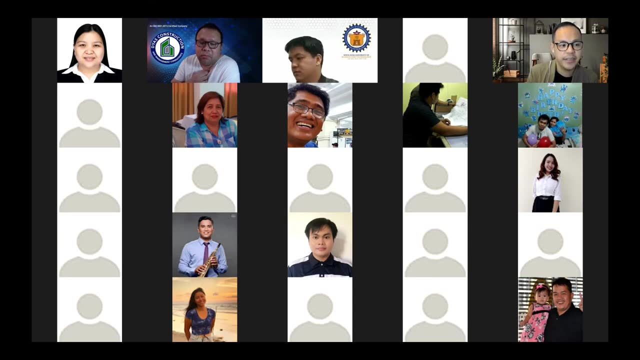 isang. So yung sinasabi niya kanina, kasi sabi niya, siguro sabihin niya sana sinabi namin na we can still mitigate, kaya pa namin habulin, but after that realize namin ay hindi pala. 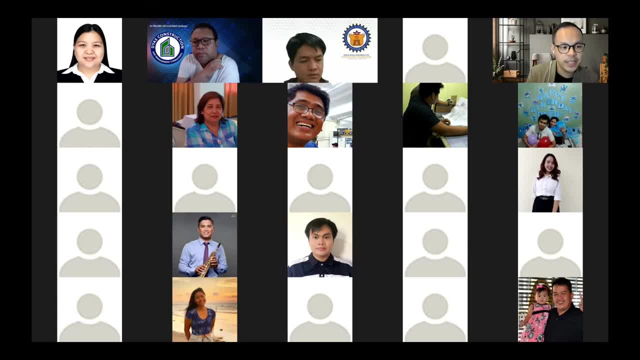 That is where the notices come in. Pwede mo sabihin dun na okay, merong delay event ha, pero we will try to. we will try to mitigate. However, we will reserve our right in the event na, sa totoong buhay, eh madelay kami. 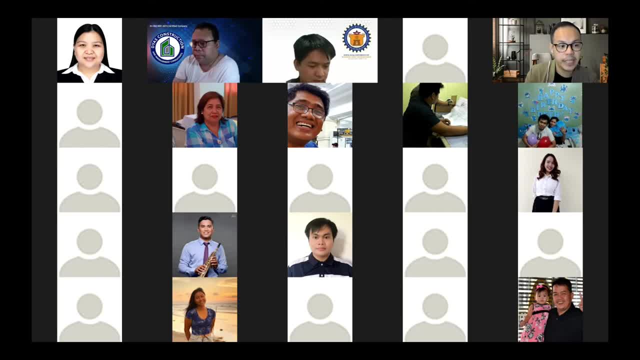 Then we will reserve our rights to claim for extension of time. That will not only say: preserve your right for extension of time. mahihit mo pa yung target mo with the time bar na nanotify mo siya. So I hope. 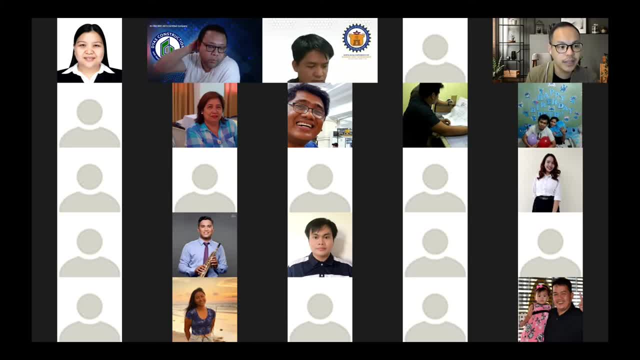 na nakapag-submit. sila ng notice for that Sure. Okay. So, Sir, do you feel nabasa na po ba itong kay follow-up question niya? Yes, sir, Follow-up mo, sir. Okay na sir. 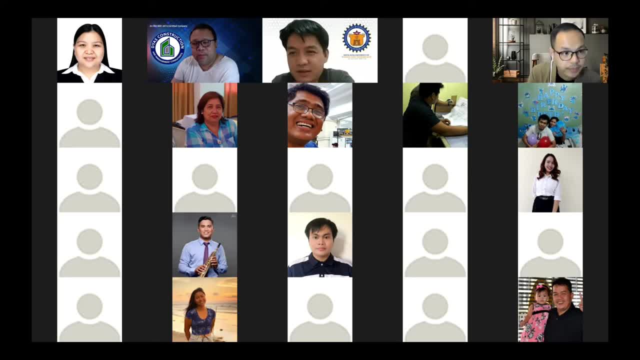 Okay, sir Tanong natin. Okay, So, Sir JC, another question. Okay, Another question. so what if there is a clause that says the consultant cannot claim for additional fees due to the time extensions? however, due to the unforeseen effects of COVID-19 pandemic, they are now claiming prolongation cost. considering that the pandemic is considered an abnormal condition, is their claim valid? 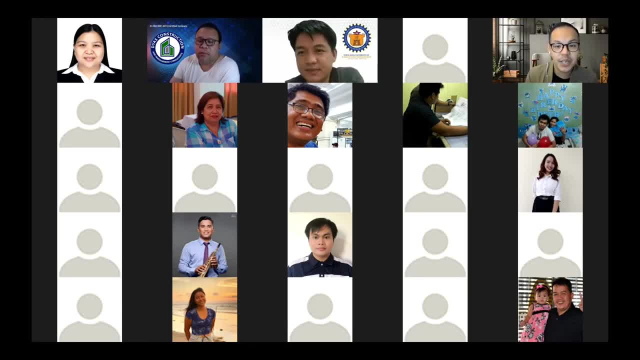 What is ano yung nakasulat sa kontra? Sorry, Melio, Kasi ganoon pa natin yung sagot. what is? what is what is provided for in the contract? Sabi cannot claim for the additional fees due to time extension. 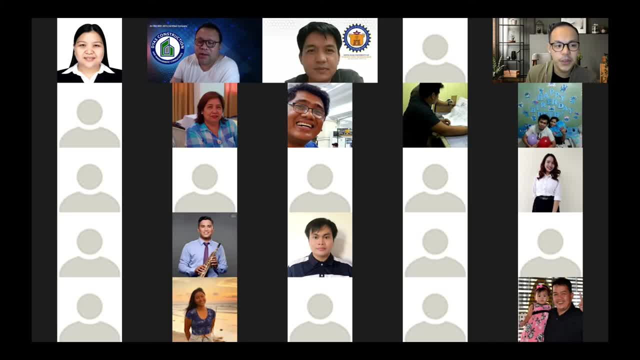 Yun ang sabi ng clause. Usually kasi consultancy fees are lump sum fees. So and if they have, if they have a clause, say, for example, na cannot claim Yeah Like say, for example, lump sum pero may contract period is. 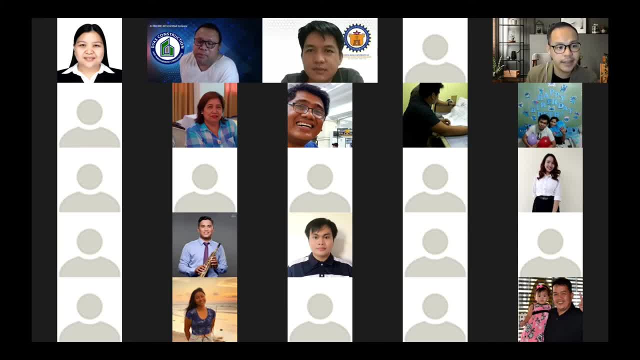 say, for example, 12 months. So then, if it exceeds 12 months and then the contract says no, parang meron din silang claim for extension of time. just in case, just in case, ma-extend yung contract. 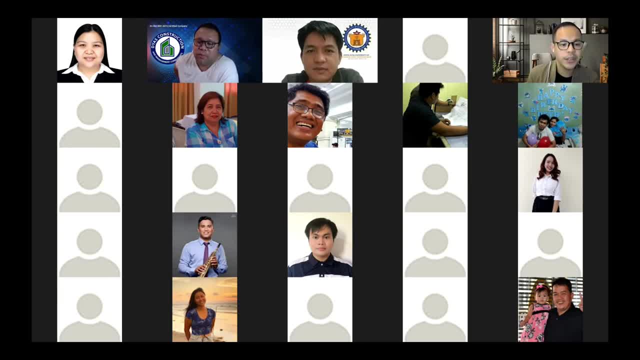 then they can claim, Otherwise they have to establish first yung legal basis. Sir, parang merong pasunod dito. So their contract is coterminous with the BNB contract. po, Ah, Christine, Christine. 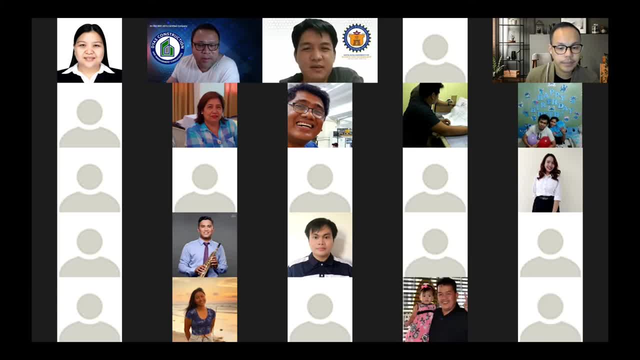 Christine. Hello, Christine, Hello sir. Ah, yeah, Eh tanong, ikaw na magtanong. Opo, Yung contract nila is coterminous dun sa contract Yung supervised po nila Ang initial talagang agreement at yung nasa kontrata is. 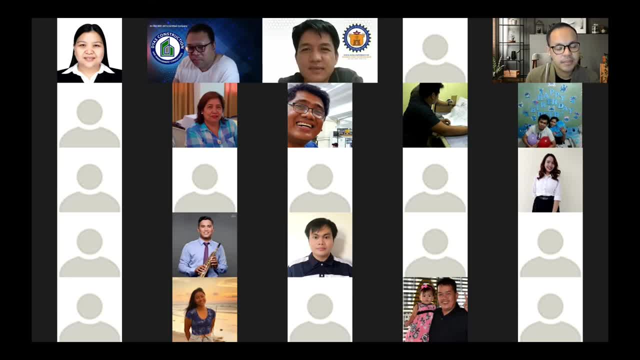 hindi sila pwedeng mag-claim in case may time extension Okay, Pero since nagkaroon niya ng pandemic, which is out of the argument nung ginagawa pa lang yung contract, nag-claim sila ngayon. 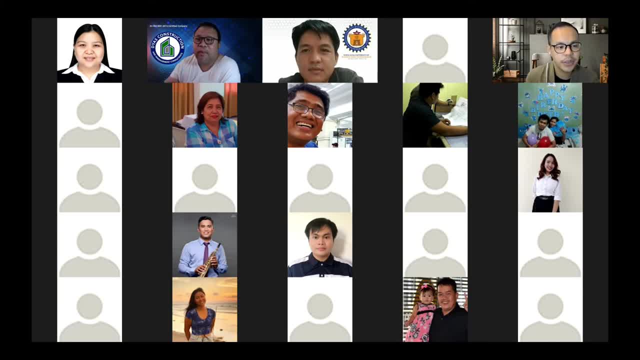 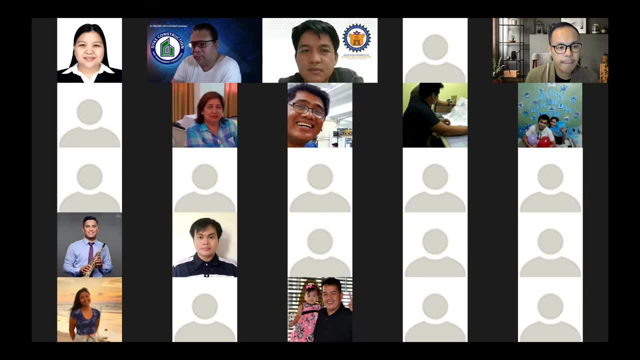 So yung contract na conclude or na-finalize, yung contract na during the pandemic, na Before po Around 2017? I think if may provision ka sa contract that says na hindi ka pwedeng mag-claim for extension of time. 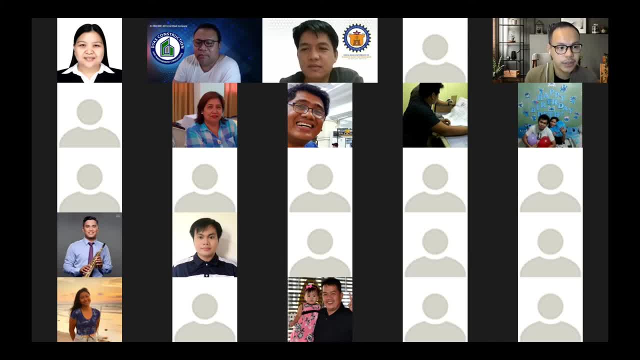 regardless kung ano na without any reasons or hindi naka-enumerate dun yung reasons, then unfortunately you cannot claim for extension of time. Pero maybe you can approach yung client mo and negotiate a settlement siguro. 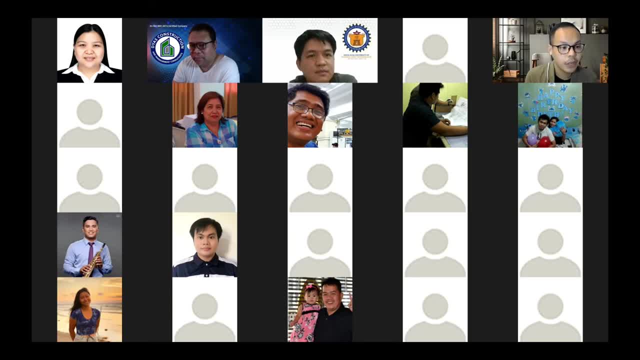 Na totoon doon naman kasi na meron kayong costs na incur. So maybe send fillers to the client na parang you want to claim and you're open for. So maybe send fillers to the client na parang you want to claim and you're open for. 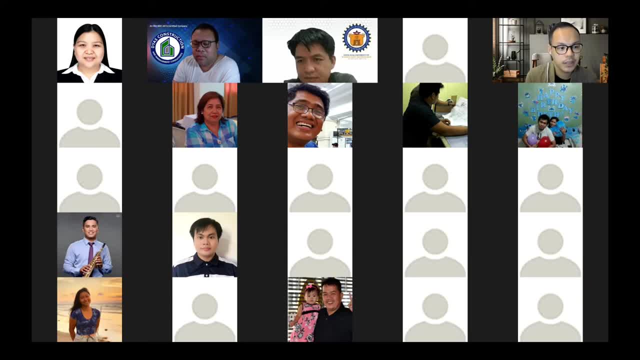 ah, negotiation of the additional fees. Okay, So ang ina-advise niyo po is for us to settle. Hindi ko ina-advise Ang opinion ko. Ang opinion ko is. ang opinion ko is Okay. 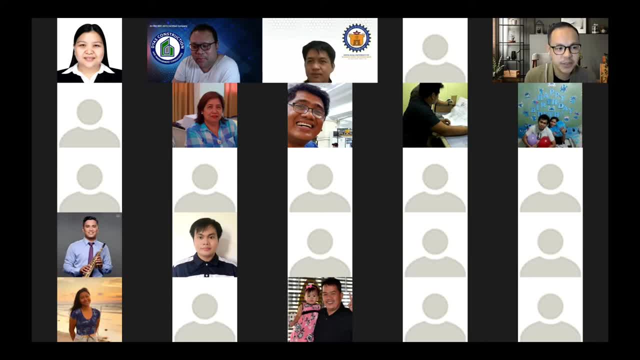 try a try a try a negotiation or hindi. ko ina-advise Okay, Kasi meron legal connotation yung advice which may expose me to liability na hindi covered ng aking professional indemnity insurance. So Sa case po kasi namin, kami yung client. 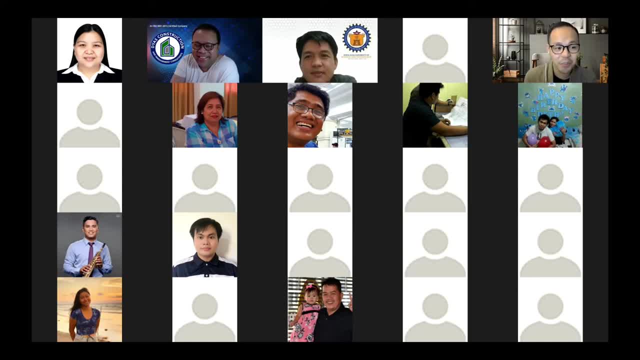 fit Oso kayo yung client. so are you even open for that? Then the next question is: are you open for that? I mean, are you willing to help your consultant Yun kung yung under Приvely abay niya? 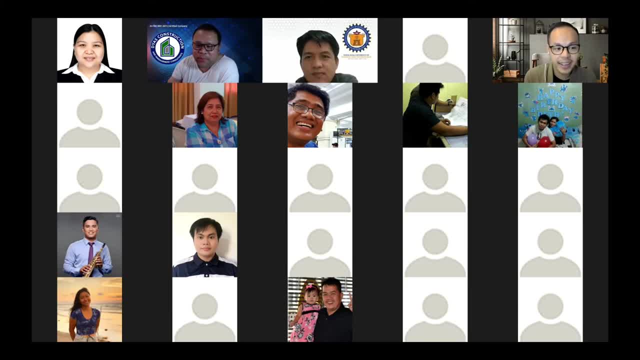 I work for a consultancy company and never pumasok sa isip namin na mag-claim kami for additional fees, because we don't have a right in the contract to claim for additional, Because the contract is lump-sum, Lump-sum, without any provision. 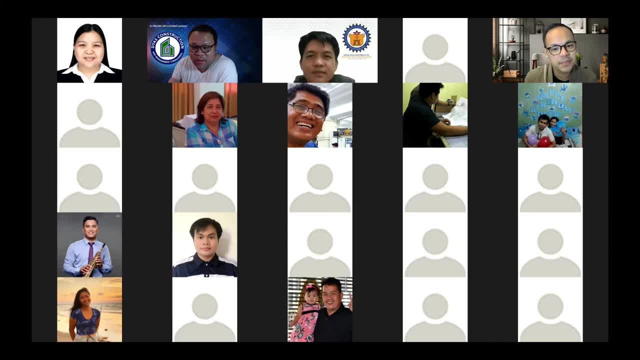 Hi Christine. Hi sir, We are a consultancy firm. We didn't request a time extension. Time extension is point, but more on the cost claims arising from the extension of time Is the monthly payment your consultant? The payment is based on the milestone of the construction contractor. 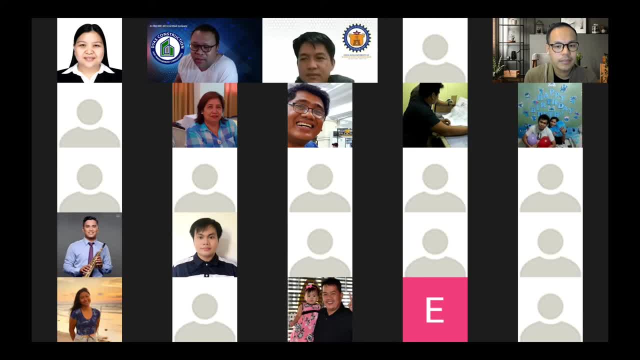 So he cannot claim because he didn't have POC at that time, right? No, he doesn't have POC at that time. Yes, But here the argument that would be- That's where I'm going to- If he didn't achieve the milestone, if your payment to the consultant is on a milestone basis, 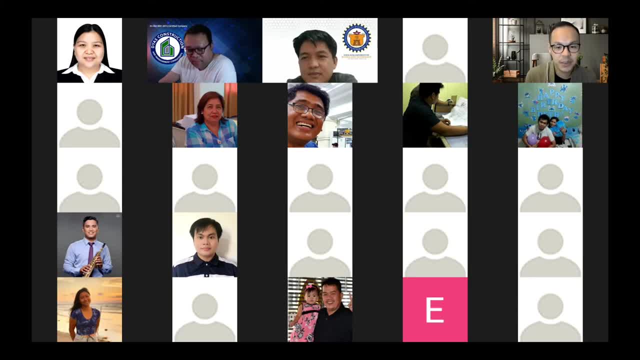 until the contractor doesn't achieve that milestone, then there is no entitlement for payment. So what if 10 years after he can't achieve that milestone? So I don't think you have a very good. The consultant has a very good. 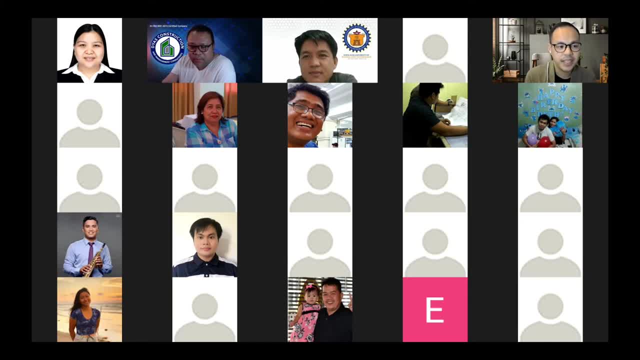 The consultant has a very good. The consultant has a very good legal foundation in terms of seeking for additional payment, especially if it's a milestone. That's why I asked if it's monthly or by milestone. It's risky because the consultant is already at risk. 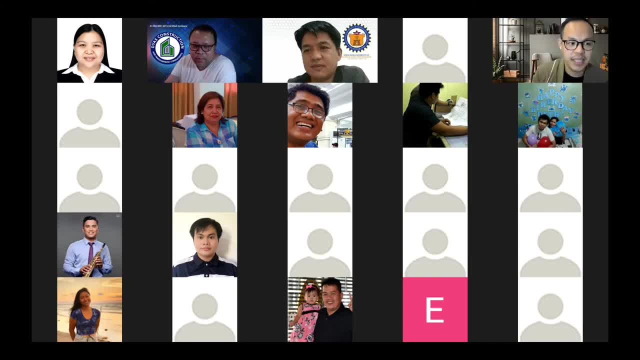 And they are very aware. The consultants are experts in construction And I'm sure that they've already mitigated that, or it's already included in their costs. It's just that maybe they're just asking for more. Another scenario is what if we issued a slowdown? 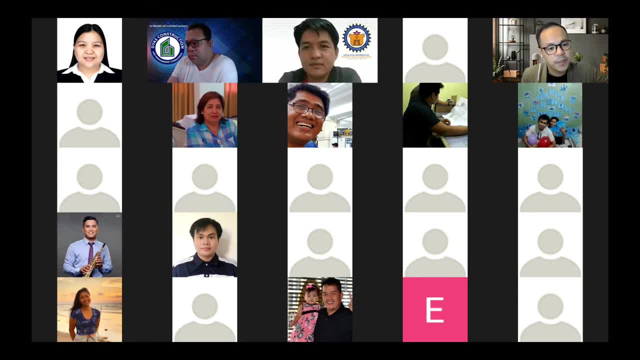 Because we also don't know the financial status of the project. What do you mean? What if we issued the slowdown, for example, from June to December, Because the lockdown was issued starting March up to May, And then, by June, we issued the slowdown? 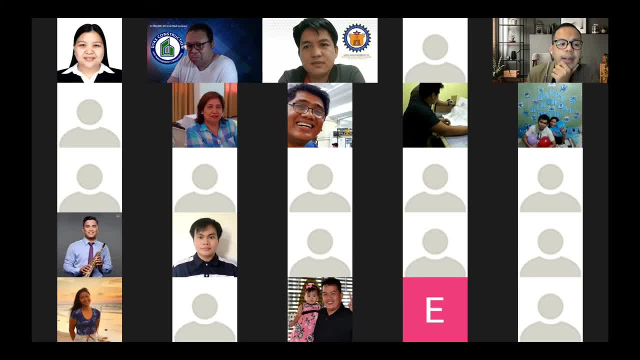 So a slowdown, meaning you imposed limitations On the design, On the design, On the design works, On the design works, For example, On the design works. Yeah, Because the contract is easy Again if the payment claims are also milestones. 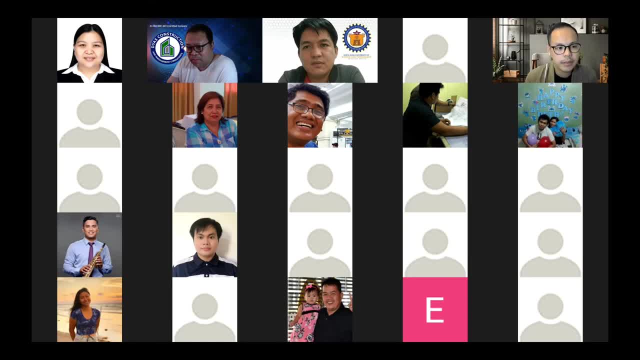 the entitlement for payment claim, then, Sorry, you haven't achieved the milestones yet, So there's no entitlement for payment yet. No, no, Wait, But that's a different case, because the proponent: Oh, it's a different case. 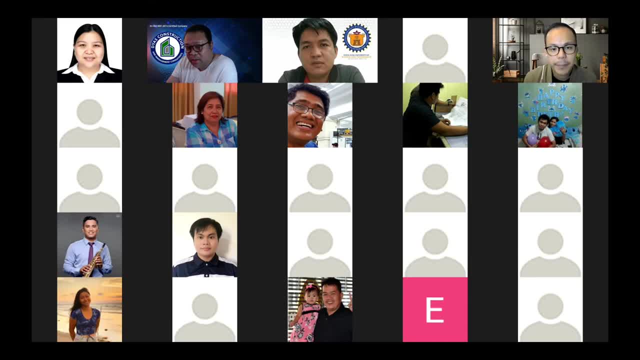 He said that there is a slowdown in the design phase. So the tendency is that the POC would be affected by the slowdown of the design phase. So that's a clear conflict between the contract. So there's- Oh, I get it now. 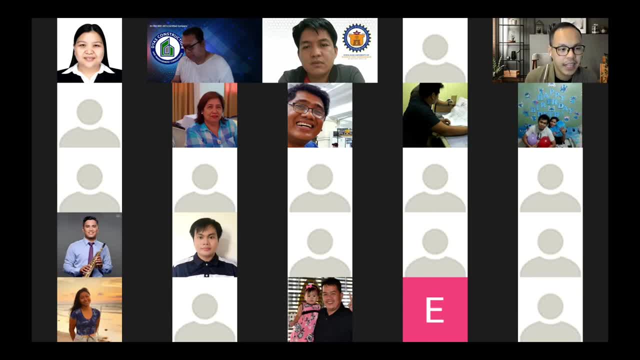 So there's Okay, I get it. But then again you have to check your contract. if you have a provision on that, If not, or if there's none absent any express provisions in the contract, then Yeah, Maybe you will be invited to the table for negotiation of revision of fees. 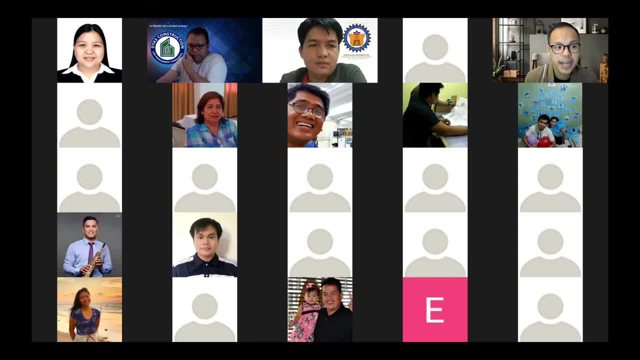 Check your contract. It's very important For the consultancy contracts. maybe it's only 10-15 pages. Thank you for answering your question. Sure, Sir, do you see another from Saray Munda? Okay, Another question, sir, related to possession of site. 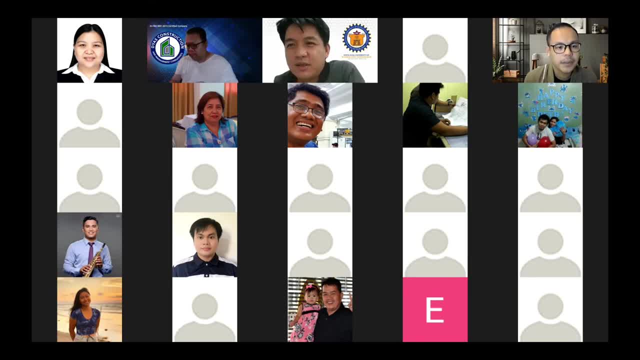 What is your opinion on public works projects where the employer is neither in possession of site but the contractor insists that the employer failed to give possession. Oh okay, So what is the risk of possession of site? Is it the risk of the employer or is it the risk of the contractor? 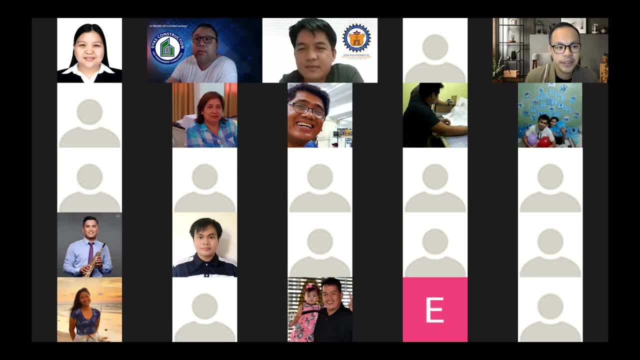 Because, without disclosing further details, I have encountered such a case. Their problem is the risk of clearing the site is under the contractor, So the site has many informal settlers, So they are still looking for ways to relocate the settlers and stuff like that. 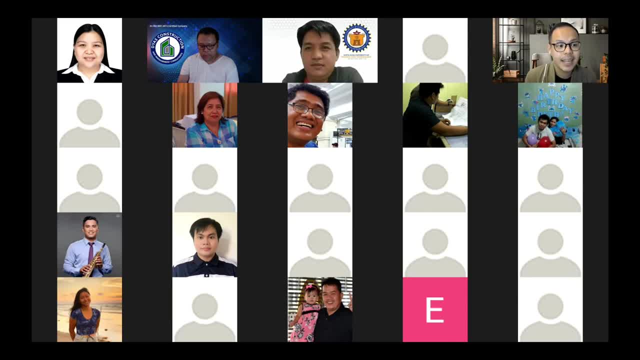 So it depends on whose risk it is. Is it the risk of the contractor or is it the risk of the employer? And then from there, that's where the determination of the entitlement or extension for failure to possess the site will start. Sir, what if the risk is not defined in the contract? 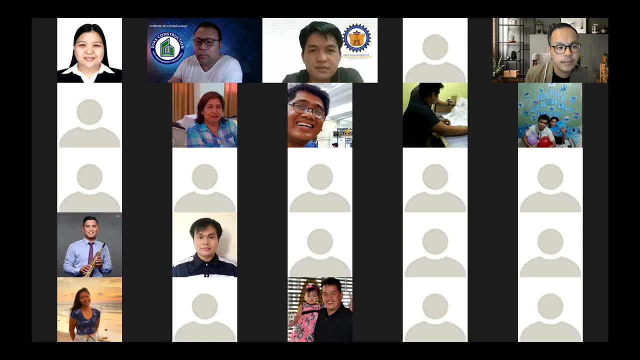 Meaning. this specific problem encountered is not defined in the contract as the employer's risk. neither is the contractor's risk. Hmm, Then you have to look at your costs. Do you have costs for the possession of site? If yes, if it includes site clearing or site preparation, stuff like that. 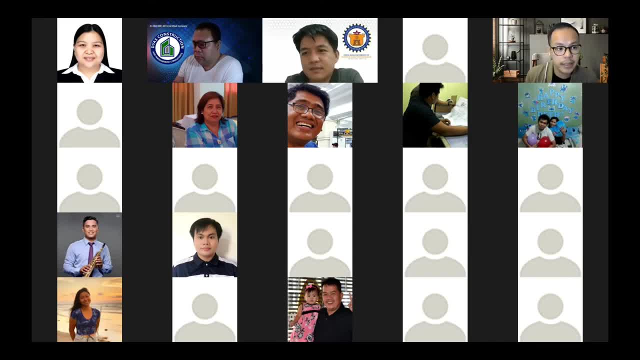 then it's under your. I would opine that would be under your risk. Hmm, Sometimes it's not expressly provided right, But look at your costs. Look at the whole contract as the whole contract. Then you interpret the different clauses, how they interact with each other, and then 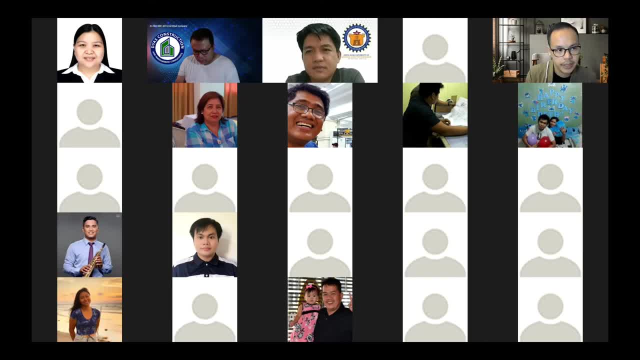 you will realize the risk of the contractor or the risk of the site clearance. Okay, Actually, sir. further to this problem, our interpretation as the employer of the contract is that the reason why we are requiring the contractor to secure the site clearance is: 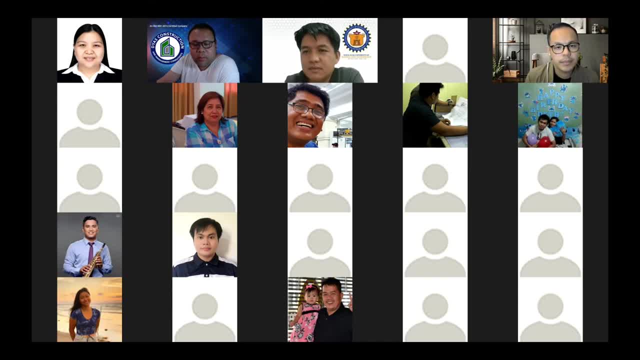 because we are requiring the contractor to secure first the permits from LGU before commencing the works, is taking possession of the site. So that is our argument with the contractor. However, the contractor insists that the employer and contractor relationship under the contract is not. 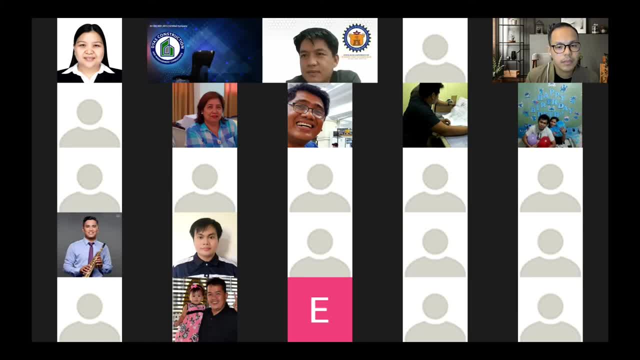 In other words, they are doing two sides of the coin. So meaning, sir, what he is saying is that, under the contract, the employer should provide the contractor possession of the site, Whereas for us, our opinion is that we do not own the site, which is why we are requiring. 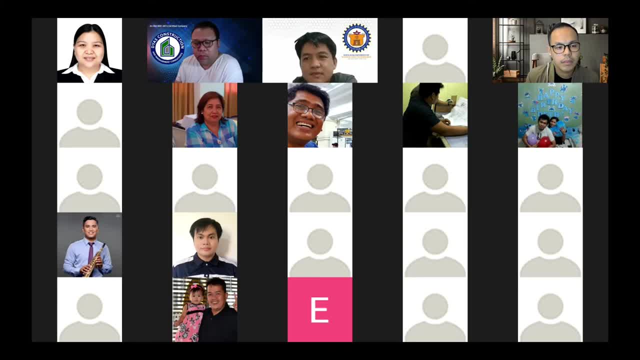 them to apply for permits. So what is your opinion on that? Again, opinion: Yes. So I think you can deduce the question. I think you can deduce your question into two parts. The first part: you said earlier the permits from the LGU is under the contractor's risk. 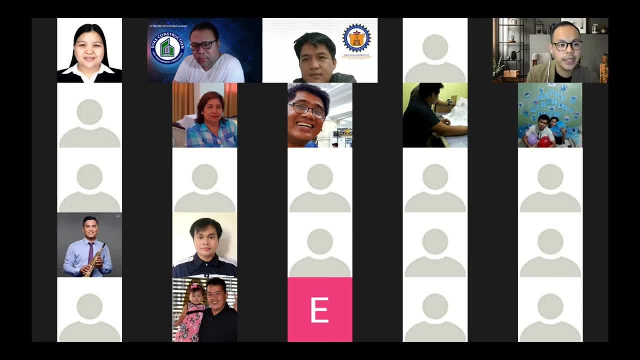 Yes, sir, And permit acquisition is a part or condition preceded to acquisition of the site. correct Or possession of the site. Yes, sir, That is what we are establishing, Yes, sir. So if you are able to establish that, then that will be a good starting point for you. 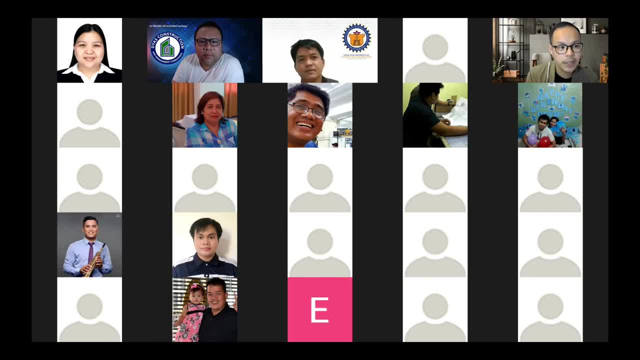 For you to pass the risk to the contractor Because you do not have. I mean, the site is there, you can start. It is just that you cannot start because you do not have a permit. Yes, sir, Who is in charge of the permit? 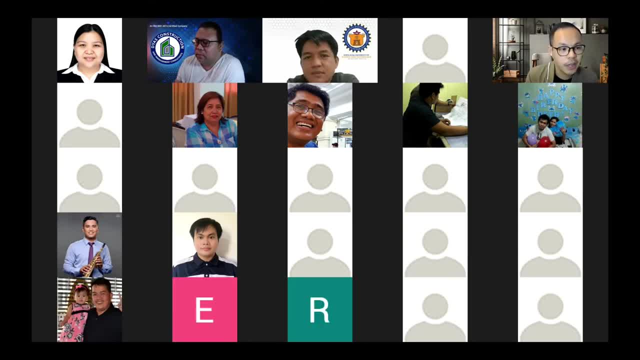 You the contractor. So, contractor, that will be your risk, if my interpretation of your contract is correct. So you look at your contract, Look at the- how do I say it? Tignan mo yung mga provisions, especially sa preambles. 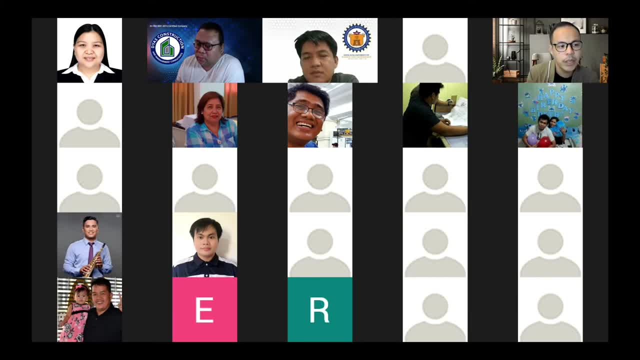 Usually nakasingit na sa preambles. If you have preambles to bills of quantities or sa specifications, May standard form of contract ba yan. Yung contract po namin ay based sa FIDIC, Pero hindi siya FIDIC. 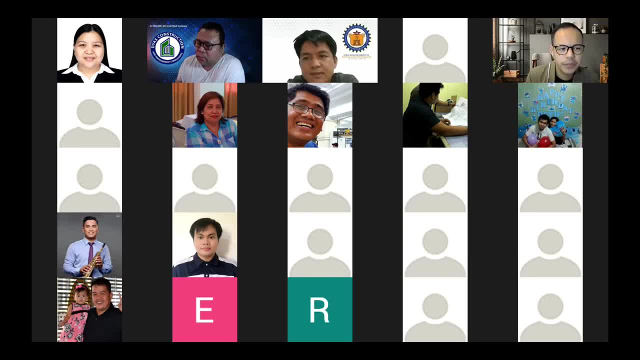 Not necessarily FIDIC. yes, sir, All right, So you just have to check. You just have to check your contract. Pero kung yung sinasabi mo condition preceded to the contract To the contractor commencing works on site is acquisition of permit from the LGU. 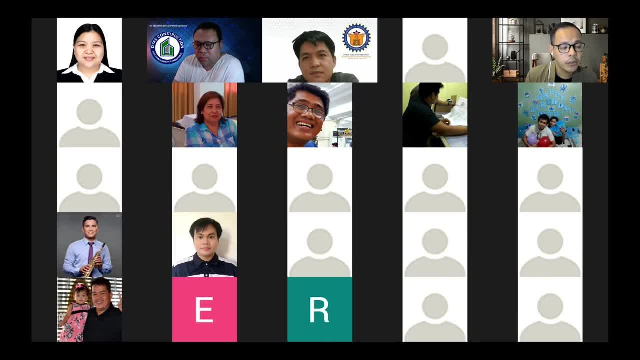 Then you have a good argument na risk nga ni contractor yung posesyon ng site Copy, sir. Thank you po All right. Okay, So another message, sir, So this is not actually a question. So from our dean Joseph Cruz. 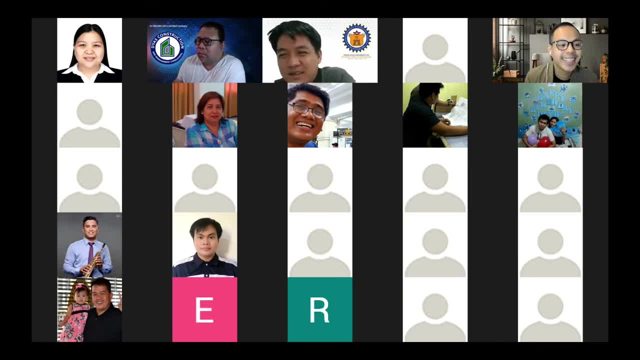 Congratulations. A very informative and productive seminar. So magaling si engineer Jose Carlo Padilla, Hindi siya selfish mag-share ng expertise. Thank you so much. So magaling po yan sa ating dean, sir JC. My pleasure, dean. 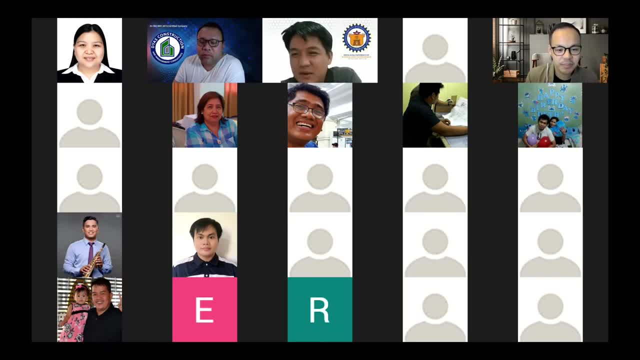 Then another question po Marami sa mga ongoing project during this pandemic may mga sariling protocol. One of these protocols is lockdown, ang mga workers sa site, In other words bawal lumabas. Then yung mga owner supplied materials na delay, so affected yung schedule ng contractor. 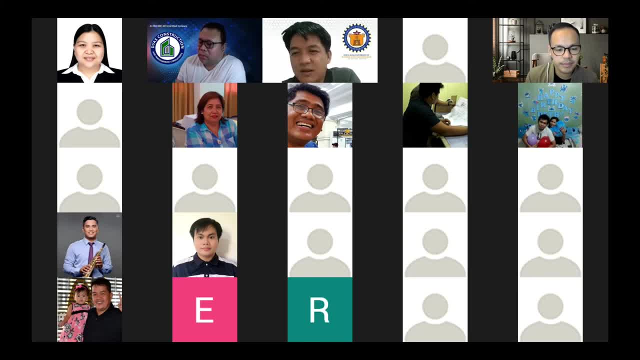 Tanong ko pwede bang mag-claim ng additional cost, si contractor, in terms of labor cost. Again, we'll go back to the reason: kung reason ng disruption or reason ng delay Is it because of the employer or is it because of a neutral event. 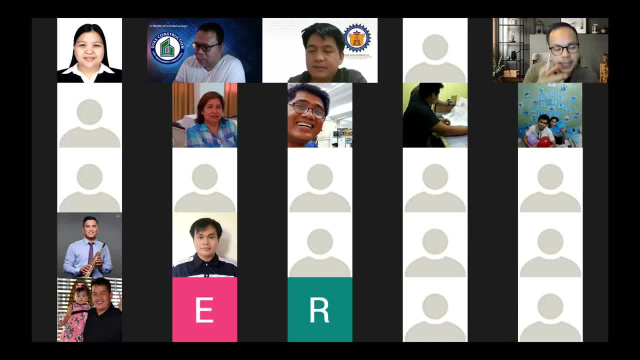 Yun yung ating base, Yun yung ating base, Yun yung ating starting point. Kung pandemic yan and may mga government orders, executive orders or government-issued instruments which has an effect of a law, then unfortunately walang ano. 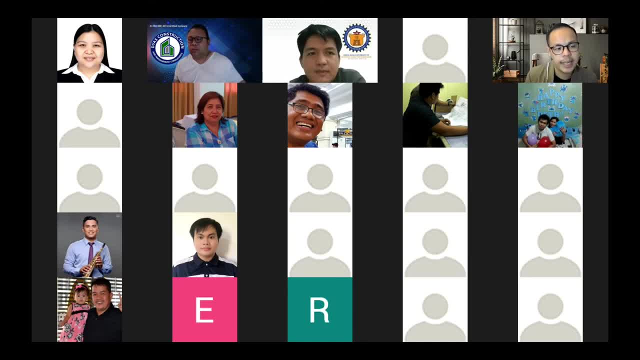 It's very difficult. It will be challenging to establish an entitlement, Pero they can try. They can still argue na they are entitled for the cost. They can still argue na they are entitled for the cost. They can still argue na they are entitled for the cost. 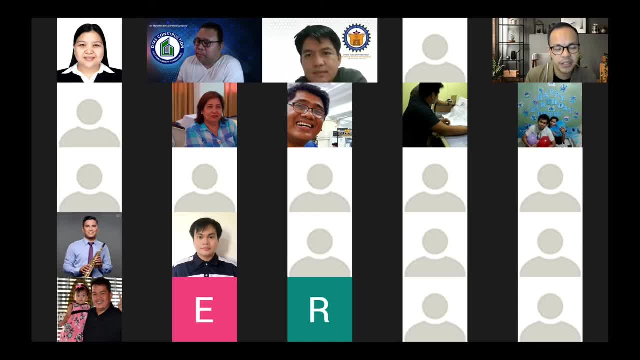 If I may just share Singapore, the government issued a legislation- cost sharing. So it's very clear. So it's very clear yung costs incurred by the contractor and the employer. So nakasulat doon ano yung pwede nila cost na i-share. 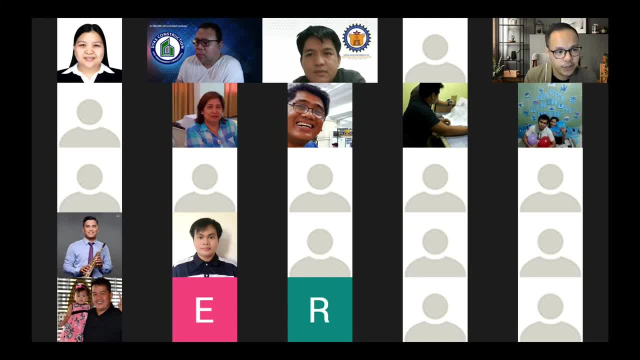 Ano, yung cost na kay contractor lang. So it's very clear. So maybe if we- I'm not sure whether yung Bayanihan Act covers this, Pero maybe you can check that one as well- Kung meron siyang cost sharing or a clause to that effect- 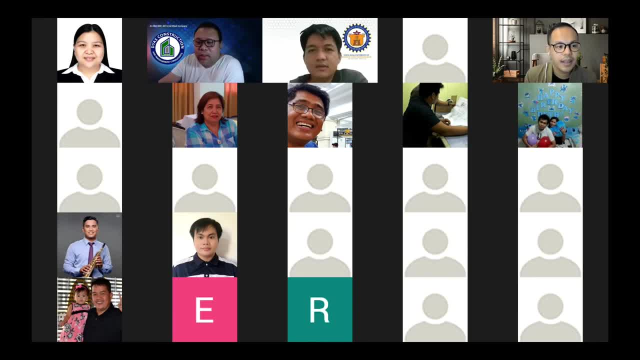 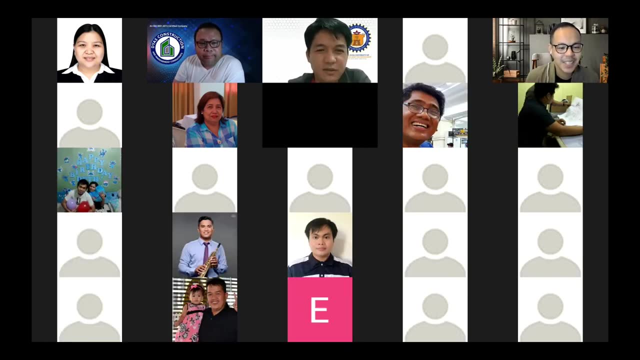 Okay, no more. Okay, kung wala na, siguro, sir, It's time na i-award na natin yung Okay. so, kung wala na pong questions and clarification, So it's time to award the certificate to our speaker. 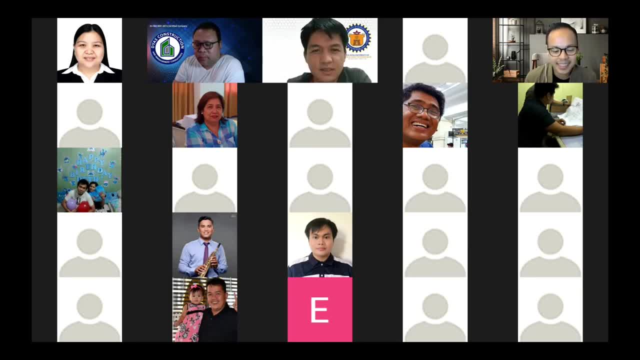 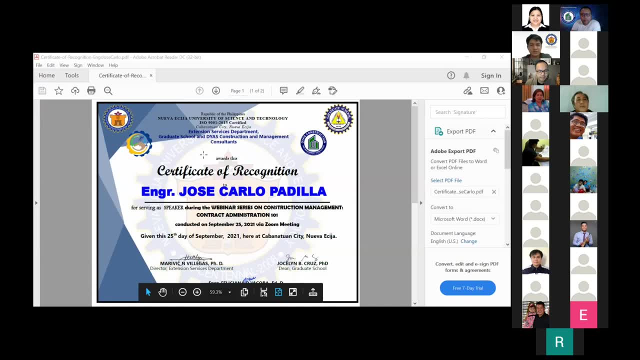 So let me share the screen, Okay. So participation. Republic of the Philippines, Nueva Ecija University of Science and Technology with ISO Certification 9001-2015,. Cabanatuan City, Nueva Ecija, Extension Services Department, Graduate School. 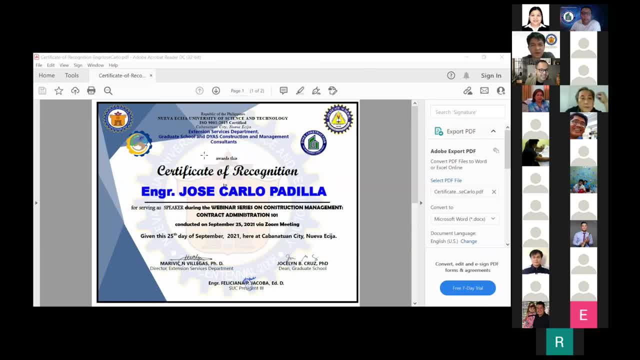 and Just Construction and Management Consultants Awards the Certificate of Recognition to Engineer Jose Carlo Padilla for serving as a speaker during the webinar series on construction management titled Contract Administration 101. Conducted on September 25, 2021 by Zoom meeting. Given this 25th day of September 2021 here at Cabanatuan City, Nueva Ecija. 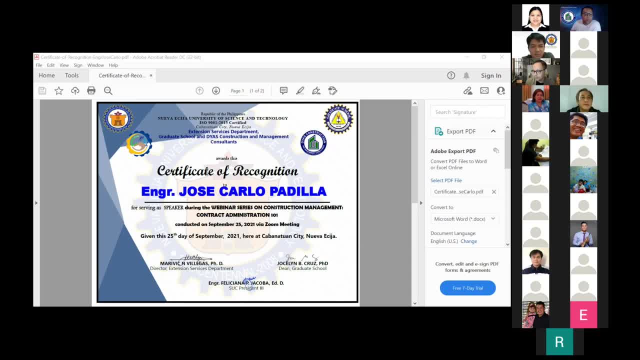 Signed: Marvic M Villegas, PhD Director Extension Services Department. Jocelyn B Cruz, PhD Dean Graduate School. Then Engineer Feliciano P Jacoba, EdD. SA President III. 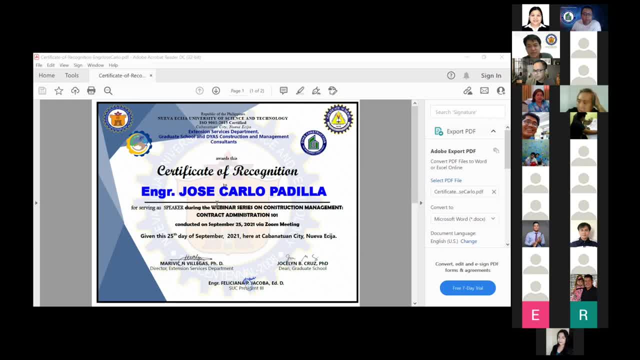 So, once again, Sir JC, thank you very much and congratulations, Thank you, Thank you. Thank you, NEUST Graduate School. Thank you, Jophel and Chet, for this opportunity you've given me today, So it was very productive. 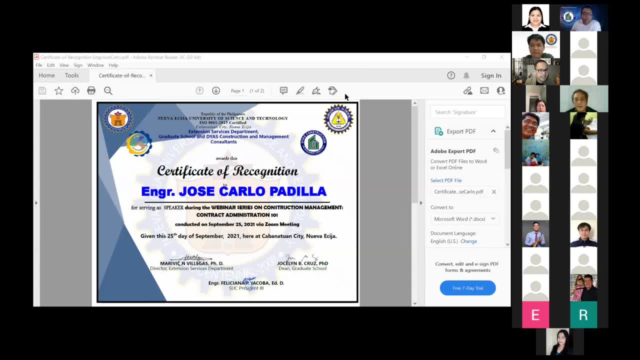 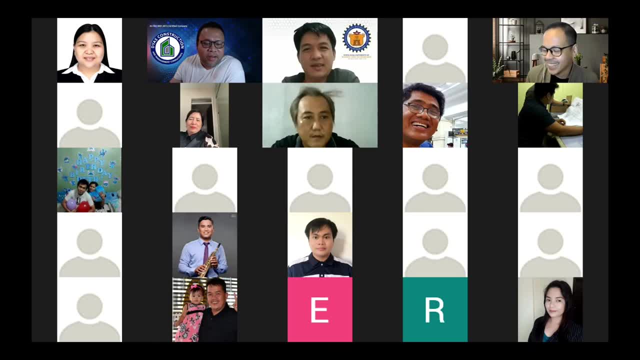 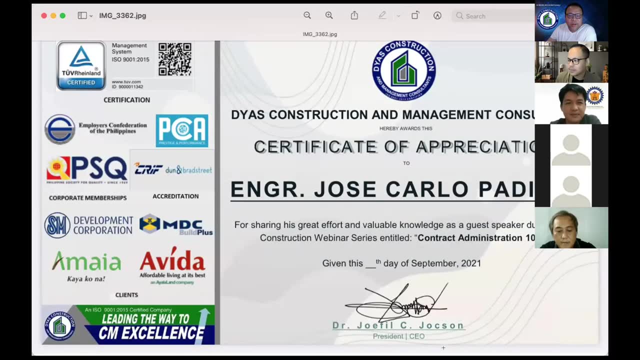 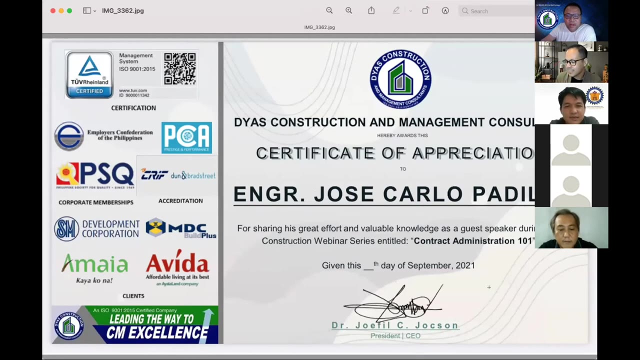 And this is a very lively conversation. Okay, All right. On behalf of the month's adjuster, I suggest the month. Okay, So here Certificate of Appreciation is also given. Just Construction and Management Consultants. An ISO 9001-2015 Certified Company in Construction Management.